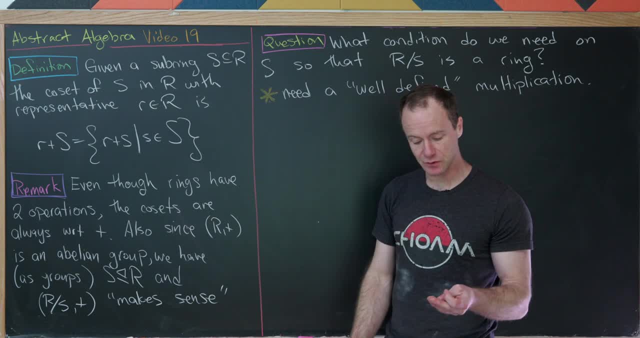 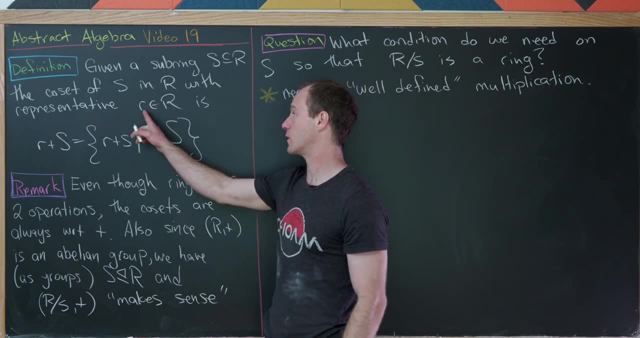 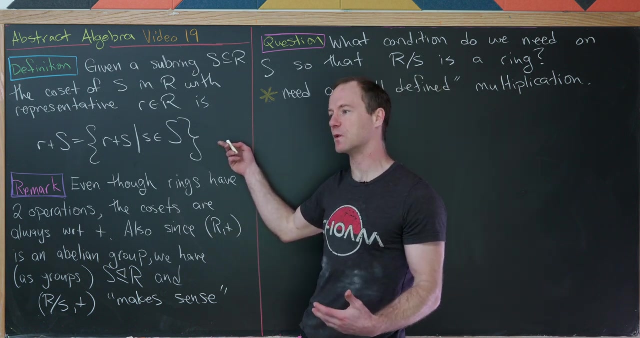 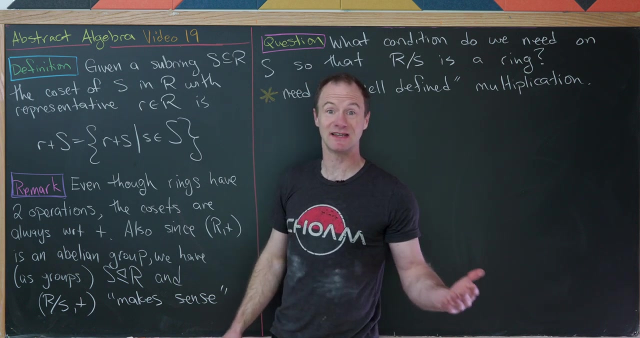 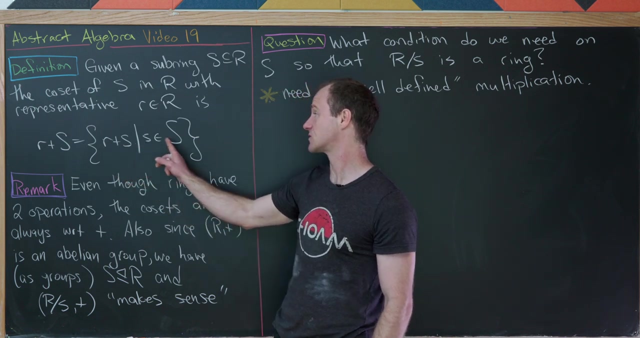 and we'll start with the following definition. So given a subring S of a ring R, the coset of S in R with representative little r is defined to be the following object, which should look familiar from when we were dealing with cosets of groups. So we have little r plus S. So that's going to be a set made up of the form everything little r plus S, as this little s ranges through the entire 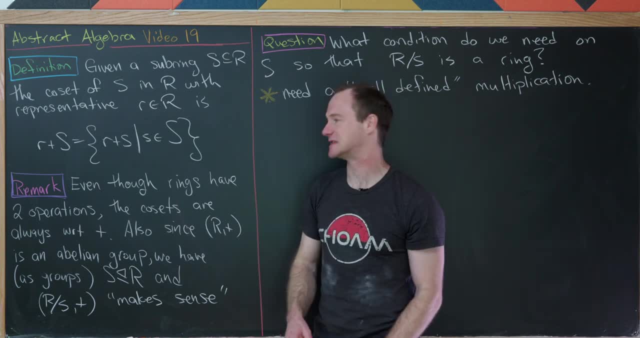 subring S. So we'll of course look at examples of this, but that's this definition of a coset. 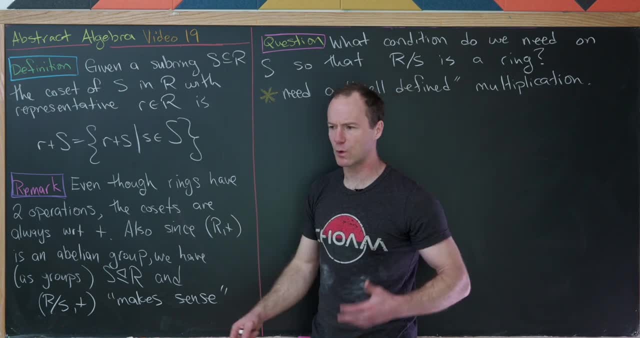 Now I'd like to make a couple of quick remarks before we move on to forging this into a set of cosets. Now I'd like to make a couple of quick remarks before we move on to forging this into a coset. 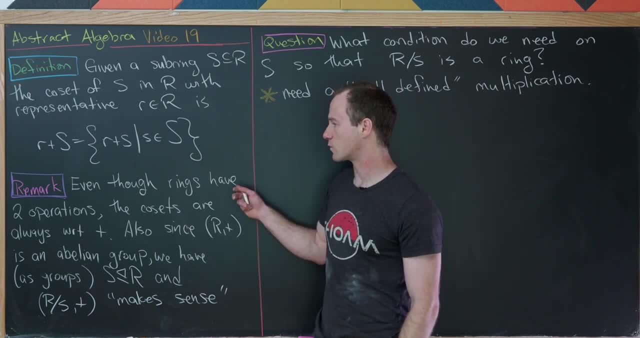 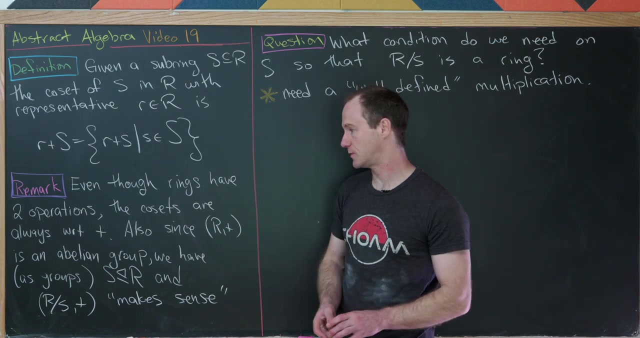 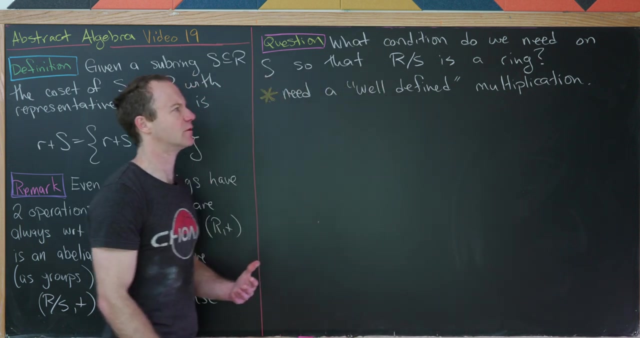 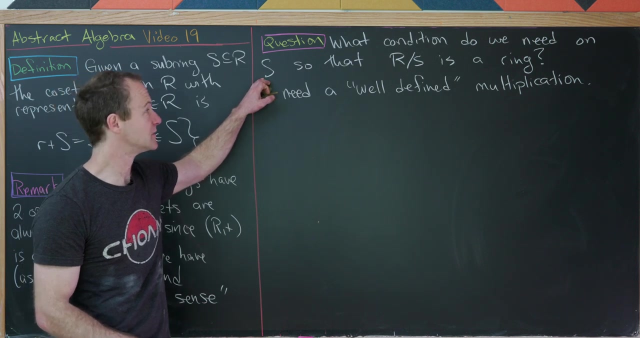 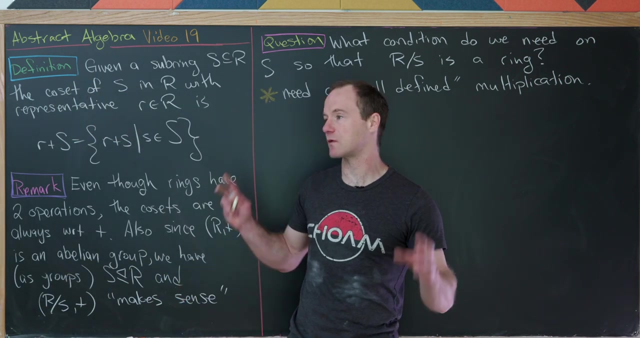 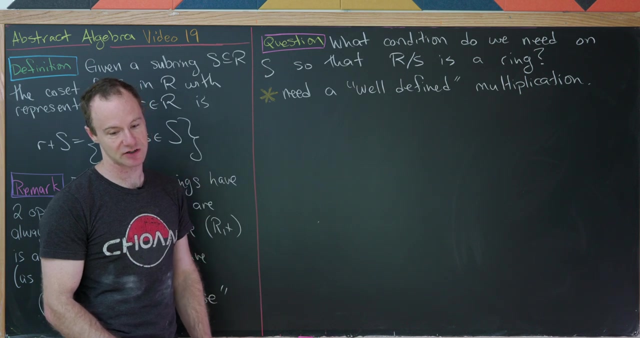 to something called an ideal. So even though rings have two operations, addition and multiplication, the cosets are always with respect to addition. And then also, since R with addition is an abelian group, then if we view everything as a group, S is a normal subgroup of R. And that's because any subgroup in the setting of an abelian group is a normal subgroup. But if you've got a normal subgroup, then immediately R mod S makes sense. The quotient group R mod S makes sense, where the operation is addition. And that leads us to the following really important question is, what condition do we need on S, the subring, so that R mod S is a ring itself? So like we noted over here, addition is already okay. So that means all we need is to make sure we have a well-defined multiplication. 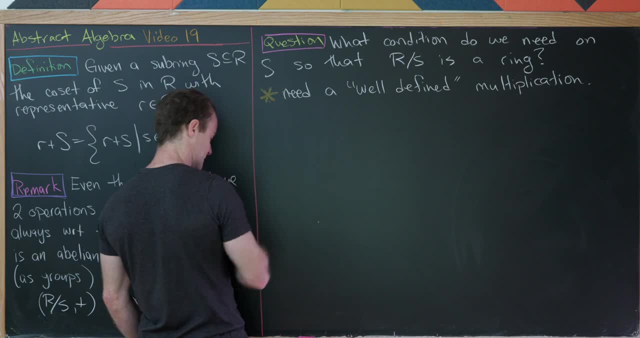 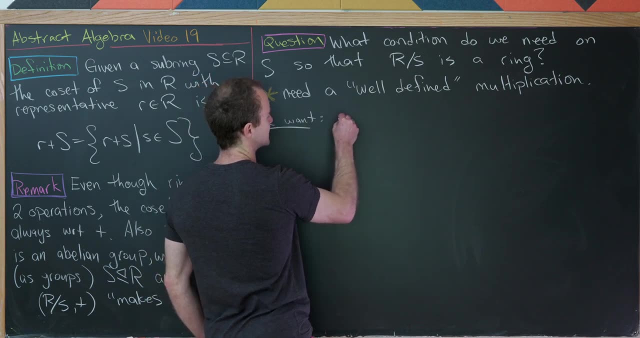 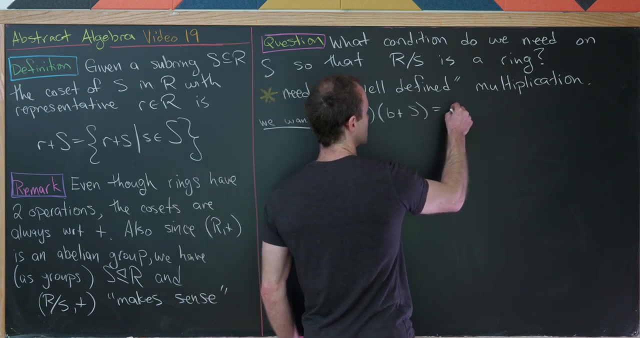 So we would probably like to define the multiplication like this. So maybe we'll write that as we want to define a multiplication so that A plus S times B plus S equals A times B plus S. So that would be the 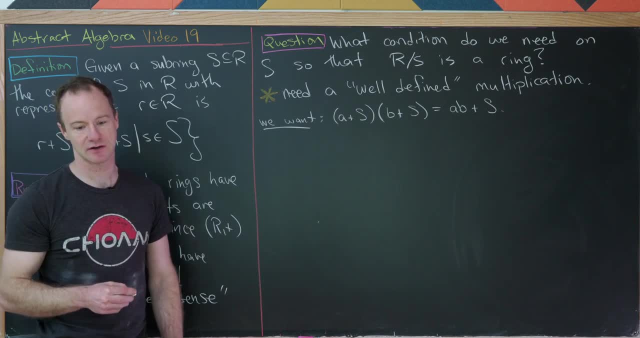 easiest way to define a multiplication. But like I said before, we need this to be well-defined. 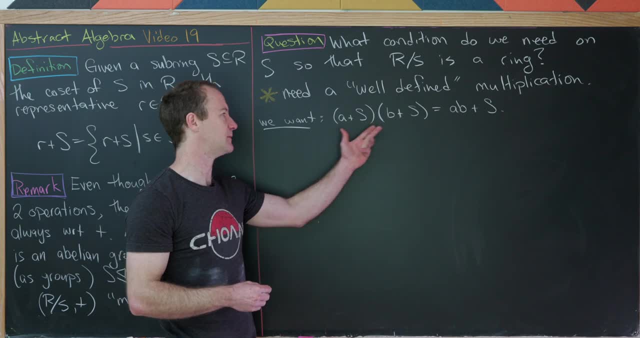 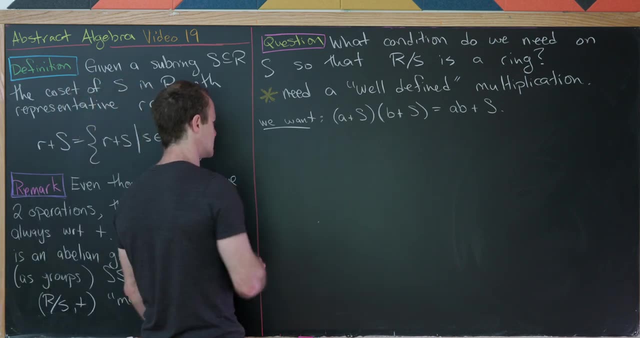 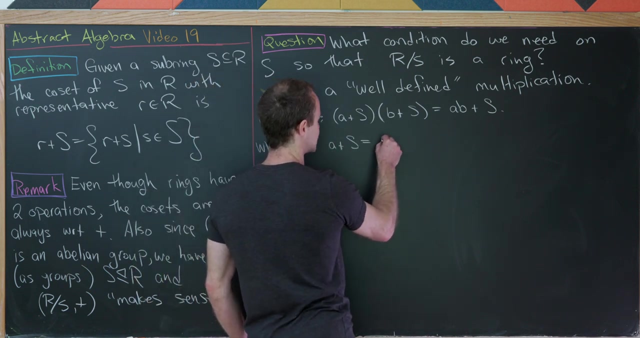 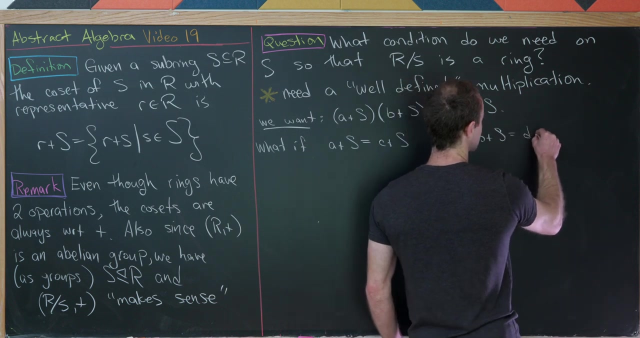 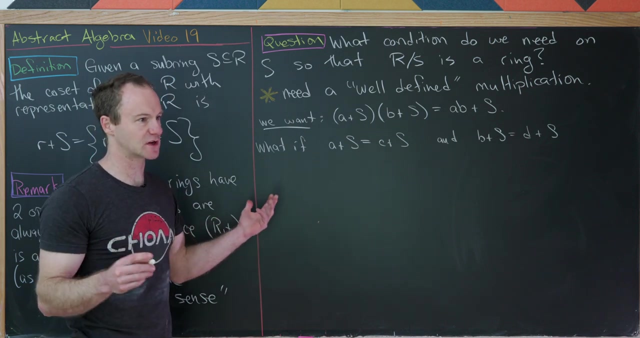 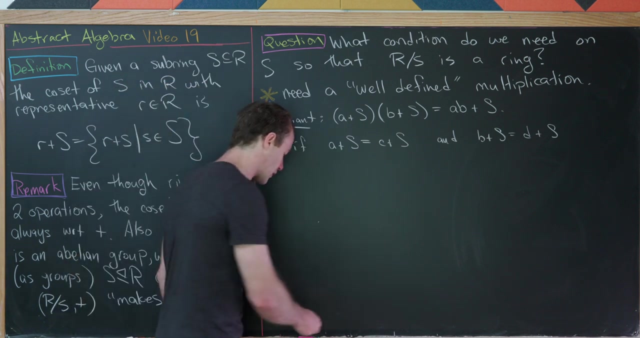 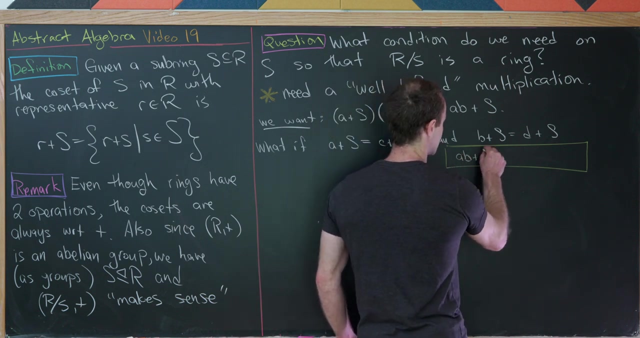 And by that, we need this not to depend on the coset representative. Okay, so let's see exactly what that means. So what if we have equality of cosets? So A plus S is the same thing as C plus S. And B plus S is the same thing as D plus S. Then it shouldn't matter which version of the cosets we multiply together in order to give us the same answer. Okay, so in other words, what we want to get out of this is A B plus S must be equal to C D plus S. But let's recall 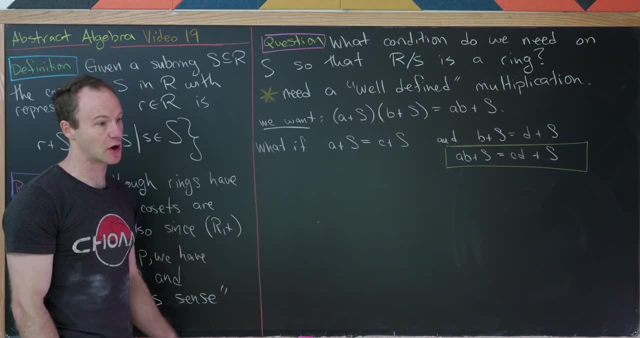 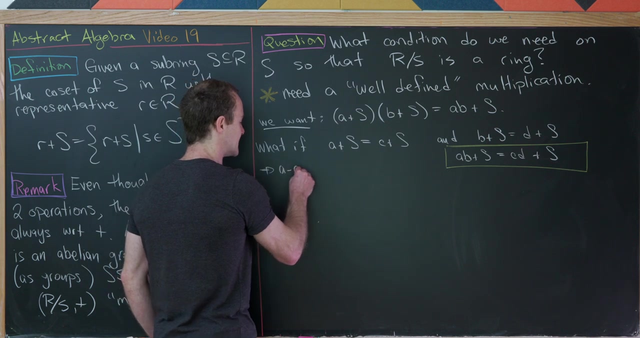 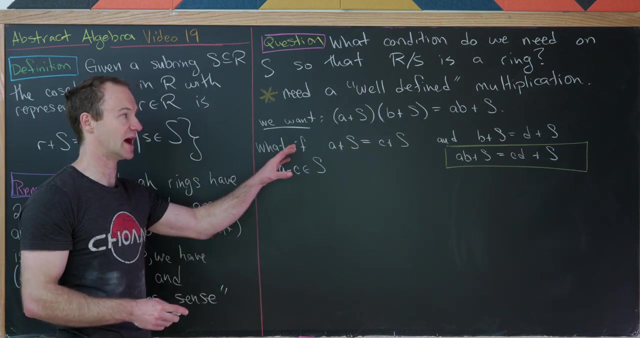 that we've got a lot of results about equality of cosets for groups. And we can use those here where our group operation is addition. So let's notice that this right here will tell us that A minus C is an element of S. That's from that big result on coset equality just applied here to the additive group, you know, R. Okay. 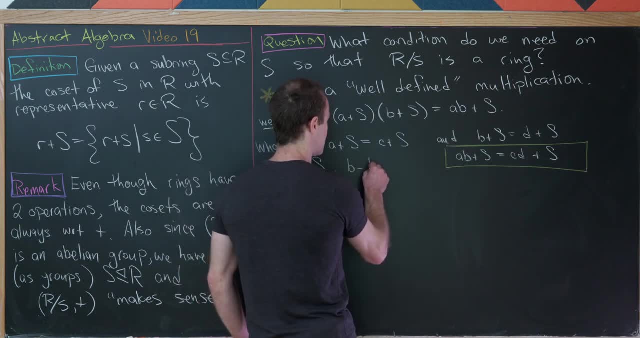 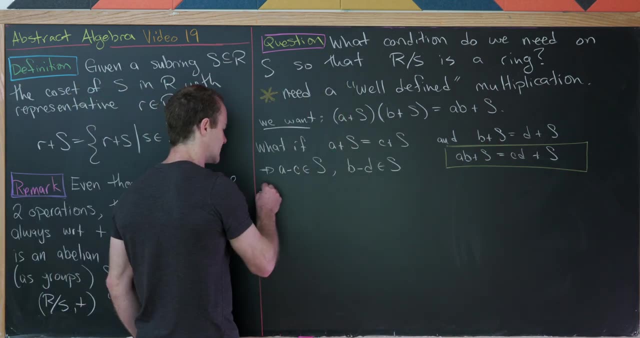 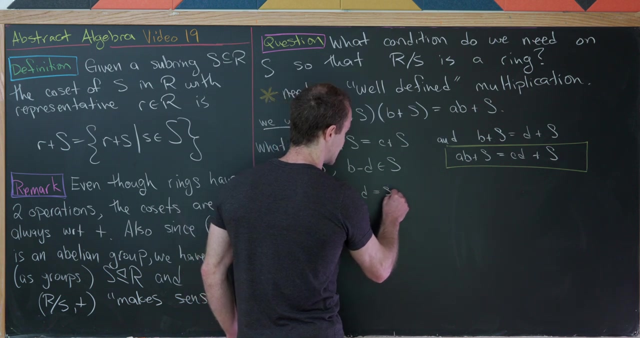 And then similarly, we'll have B minus D is an element of S from this right here. Okay, but then that tells us that A minus C equals S1, and B minus D equals S2, where S1 and S2 are elements of S. 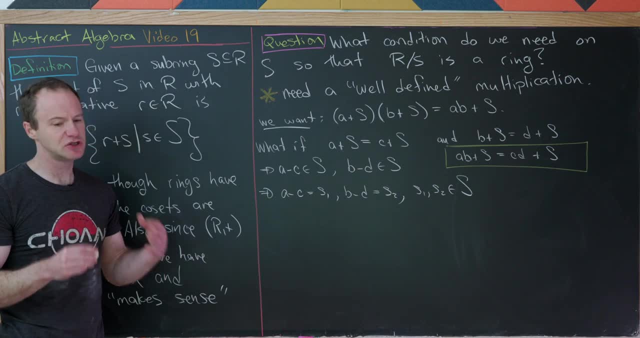 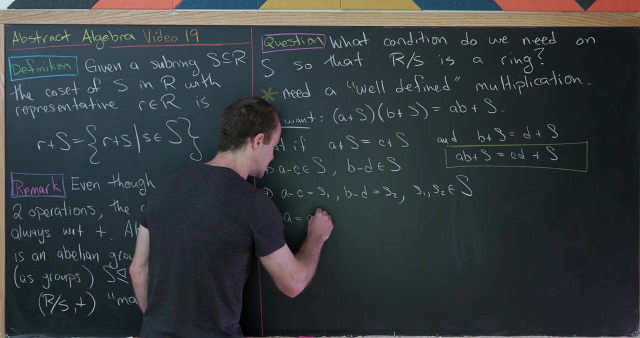 So it'll be helpful to do this so that we can maybe do everything at the level of elements. which is maybe less efficient, but more illuminating when we're getting used to this setting. Okay, but now let's rewrite this a little bit. This means that A is equal to C plus S1, 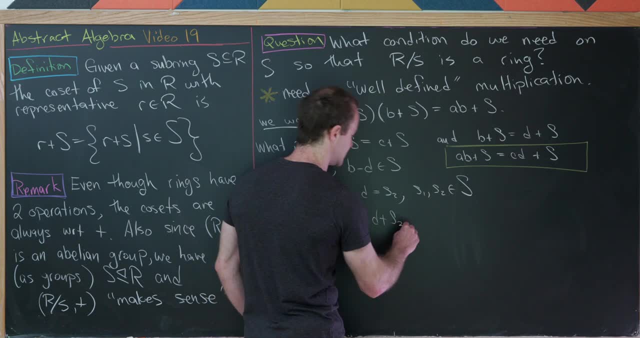 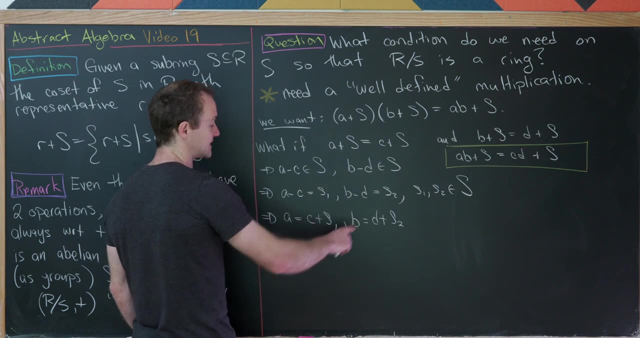 and then B is equal to D plus S2. And now let's take the product of A times B, and the product of C plus S1 and D plus S2. Well, those are the same products. So let's maybe put this as like an observation. Let's notice that in fact, A plus B is equal to 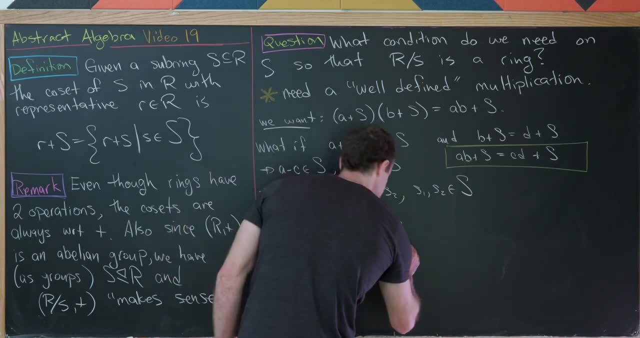 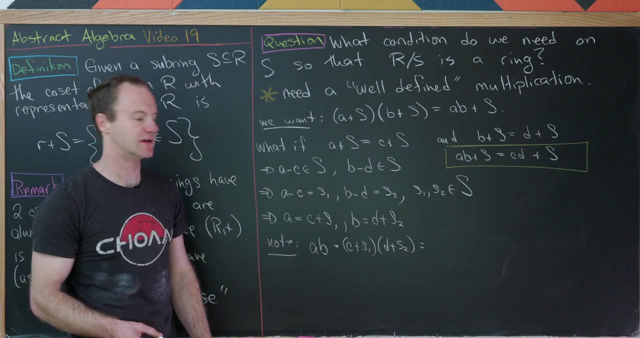 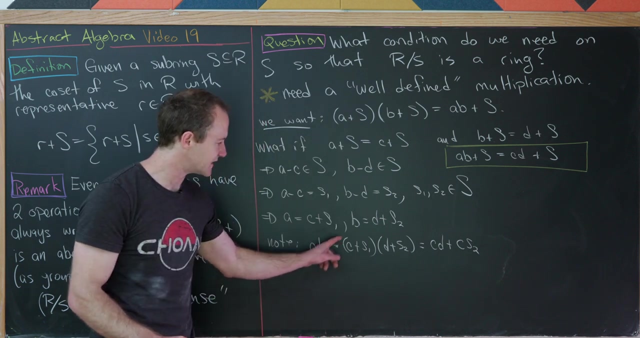 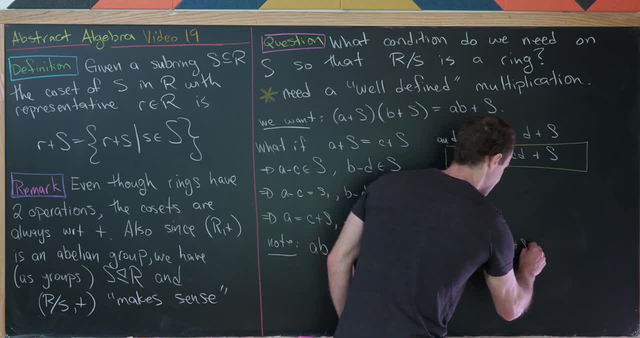 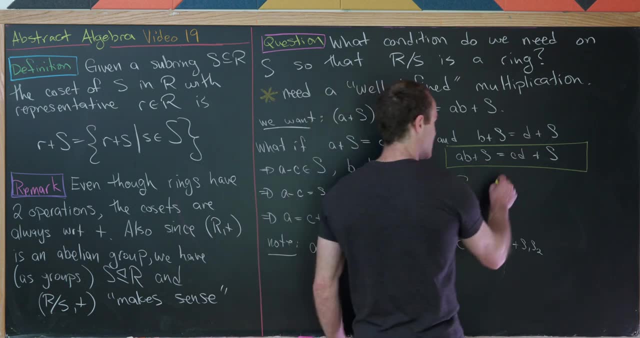 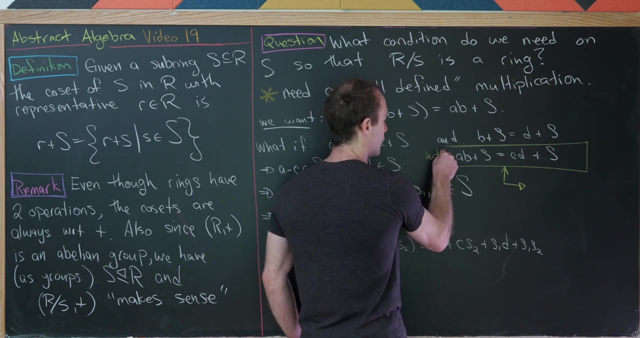 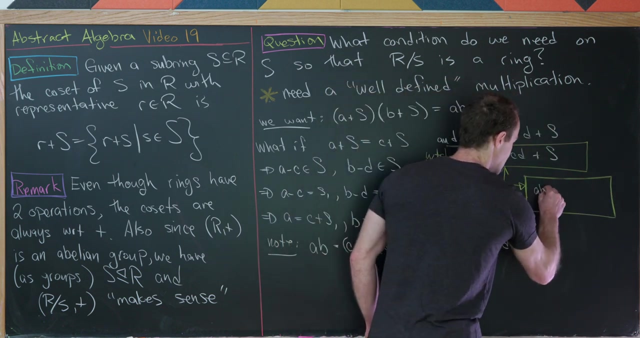 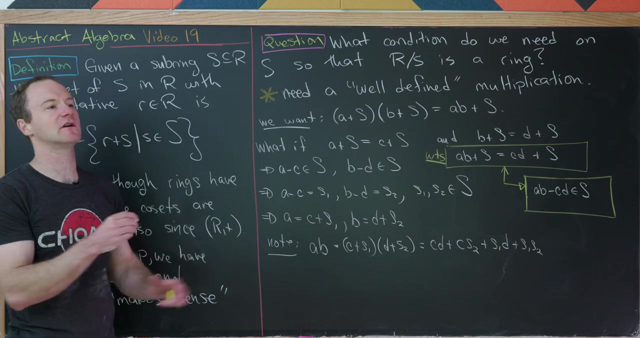 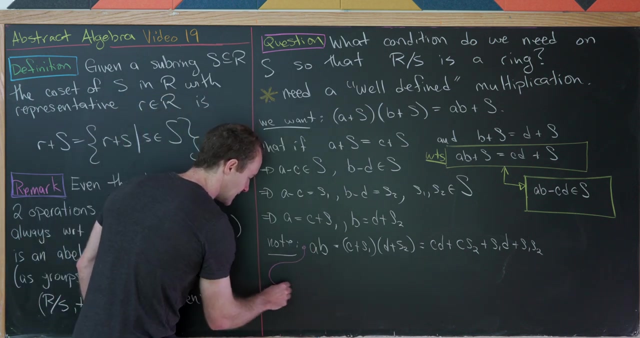 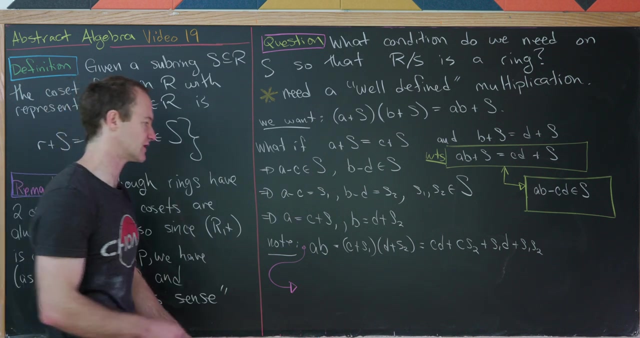 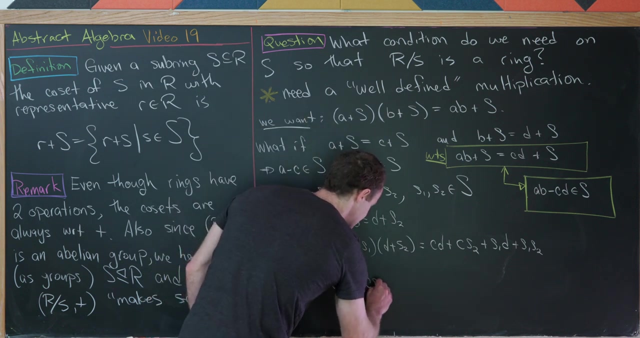 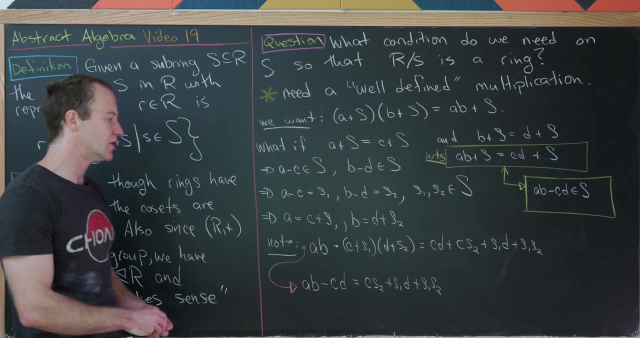 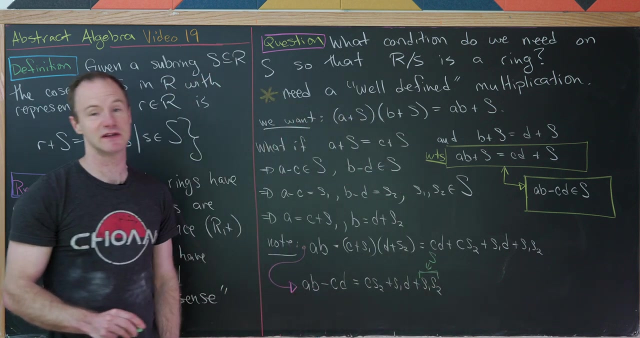 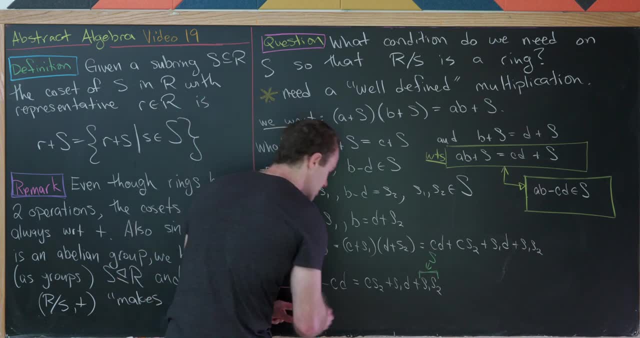 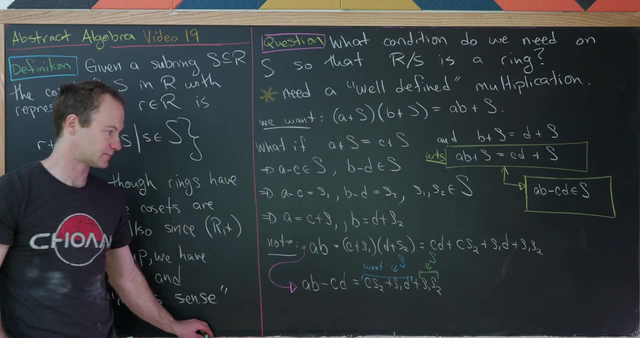 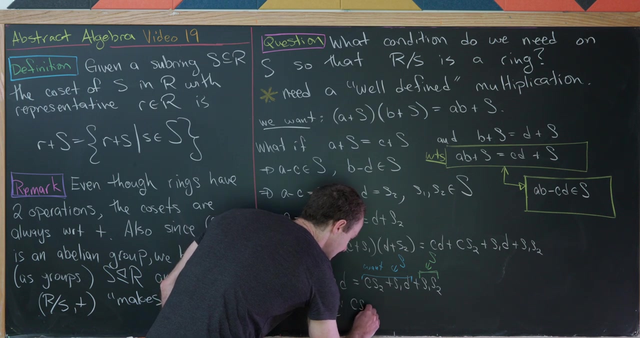 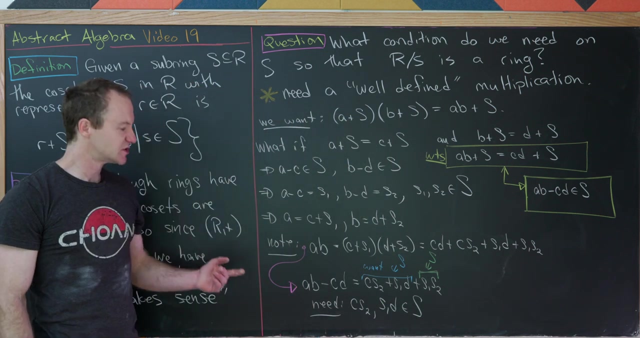 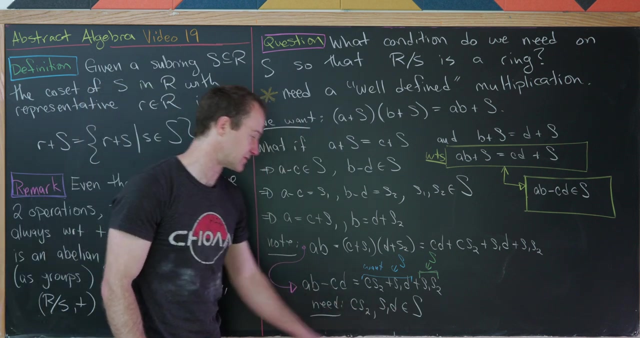 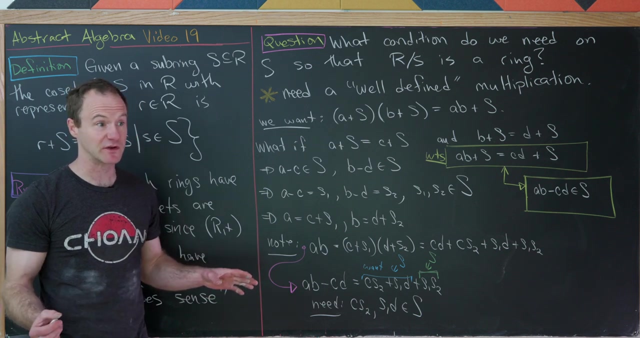 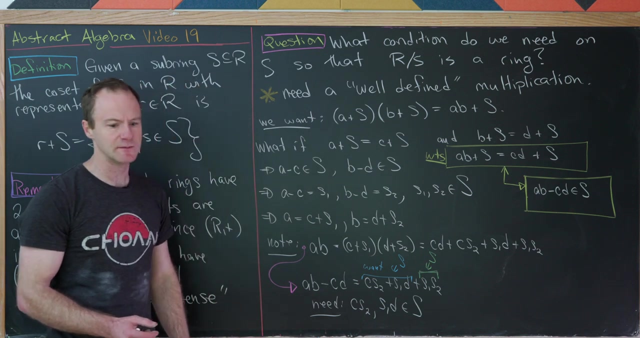 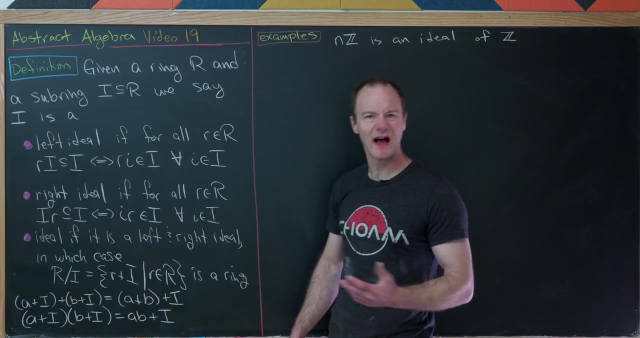 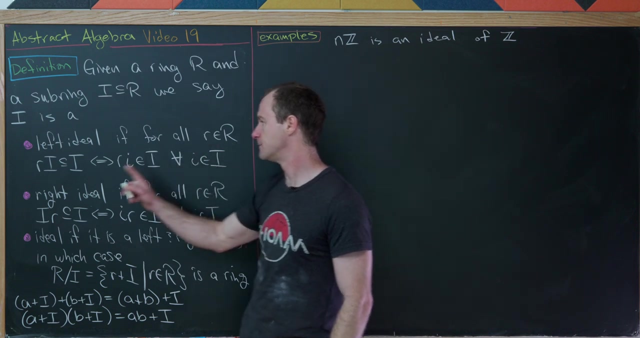 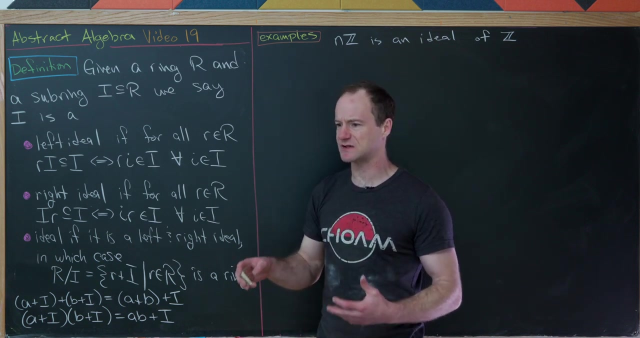 So let's maybe do this in a slightly different color. So we want these two to be elements of S. Okay. So that means that what we really need to occur is for C times S2 and S1 times D to be elements of S. So in other words, if we right multiply something by an element of S and left multiply something by an element of S, we should end up in S. And that's in fact the condition that we will need in order for this quotient to be a ring. And that condition will be called being an ideal. Okay. So now that we've motivated this condition, let's write that definition on the board over here and then explore some examples. So summarizing that condition we got on the last board leads us to the following definition. So given a ring R and a subring, we wanna write it as a subset of I. We say that I is a left ideal if for all r in R, little r times I is a subset of I. But that's like the way of writing it as a subset condition. 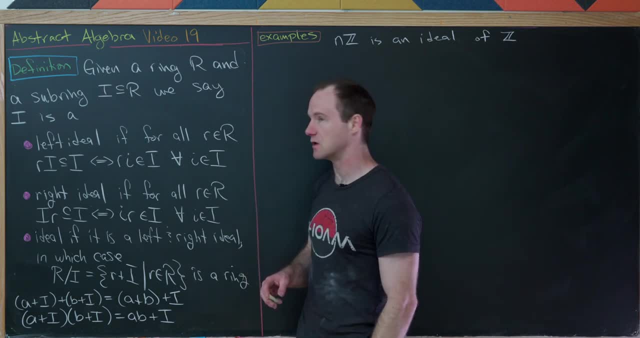 But usually it's a little bit easier to write it or little bit easier to come to grips with it when 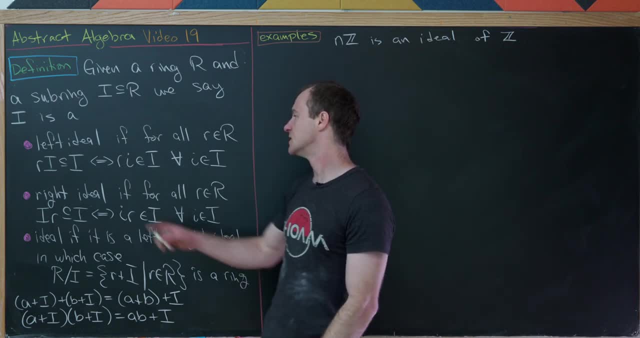 you're learning this stuff with an element condition. So that's equivalent to saying that little r times little i is an element of I. for all I in capital I. And then we've got another definition for a right ideal. And that says that 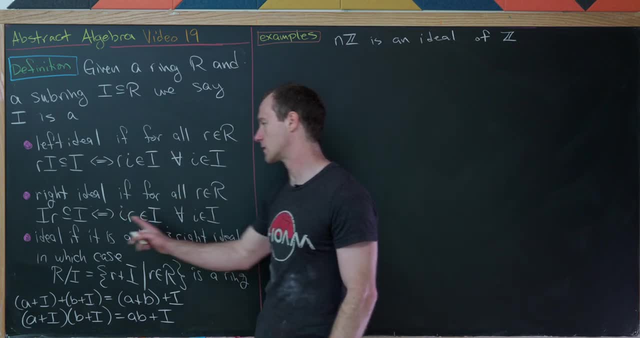 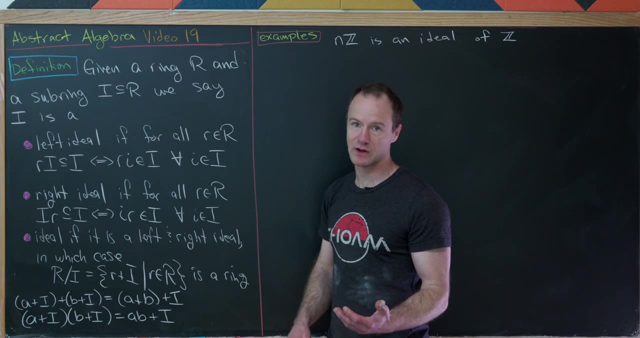 this is a right ideal if for all little r in R, I little r is a subset of I. But again, if we want to write that in an element-wise setup, we would have I little i times R is an element of I for all I in I. And then we say it's an ideal or sometimes a two-sided ideal if it's both a 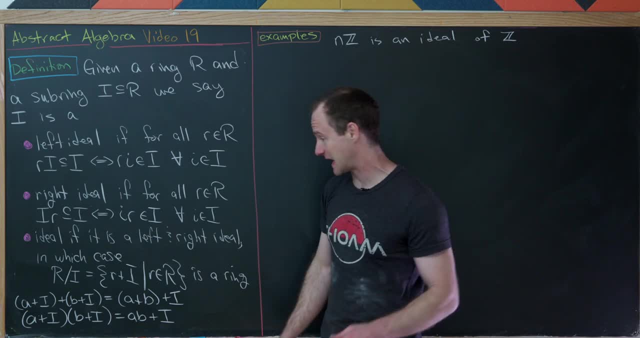 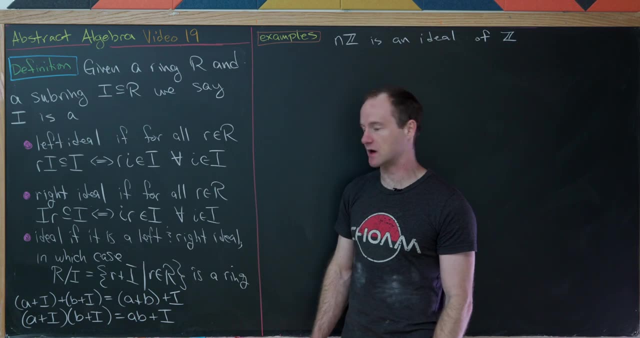 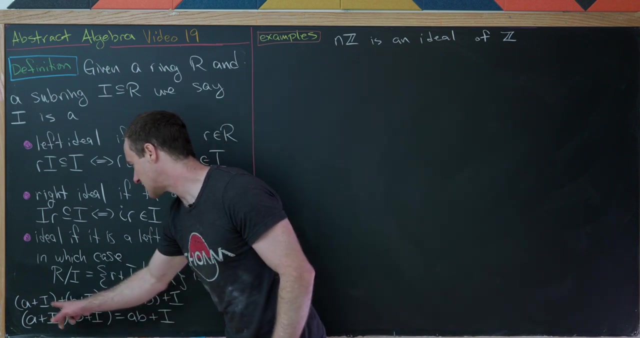 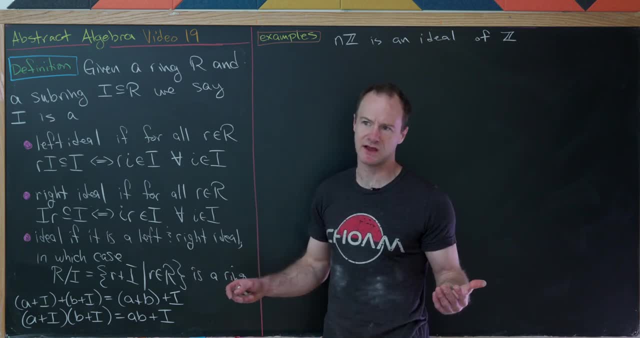 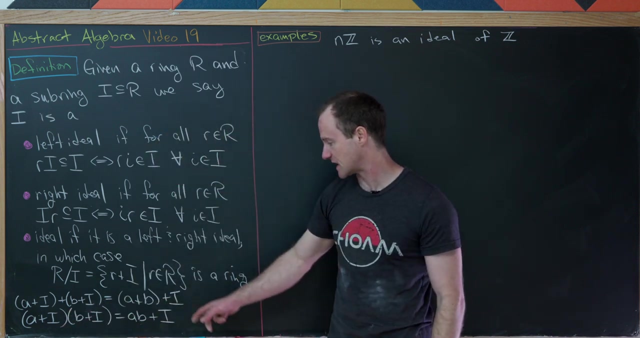 that's at the level of billion groups, so that shouldn't be like any problem at all. And then this structure of the ideal means that the multiplication is well defined as we discussed earlier, and so that we have A plus I times B plus I is A times B plus 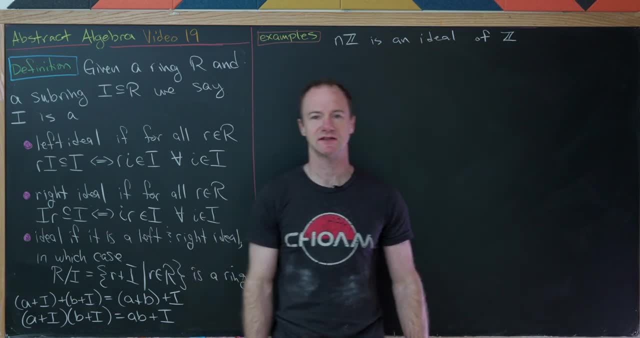 I. So coset multiplication makes sense in this case. 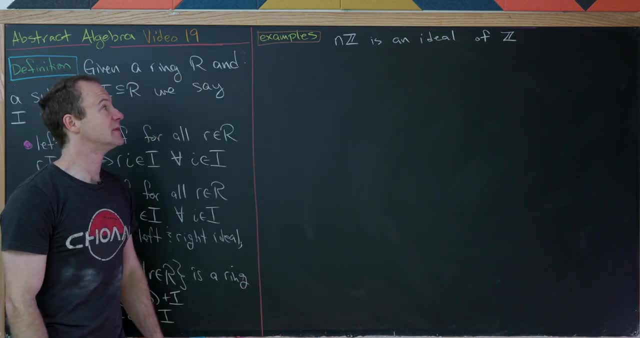 So now let's look at some examples, starting with a very basic one. NZ is an ideal of Z. Okay, so we can check this really easily. So this is a subring. That's pretty easy to check. I won't do that. 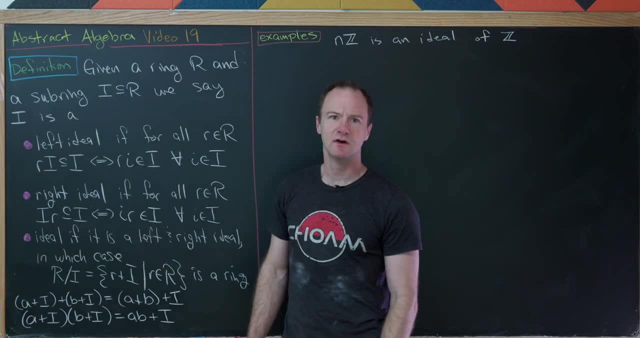 Let's check that it has these ideal properties. Since this is commutative, we only have to check one of them because there are no left and right ideals inside of commutative rings. There are only two-sided ideals. Okay. 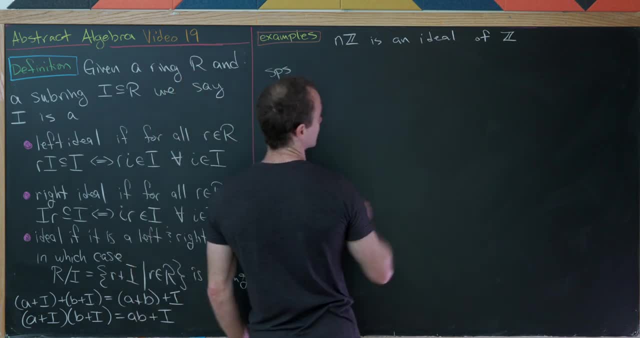 So let's suppose that we've got some sort of arbitrary element of Z. 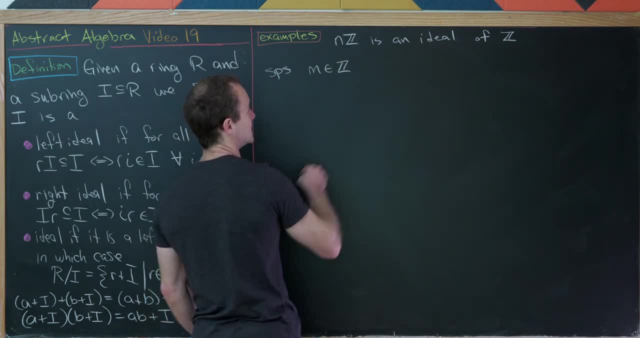 Maybe we'll call it M. So M is an element of Z. 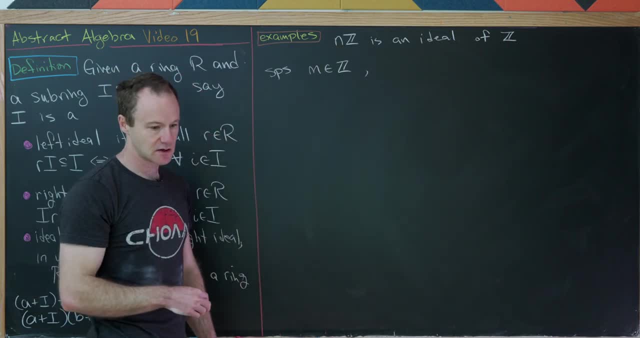 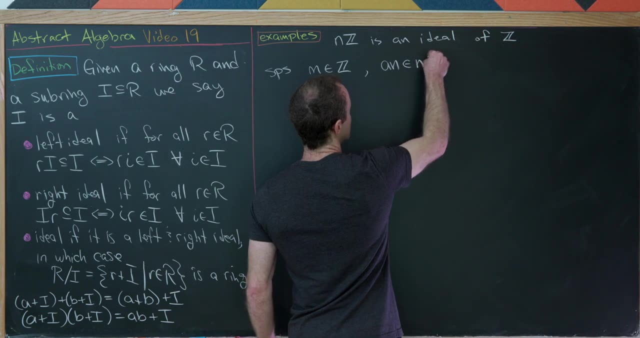 And then we've got an arbitrary element of NZ. But an arbitrary element of NZ is just a multiple of N. So we'll call that AN, which is in NZ. 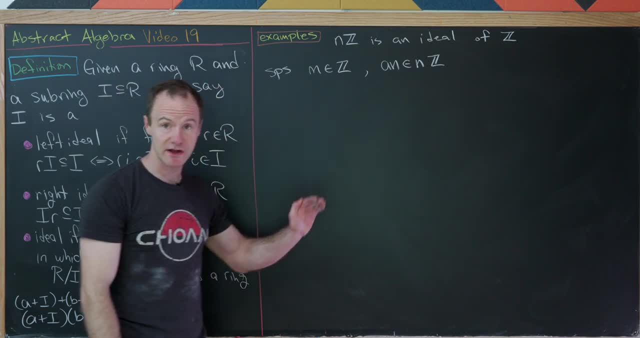 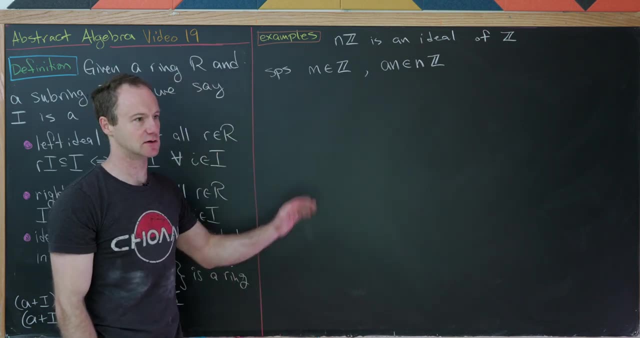 And now let's look at the product of those two. So just to reiterate, we're taking the product of an element of the ring with an element of the ideal. And we should end up in the ideal. That's what's happening over here. 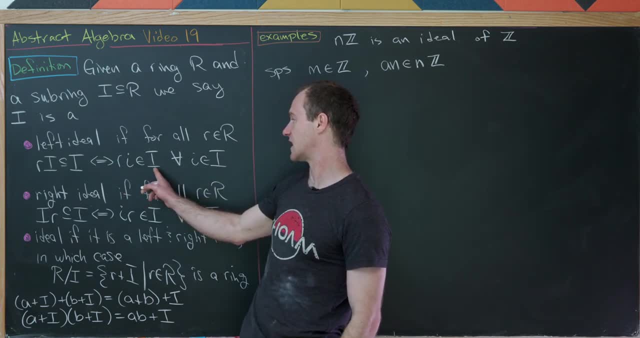 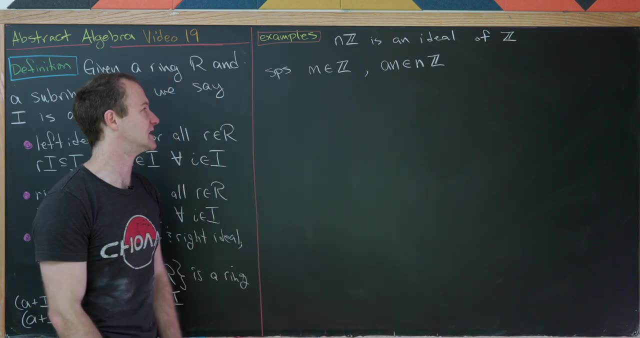 An element of the ring times an element of the ideal is inside of the ideal. An element of the ideal times an element of the ring is inside of the ideal. That's the special condition here. 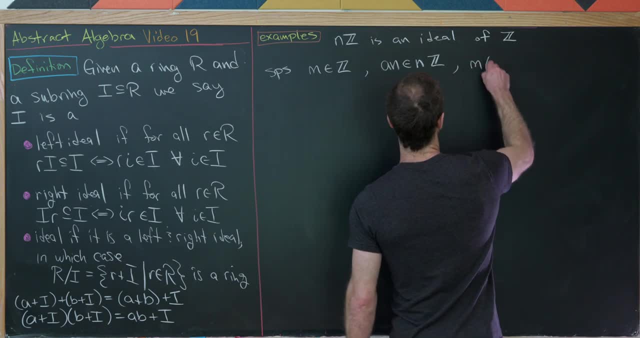 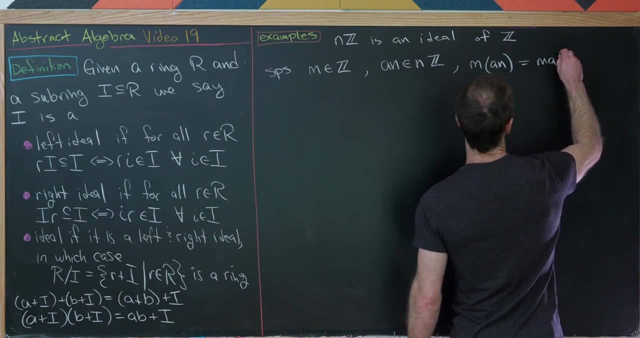 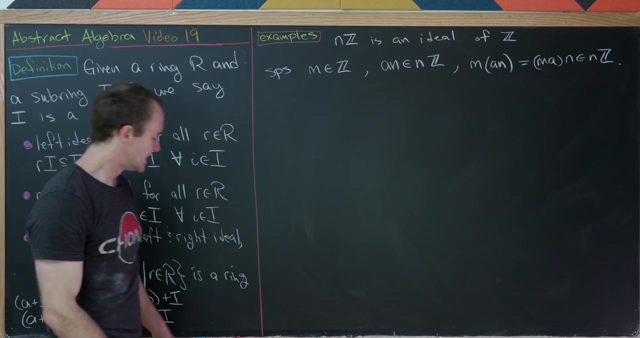 Okay, so we've got M times AN. Well that's going to be equal to, maybe very clearly, MA times N. But that's clearly a multiple of N. So that is within NZ. 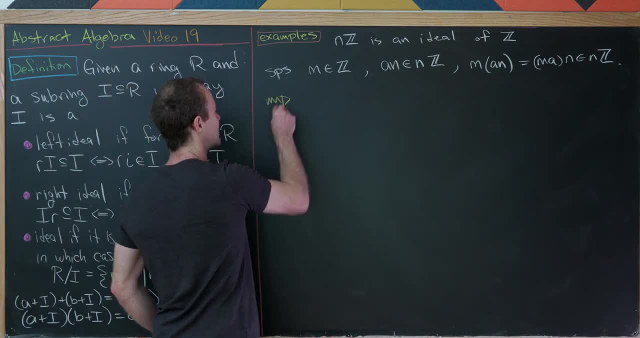 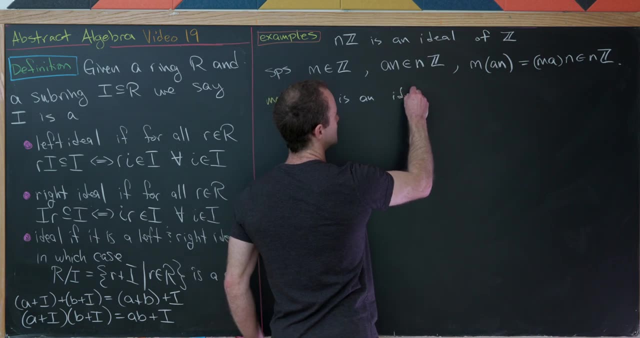 Now if we were to do this on like a specific example, which isn't a terrible idea. Let's say 6Z is an ideal of Z. Okay. 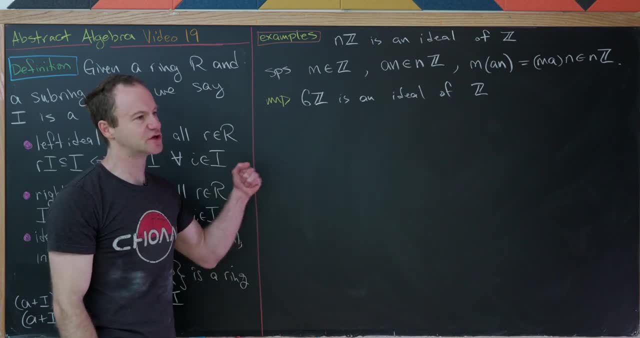 And then let's do this on some example elements. So this will not prove that it's an ideal. 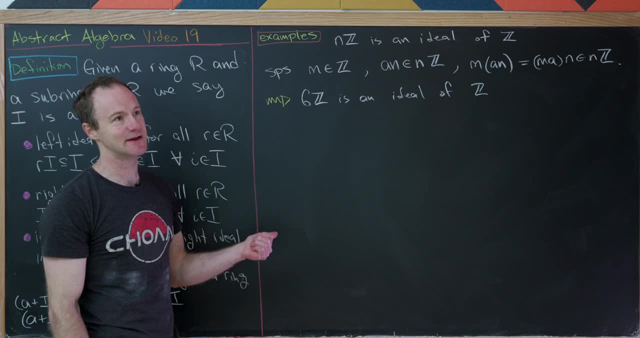 Well we already proved it's an ideal up here in general. It just exhibits the ideal condition. 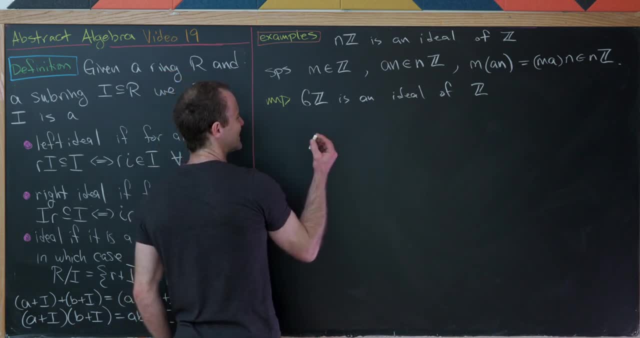 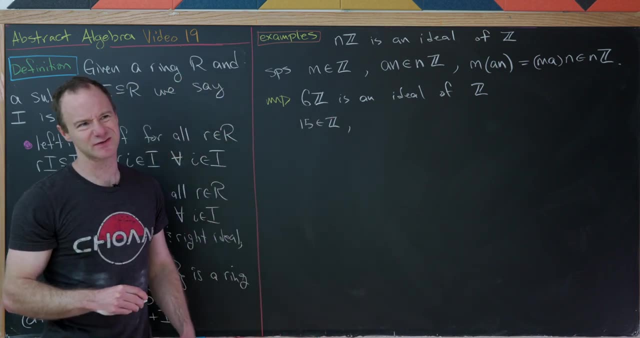 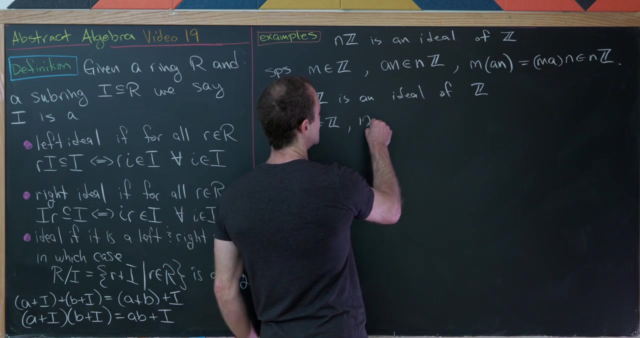 So let's take an arbitrary element of Z. So for instance, the number 15 is an element of Z. And then let's take some sort of random element of 6Z. So that's got to be a multiple of 6. So for instance, 12 is an element of 6Z. 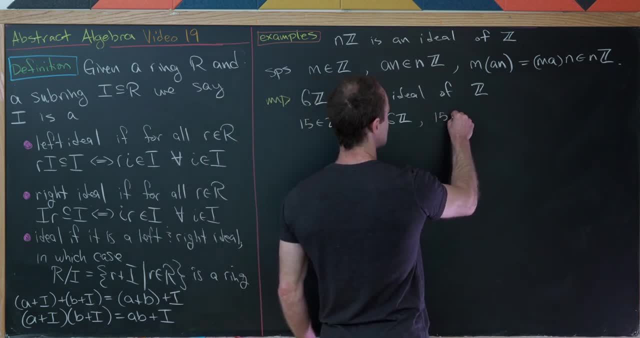 And now let's take their product. So 15 times Z. 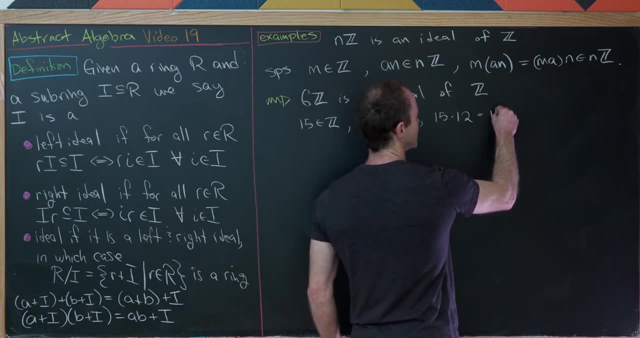 Times 12. Well that can be rewritten as 15 times 6 times 2. 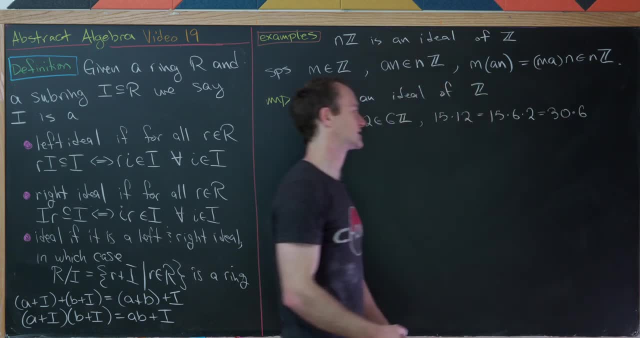 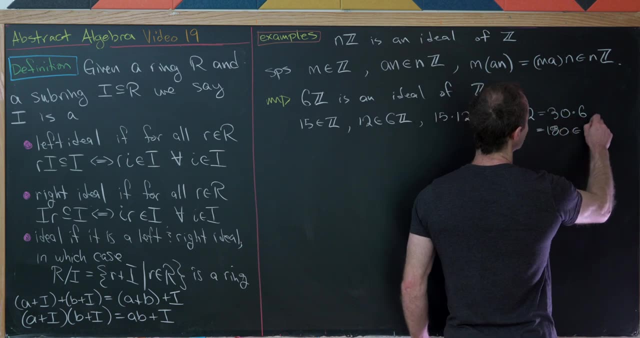 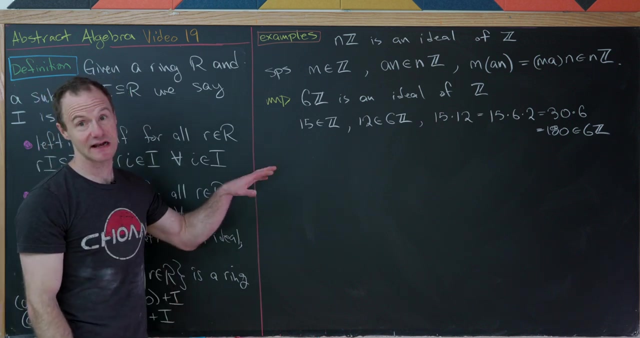 But that's equal to 30 times 6. Oh, but notice 30 times 6 is clearly equal to 180. But that's an element of 6Z because it's a multiple of 6 by our expression above. So that doesn't, like I say, prove that 6Z is an ideal. We did that up here in general. That just like. 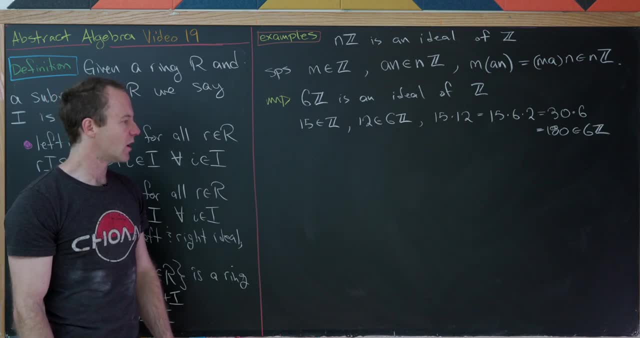 Exhibits the ideal relationship. 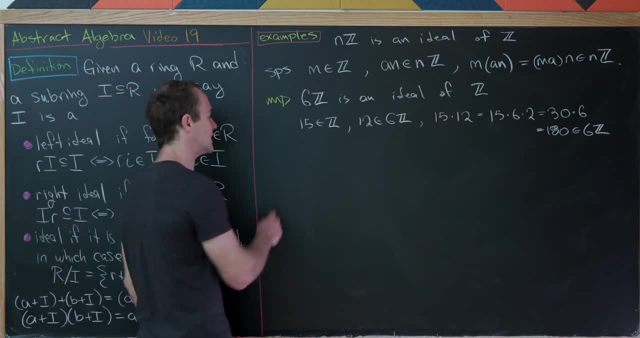 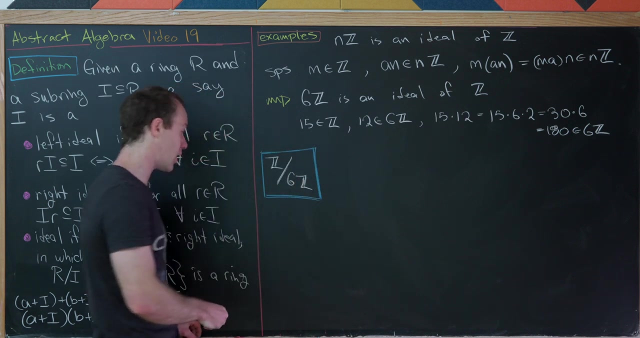 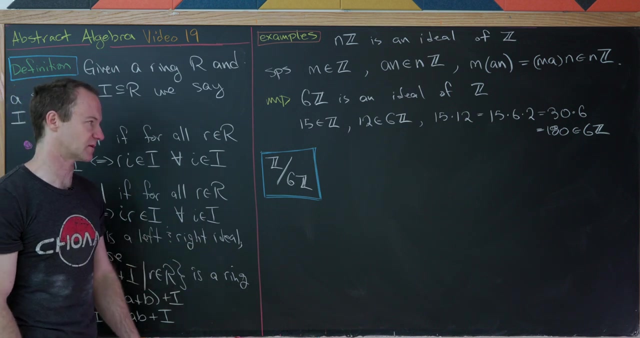 Okay so now let's do some example calculations in the quotient ring. So the quotient ring here is Z mod 6Z. Which we know as a group is isomorphic to Z6. We don't yet know that it's isomorphic to Z6 as a ring. Although we know that Z6 is a ring. But we will prove that later once we know something about the isomorphism theorem for rings. 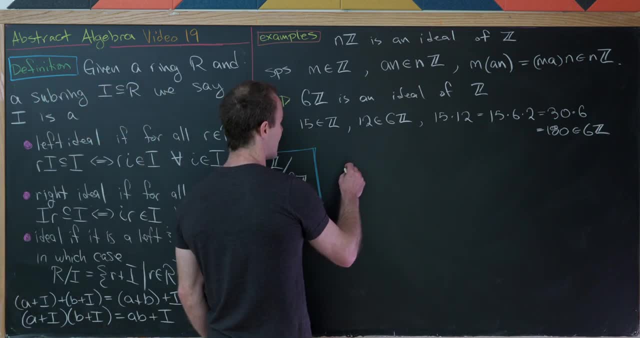 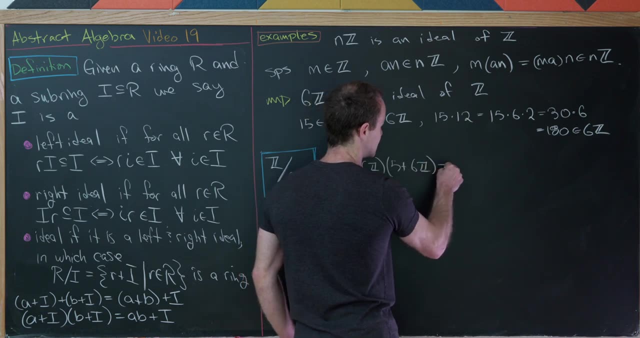 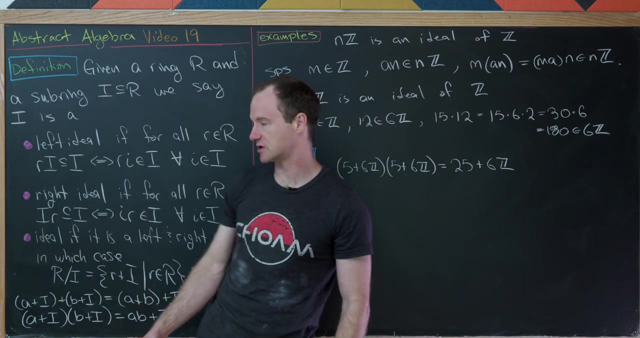 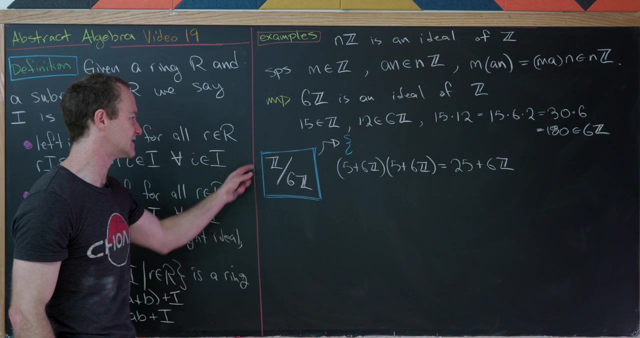 Okay so let's notice for instance that 5 plus 6Z times 5 plus 6Z is equal to 25 plus 6Z. By the definition of the operation. And now we need to reduce that to maybe some which is contained in the typical set of cosets which defines Z mod 6Z. Okay. 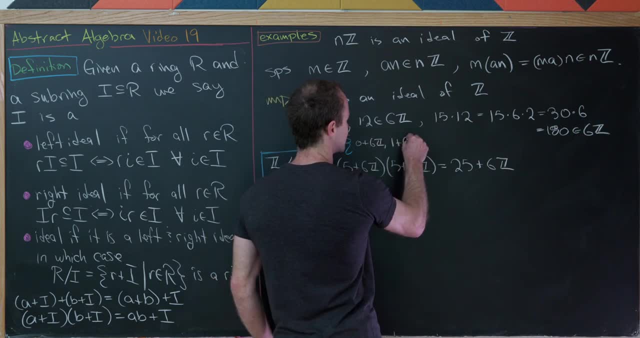 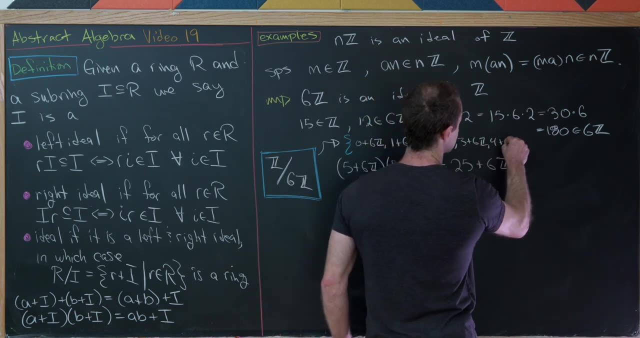 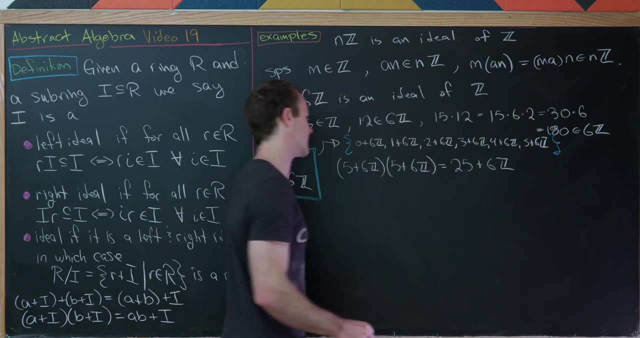 Which would be like 0 plus 6Z 1 plus 6Z 2 plus 6Z 3 plus 6Z and then 4 plus 6Z and then finally 5 plus 6Z. So that would be the typical full list of cosets of Z mod 6Z. 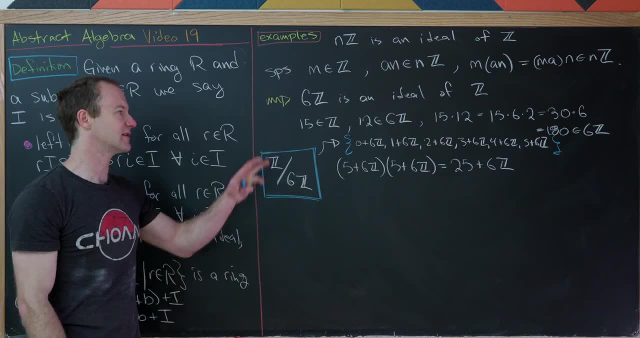 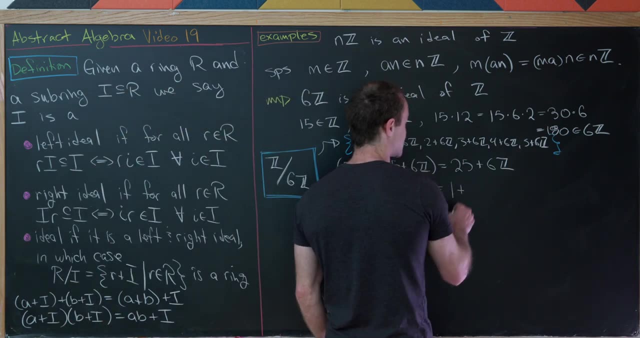 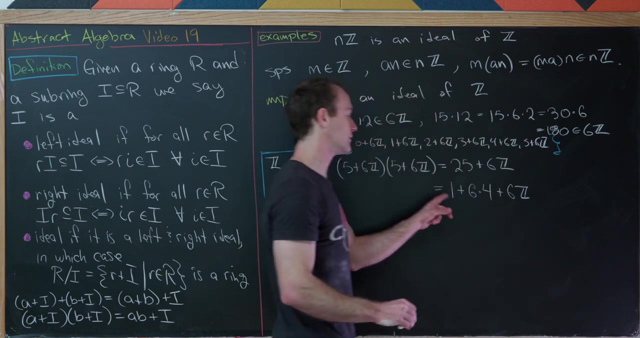 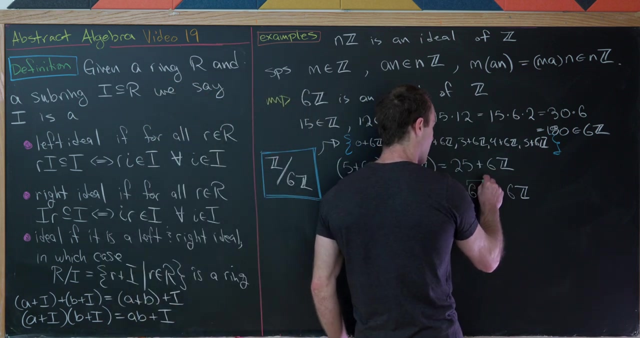 So which one is that? Well I think you can probably immediately see that it's 1 plus 6Z. But let's spell that out. So notice that this is equal to 1 plus 6Z. 1 plus 24. But 24 is the same thing as 6 times 4. So we have this is 1 plus 6 times 4 plus 6Z. But then we're going to use the fact that 6 times 4 is a multiple of 6. 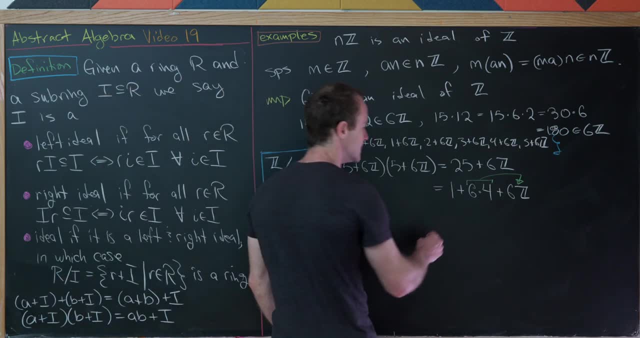 And then absorb it into 6Z. 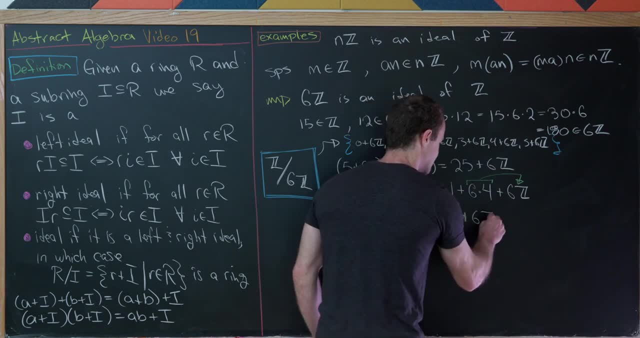 So that means after this absorption we have this 1 plus 6Z. And this is a fairly typical way of doing this. Let's do another example. 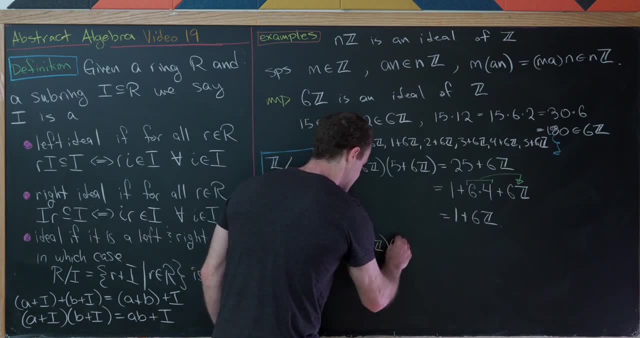 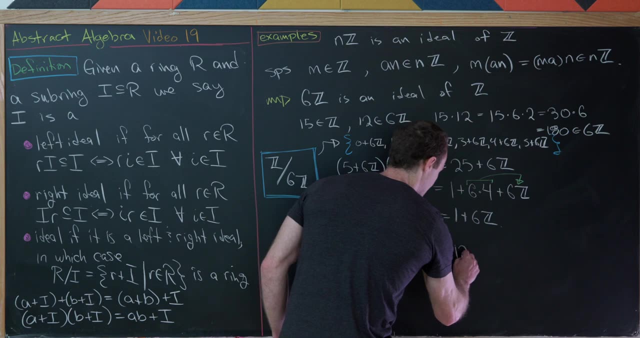 Let's maybe do 3 plus 6Z times 4 plus 6Z. Okay so multiplying those will give us 12 plus 6Z. But then 12 is inside of 6Z so we can absorb it inside of 6Z leaving us 0 plus 6Z. 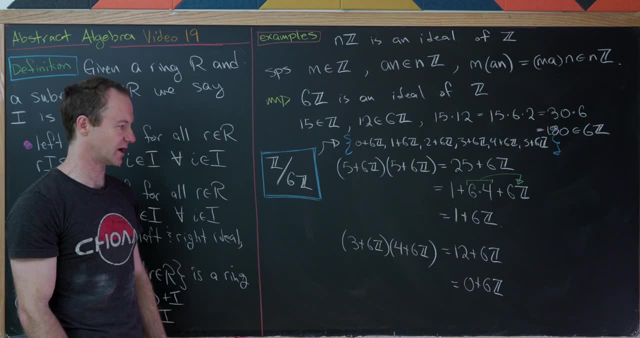 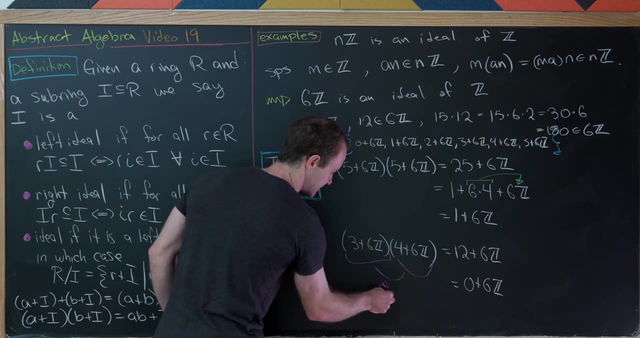 So those are some example calculations inside of this quotient ring. But I'd like to point out. That this means that these two are in fact zero divisors because their product was zero 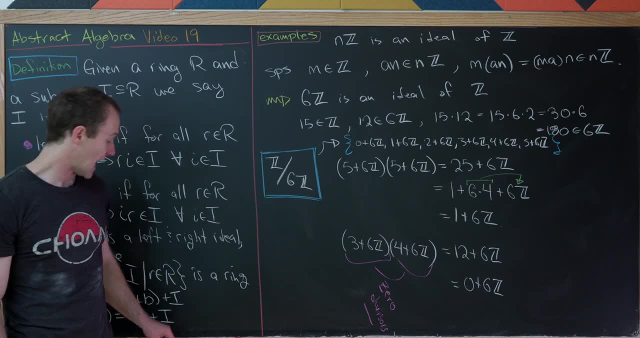 whereas neither of them were zero. 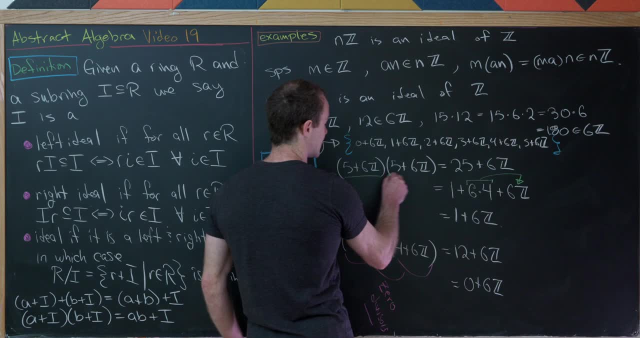 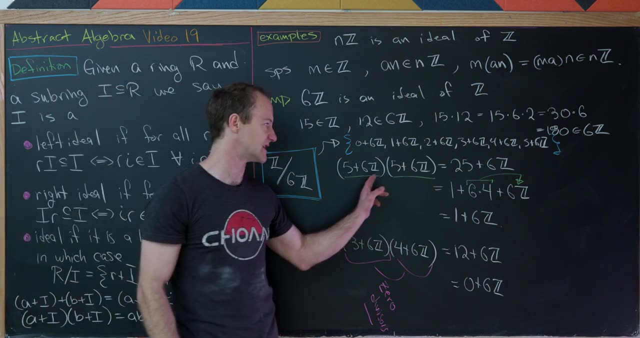 And then this product right here tells us that these two well they're the same number or they're the same element are units. In fact that is its own inverse because their product was equal to the multiplicative identity. 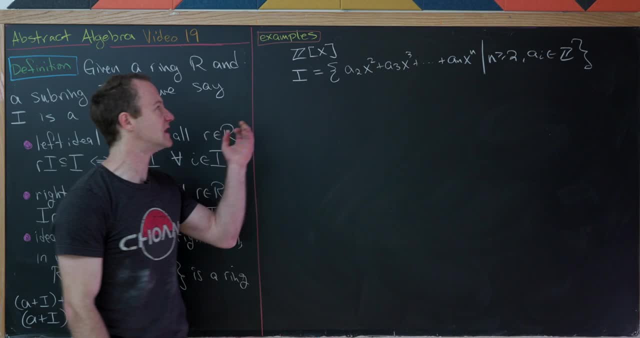 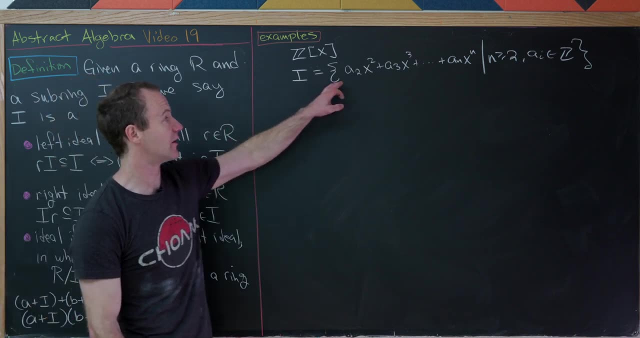 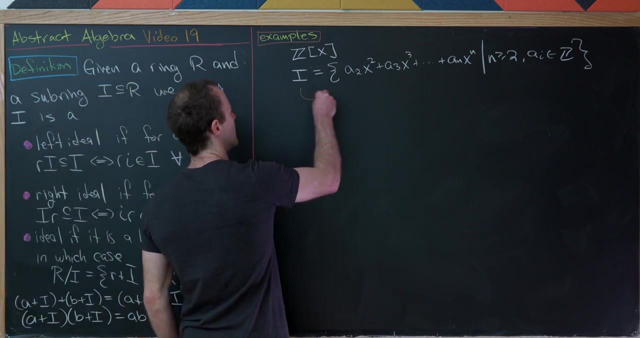 So let's do another example. For our next example let's take the ring to be the ring of polynomials with integer coefficients. And then we'll take the ideal to be all polynomials that have degree 2 or higher. So just as like an example what are some elements in here. So notice that X squared plus 3X cubed is an element of this ideal. Maybe X to the fifth plus 12X to the seventh. So that's the ideal. Okay. 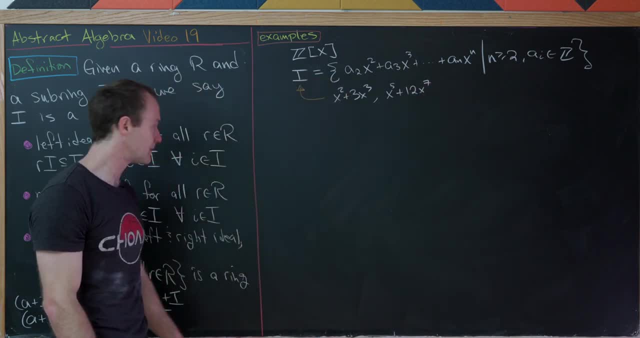 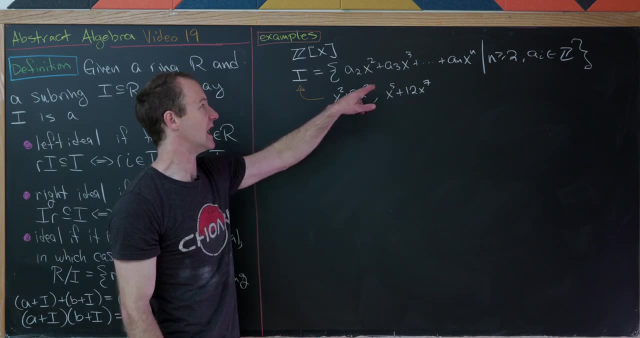 And then the seventh is an element of that ideal and so on and so forth. And here I've written like an arbitrary element of this ideal. It starts at A2X squared, A3X cubed all the way up to ANX to the N. So here N has to be bigger than or equal to 2 because we're starting at a squared term. 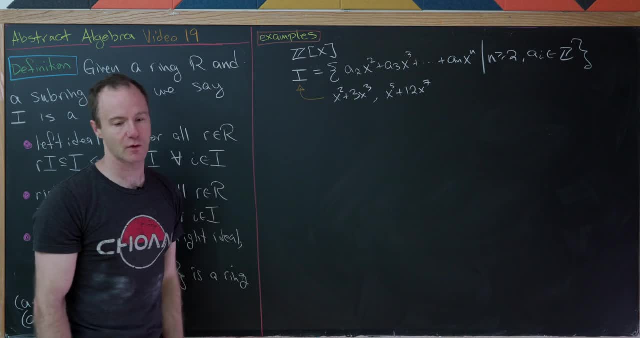 And those AI terms have to be integers just given the fact that we're inside of Z adjoin X. Okay. So let's check that this is an ideal. 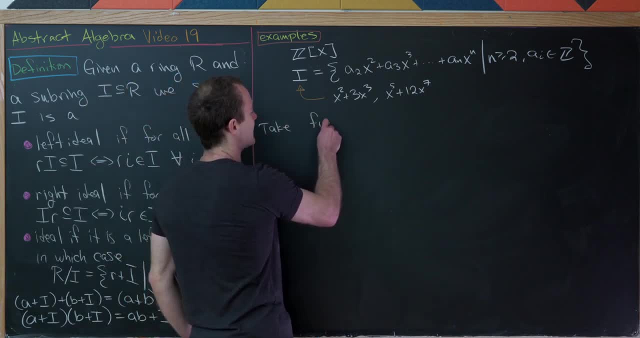 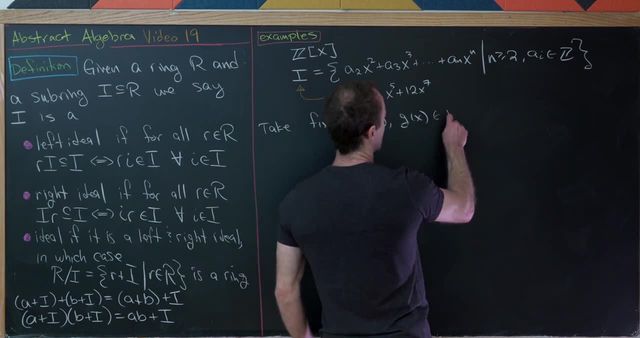 So let's take maybe F of X from Z adjoin X and then we'll take G of X from I. And we're going to use this little fact here which you know I don't believe that we really need to prove. 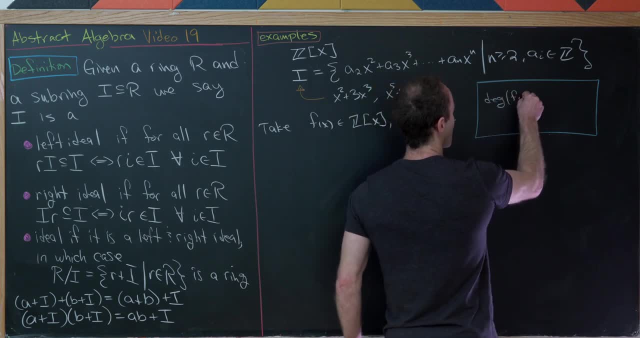 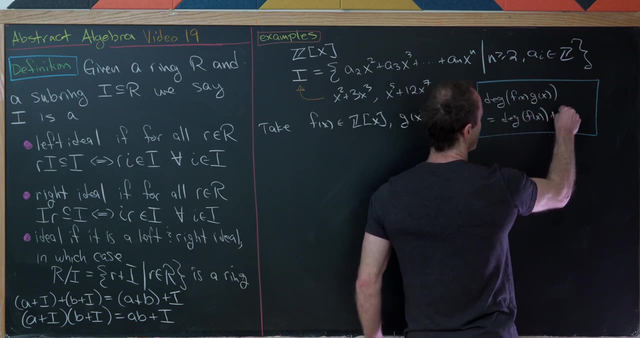 And that says that the degree of F of X times G of X is equal to the degree of F of X plus the degree of G of X. 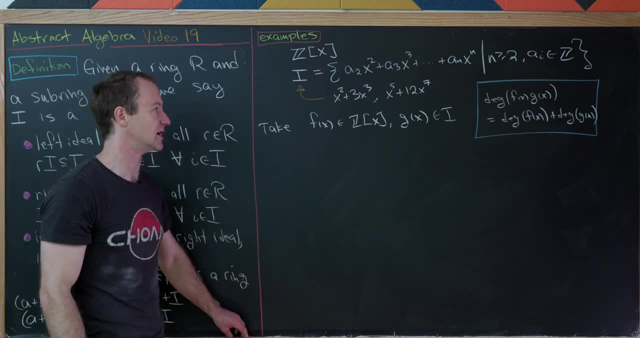 And so just as a quick reminder what's the degree? Well the degree is the largest power of X that we see. 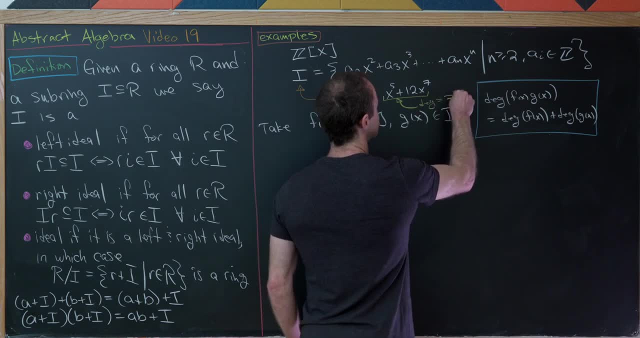 So that means the degree here is equal to 7 because that's the largest power of X we 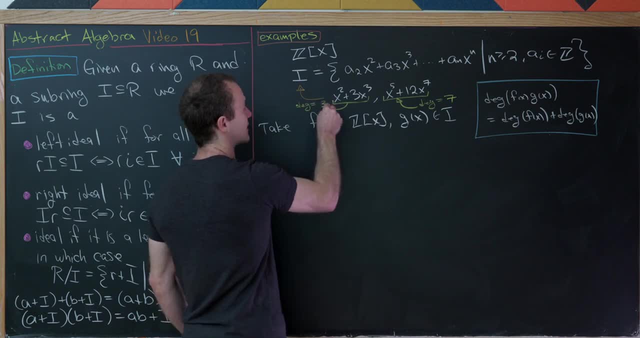 Here the degree is 3 because that's the largest power of X we see. 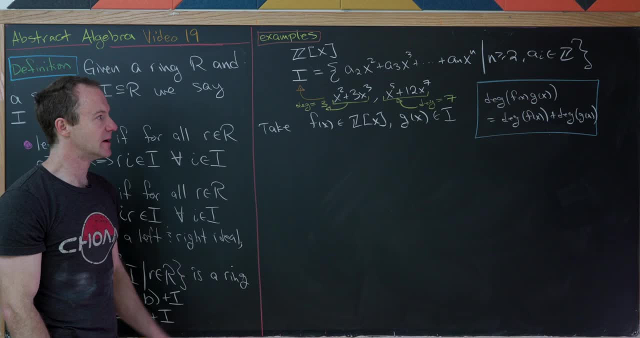 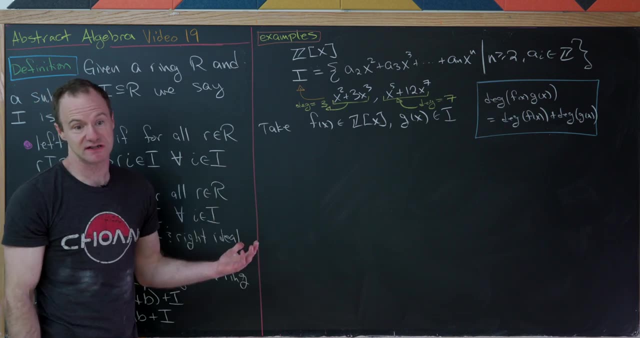 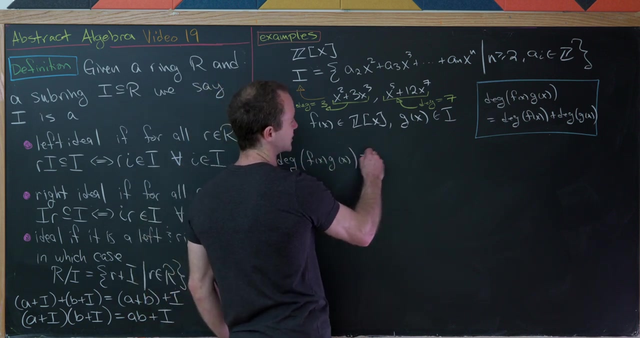 And so now let's take the product of F and G. But we want that product to be inside of I. But in order to be inside of I we need to measure its degree. So let's do that. So let's notice that the degree of F of X times G of X. Well I'm essentially going to rewrite this again. 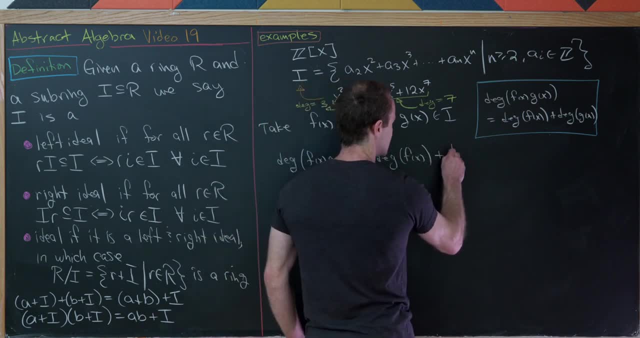 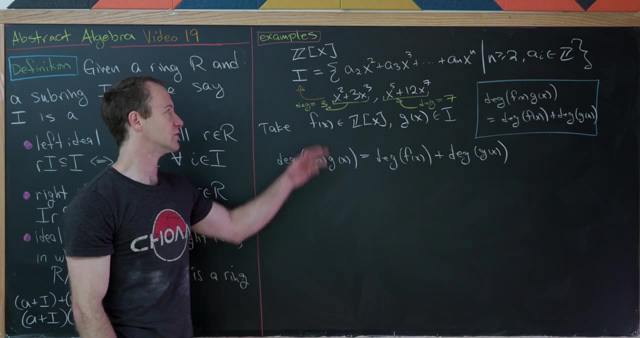 Is equal to the degree of F of X plus the degree of G of X. But the degree is always bigger than or equal to zero. 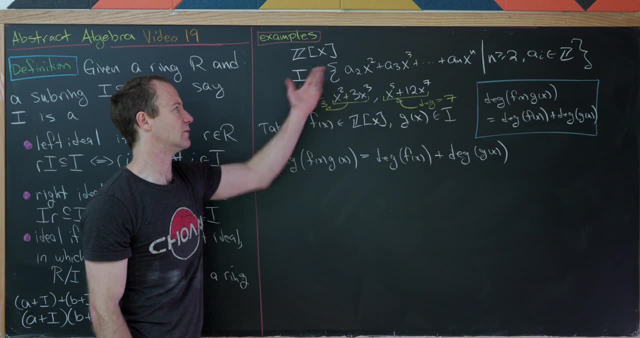 So degree zeros are constants. Degree one. Degree two. Degree three. Degree four. Degree five. Degree six. Degree seven. Degree eight. And so on and so forth. 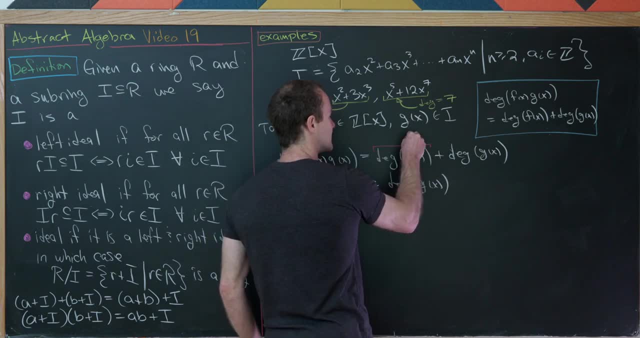 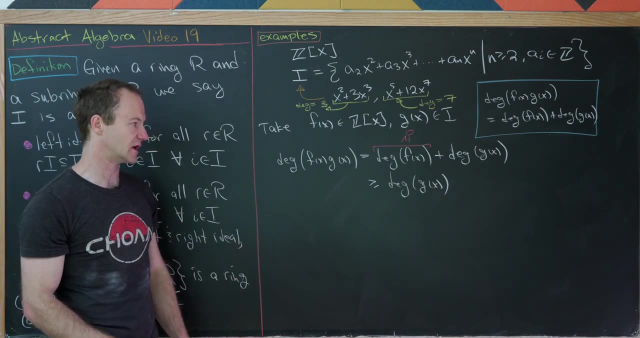 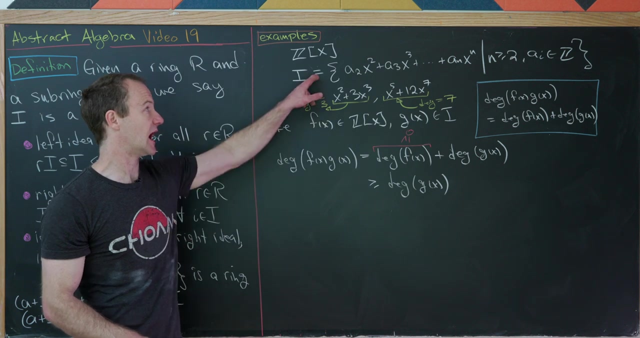 So this is bigger than or equal to the degree of G of X. Because like I just said the degree is always bigger than or equal to zero. So the degree of that is bigger than or equal to zero. So if I drop it I get something bigger than or equal to. But since G of X is inside of I and I contains only polynomials of degree two and higher. 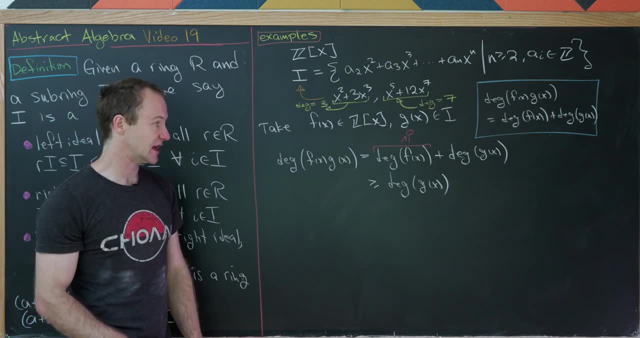 We know that the degree of G of X is in fact bigger than or equal to two. 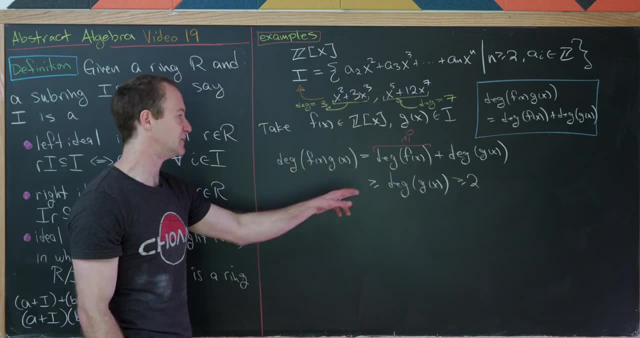 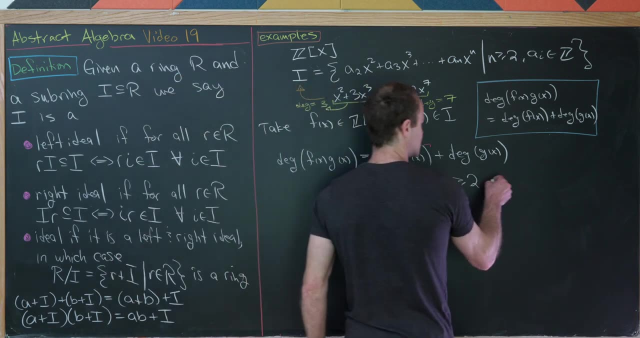 So this is bigger than or equal to two. And that's because G of X is in I. But that's exactly the condition to be inside of I. So the degree of the product is bigger than or equal to two. Meaning that this product is inside of I. 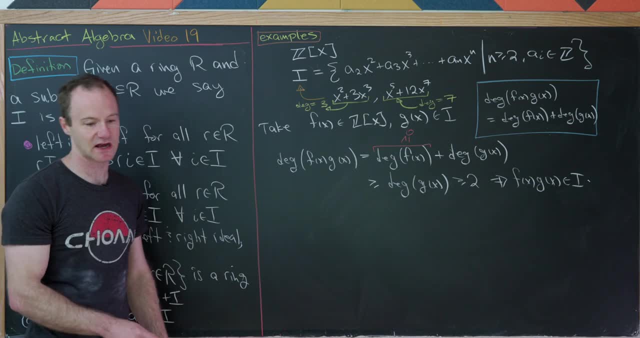 Because it's like found the condition to be inside of I. 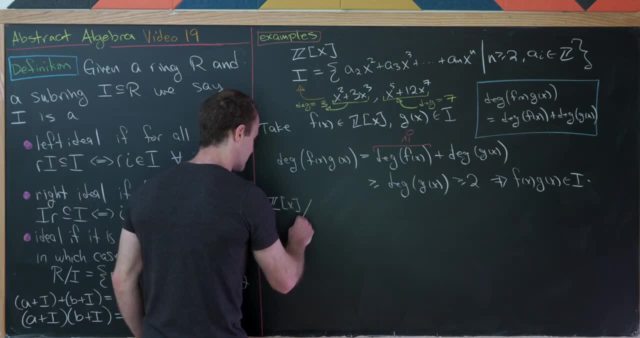 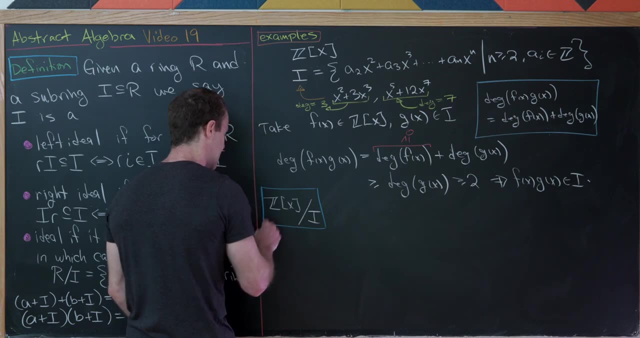 Now that we've done that let's do an example calculation. Inside of Z adjoin X mod I. So in other words inside of this quotient ring. 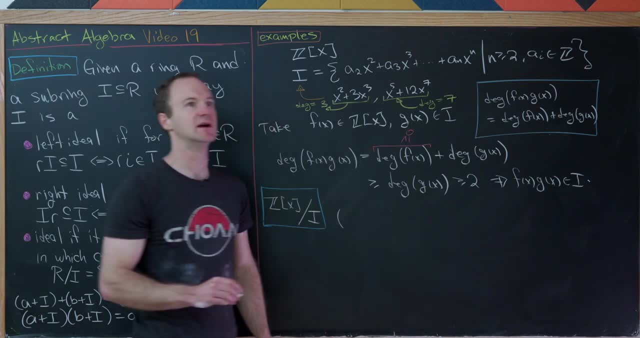 Okay well let's first start by simplifying some sort of polynomial coset. 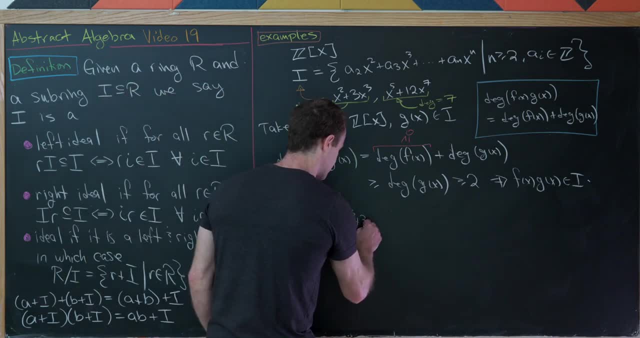 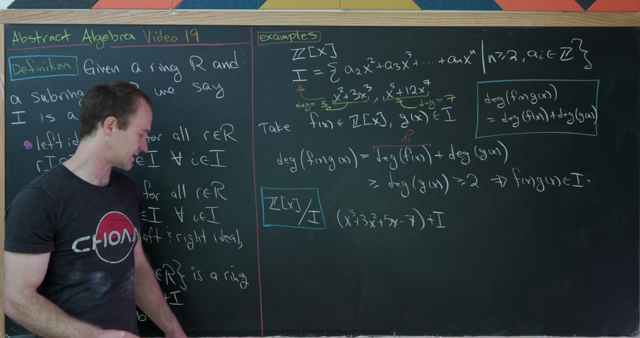 So let's look at the polynomial X cubed plus three X squared plus five X minus seven plus I. So that coset. 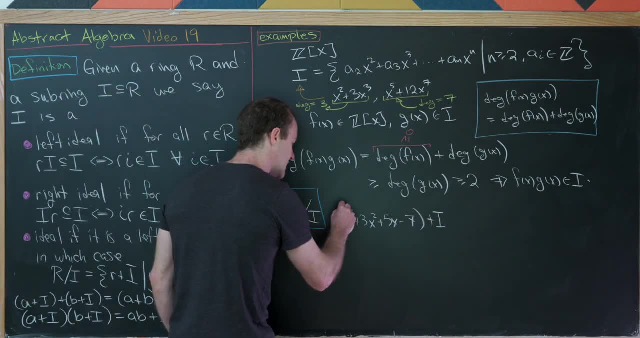 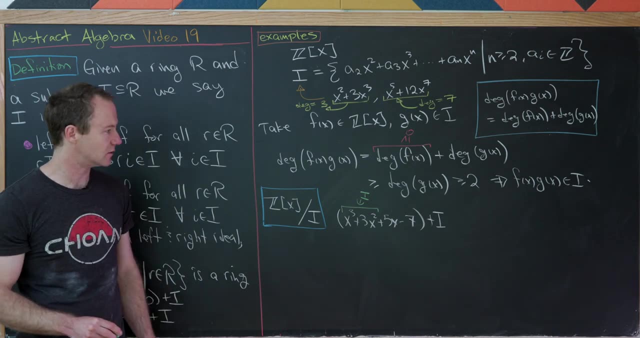 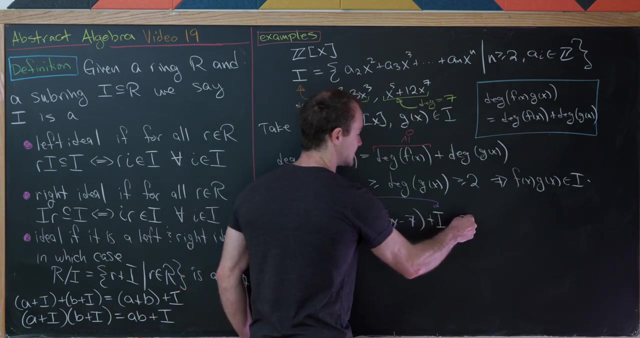 But let's notice that everything in this equation. The ring up here is an element of I. Because those two terms have degree bigger than or equal to two. So that means we can take those two terms. And absorb them into the ideal. Giving us this coset equality. 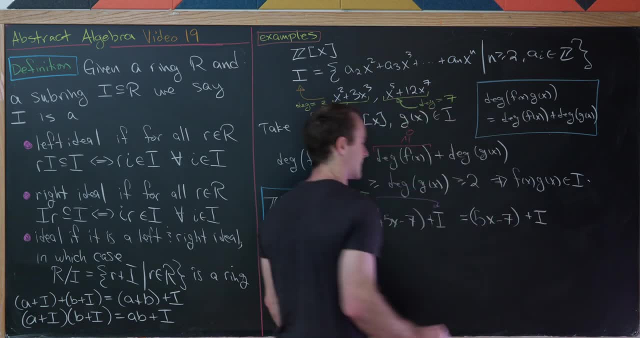 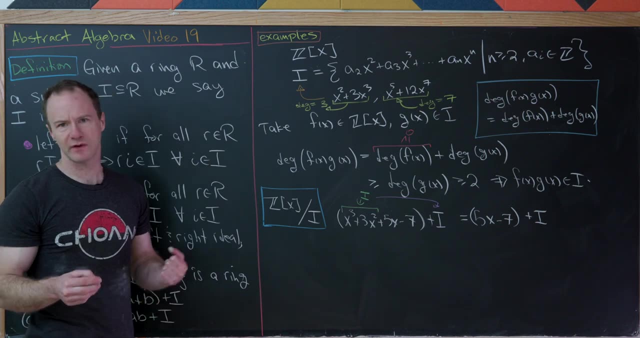 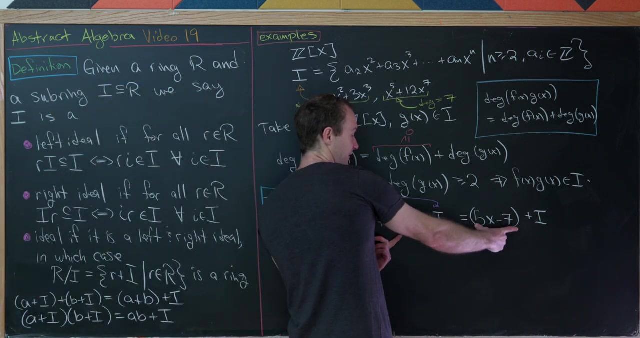 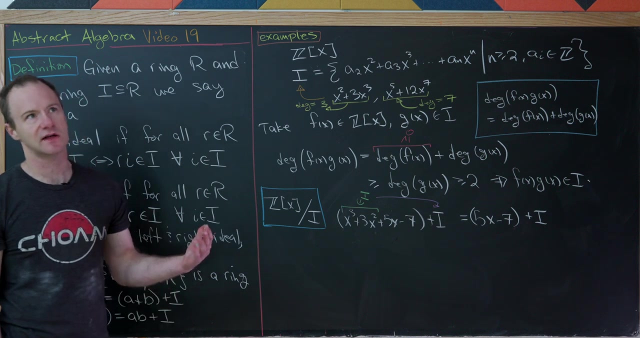 That this is equal to the coset five X minus seven plus I. So there we did that quick absorption. In order to show that we got a simpler coset. Now you could of course go back to that coset equality theorem. And say that the difference in those two. Is equal to this thing that I've over lined in green. Which is an element of I. So that means that those two cosets are equal. But this absorption is like a quicker way of doing that. 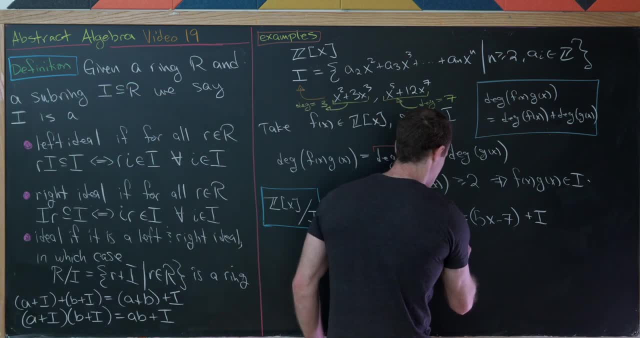 Okay so notice that this means. That everything or all of the cosets can be written like this. 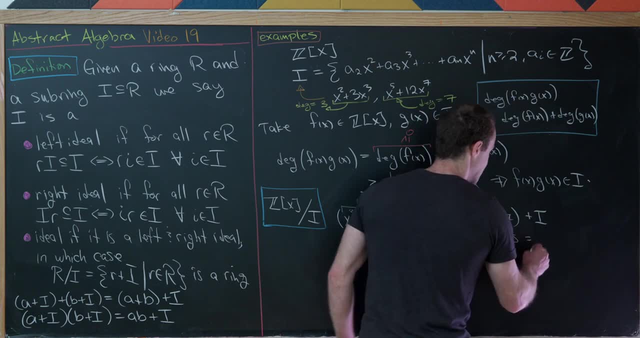 So all cosets. Will equal. 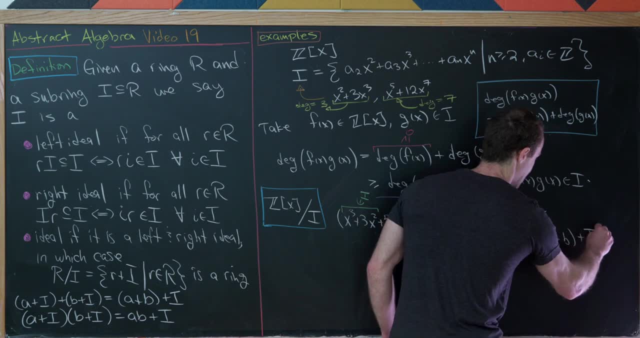 AX plus B plus I. That's because you can always take those higher terms. And absorb them into I. 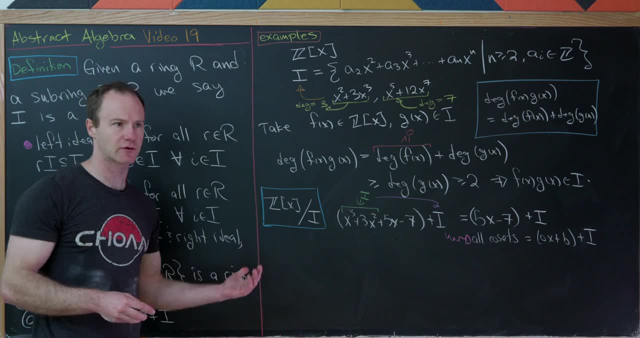 Okay so now let's do maybe a general. Yet an example calculation. 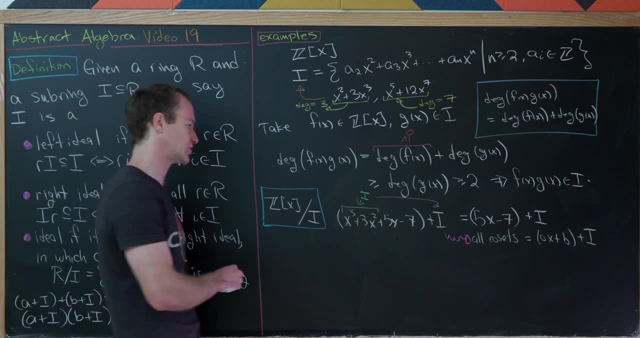 Of a product inside of this quotient ring. 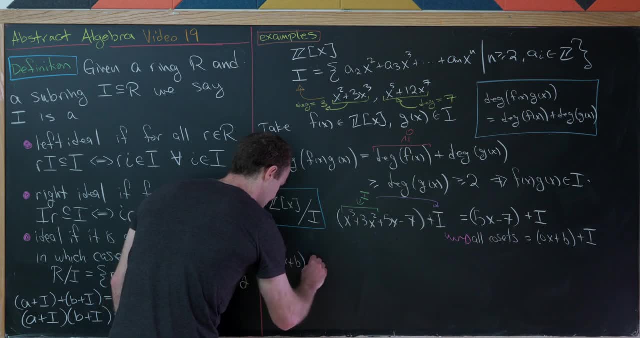 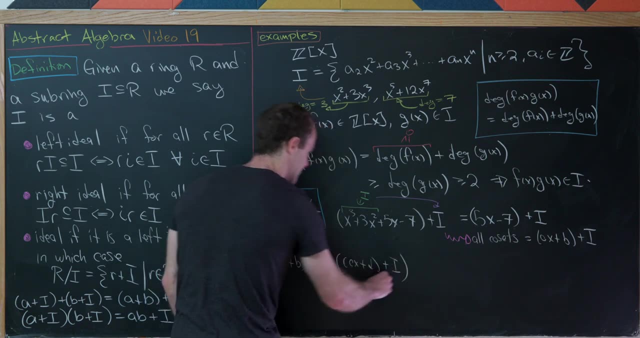 Let's take AX plus B plus I. So that coset. And let's multiply it into the coset CX plus D plus I. 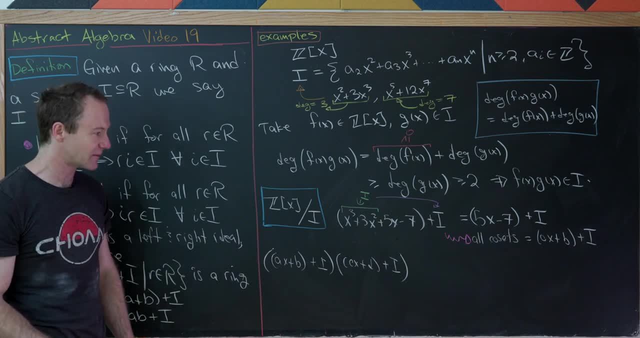 So that's as arbitrary as a multiplication. That we need to think about. 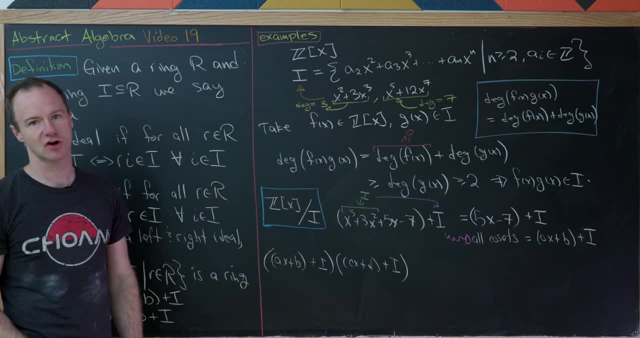 Because all the cosets can be simplified. Like we described before. Okay so this is going to be equal to. 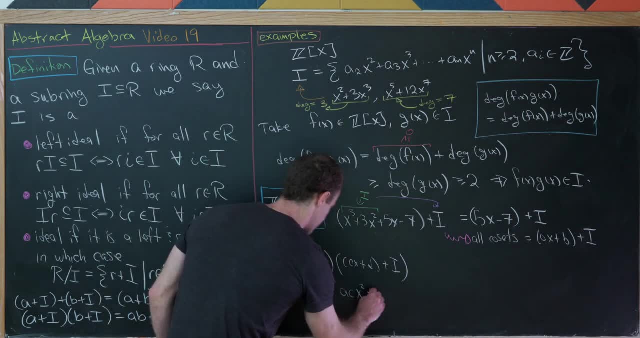 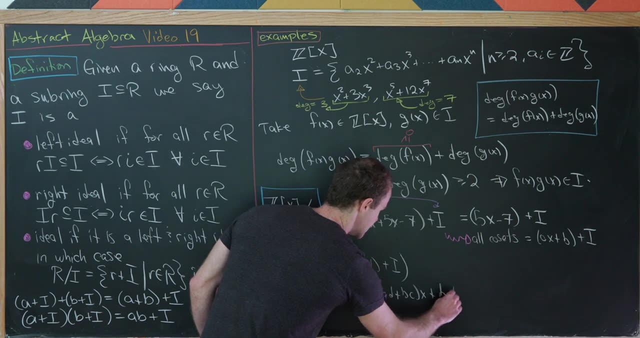 Well let's see it will be ACX squared. Plus AD plus BC times X. Plus BD. 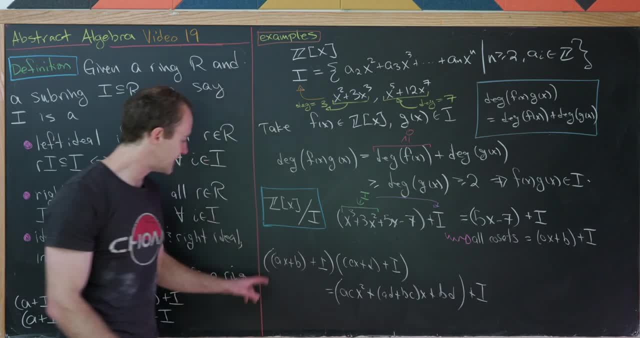 And then. Plus the ideal. That's just from foiling out those two things here. 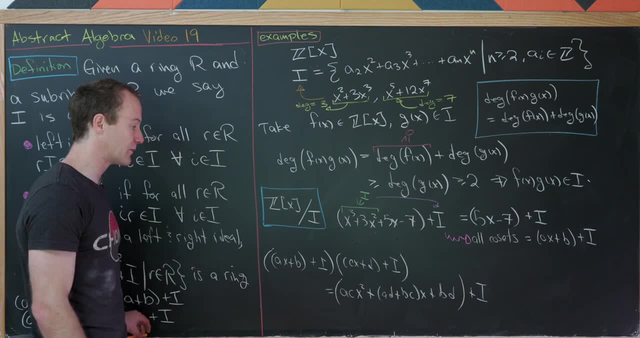 Okay but then we can take. All of the portions that have degree. Bigger than or equal to two. 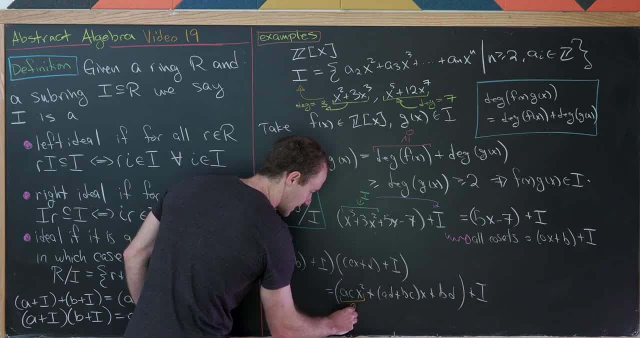 And absorb them into the coset. So that's an element of I. I should say absorb into the ideal. So that's an element of I. So we can absorb it into the ideal. 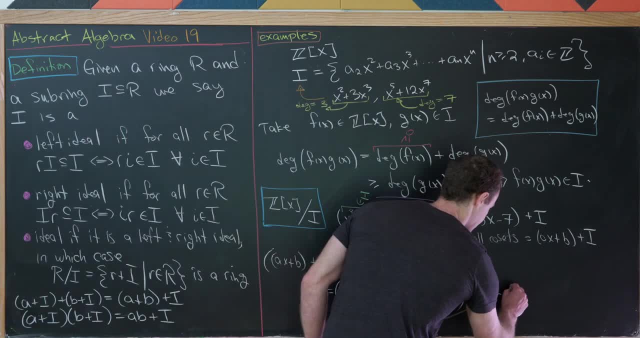 Leaving us with. The following object. AD plus BC times X. Plus. 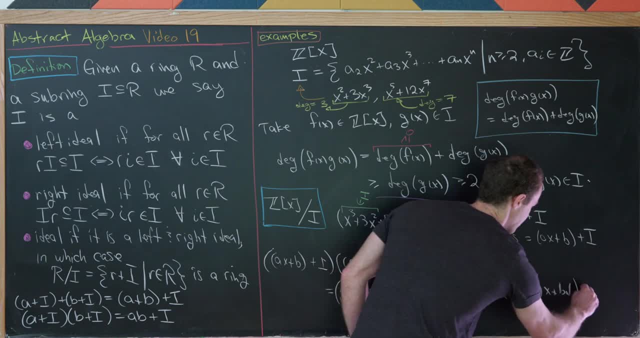 BD. And then plus I. So that would be maybe the simplest product. Of these two objects. 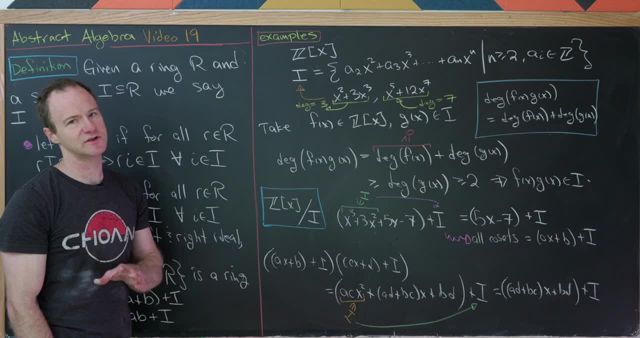 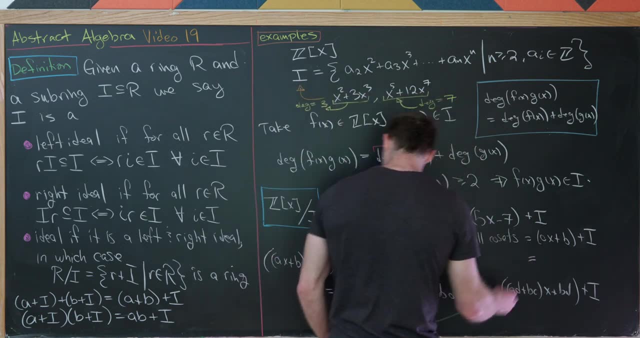 So now I want to introduce like a little bit more notation. That we're not going to use so much. But you can use for simplification. And that is sometimes. 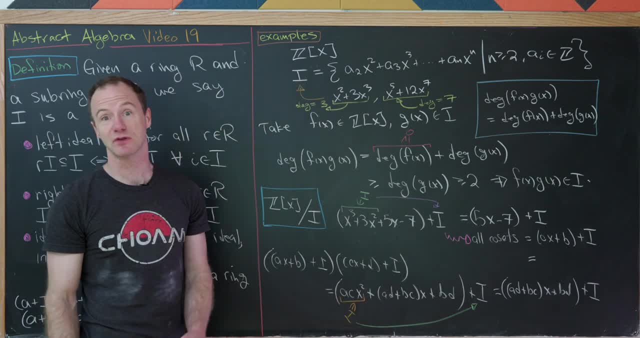 We would take this coset. AX plus B plus I. And rewrite it as AX plus B. 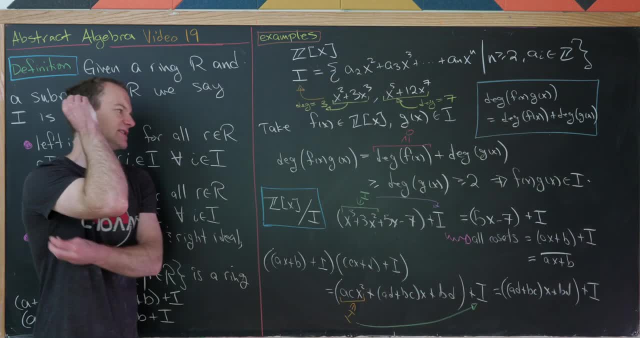 With an overline. And maybe we would read that as like. AX plus B bar. And that's just maybe a shorthand. 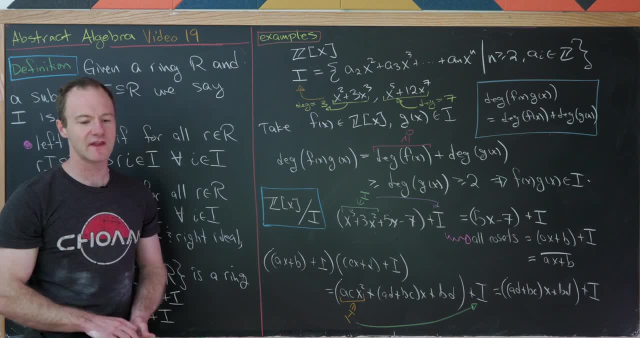 For saying that we're passing to the quotient. Okay so now that we've done that. 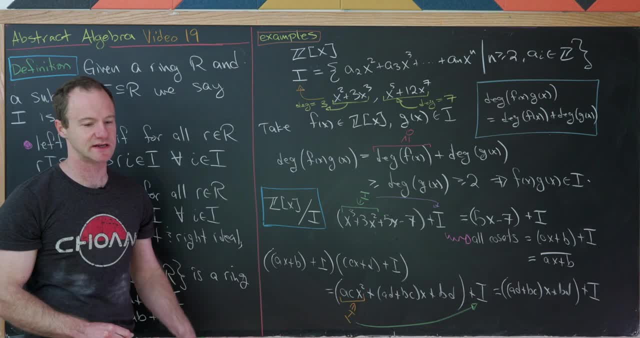 I want to look at a way of building. New ideals from old ideals. So in order to make some new ideals. From old ideals. 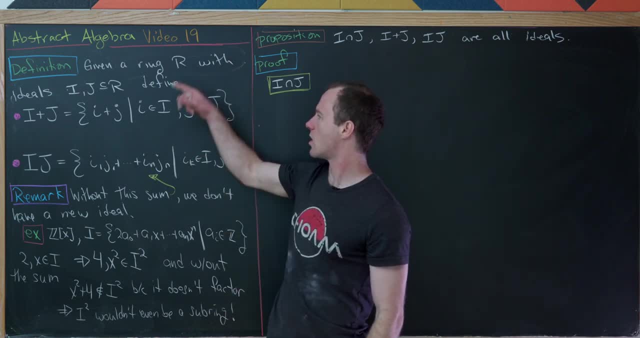 We need some definitions. And so let's say we've got a ring R. And we've got two ideals of R. Which are I and J. Then we can define their sum. 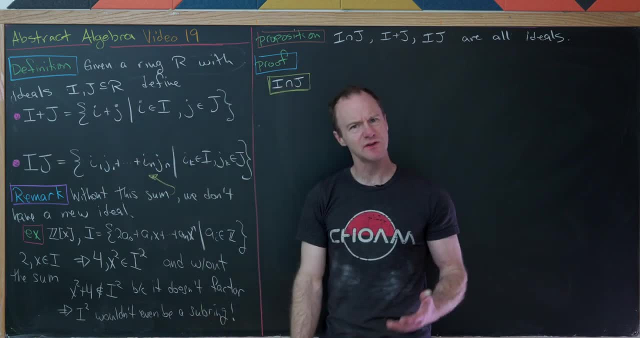 Which we'll call I plus J. To be everything of the form. Little I plus little J. Where little I is in I. And little J is in J. So that's the sum of two ideals. 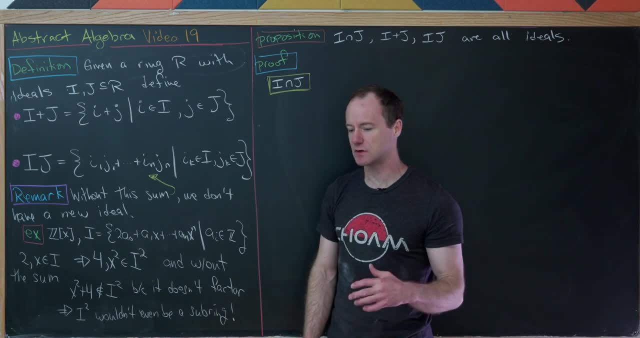 And then we could define their product. Similarly. Although not exactly the same as we'll see. 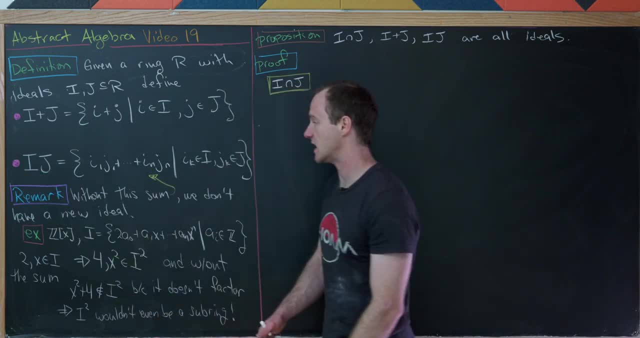 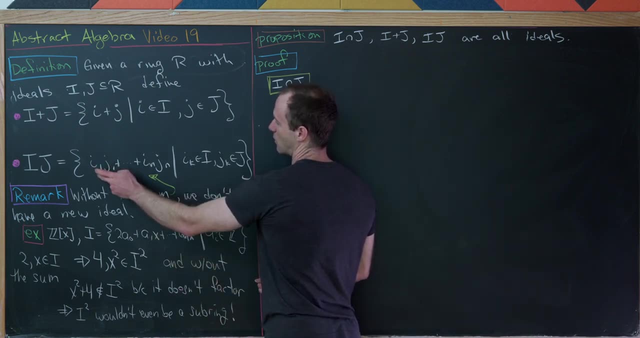 So the product. I times J. Will be all finite sums. Of products of elements. So in other words. Like I1 times J1. Plus I2 times J2. Up to IN times JN. Where all of the IKs. 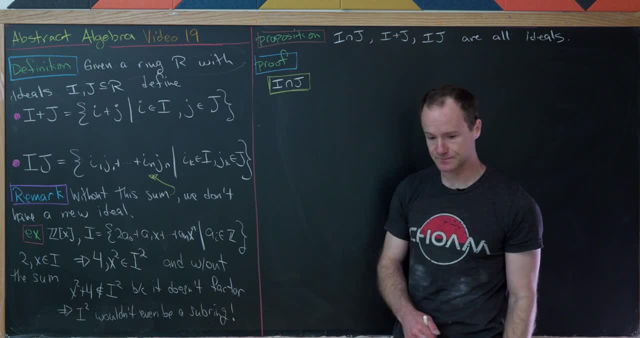 Come from I. And all of the JKs come from J. 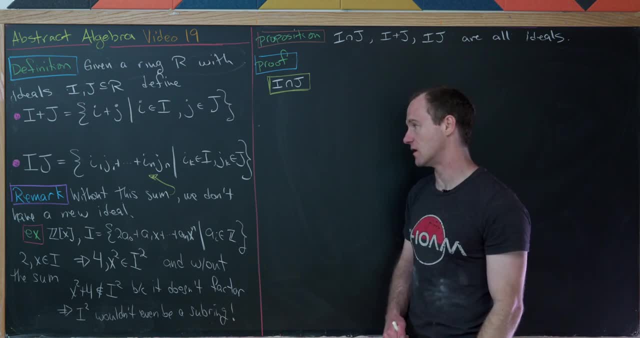 And you might ask. Well why do we need this sum? 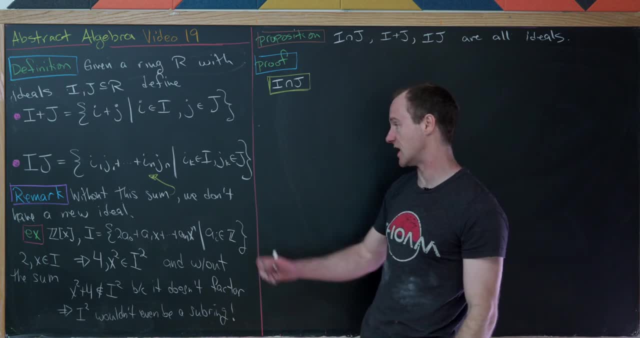 Why couldn't it just be everything of the form. I times J. 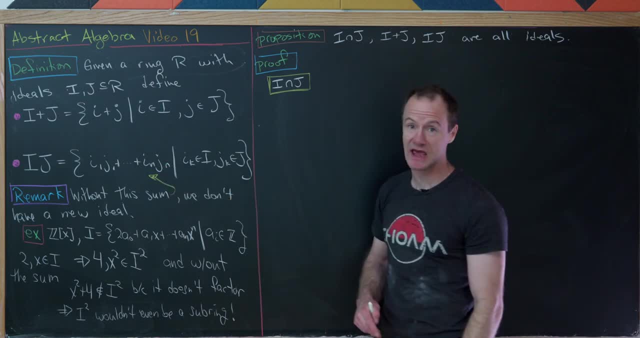 Well without this sum. Built into the game. We don't get a new ideal. 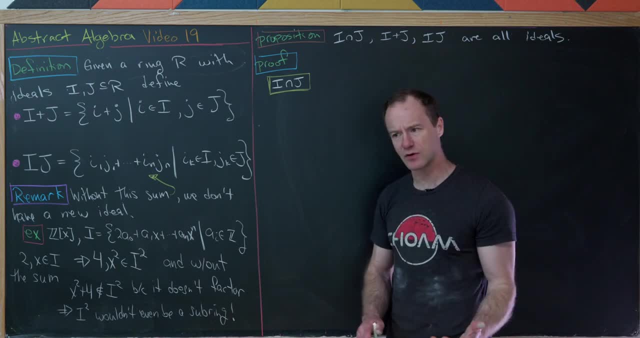 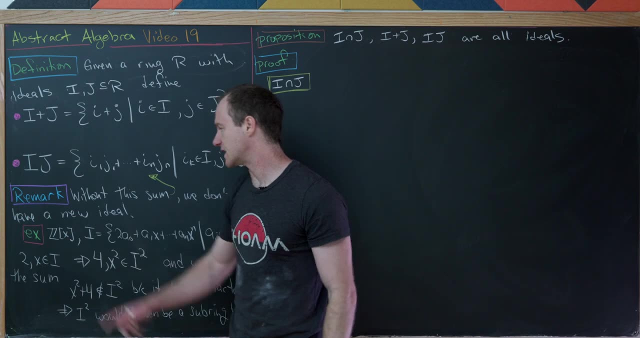 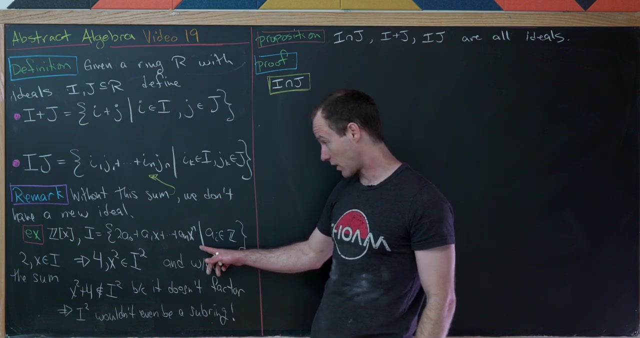 In fact we don't get a new subring. And being a subring. Is necessary for being an ideal. And we can show that. With the following example. Let's take the ring Z adjoin X. And we'll take the ideal. To be all polynomials. Where. 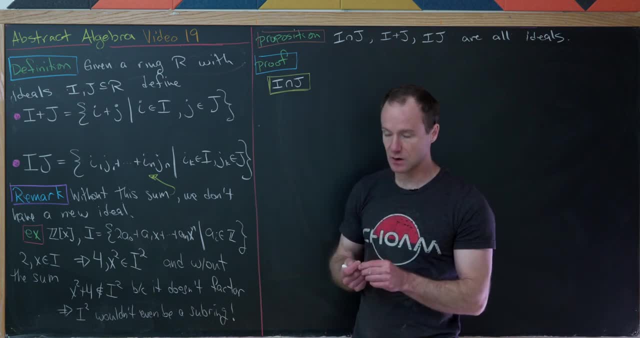 The constant term is even. So. 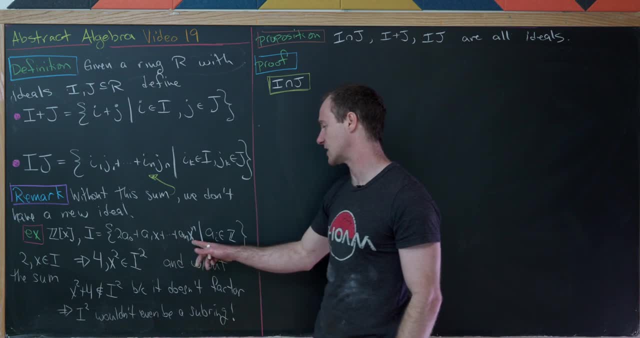 This is going to be everything of the form. 2A0 plus A1X. Up to ANXN. Where all of those AIs are integers. 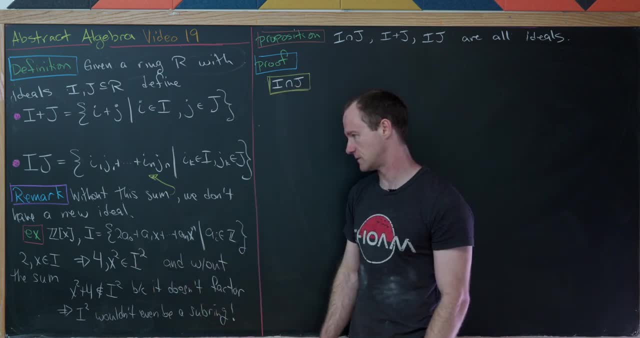 And this too ensures that the constant term. Is even. And for the product. 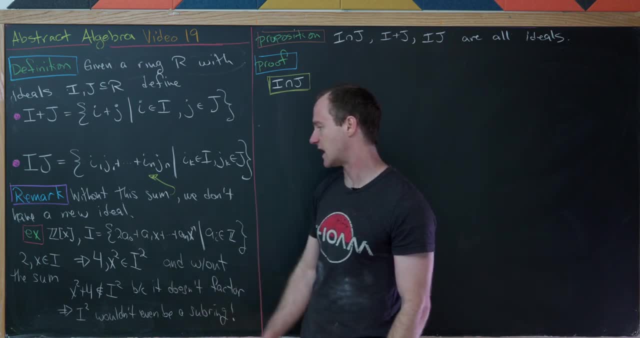 We'll just take two copies of I. And we'll denote that by I squared. So let's notice that. 2 and X. Are both elements of I. 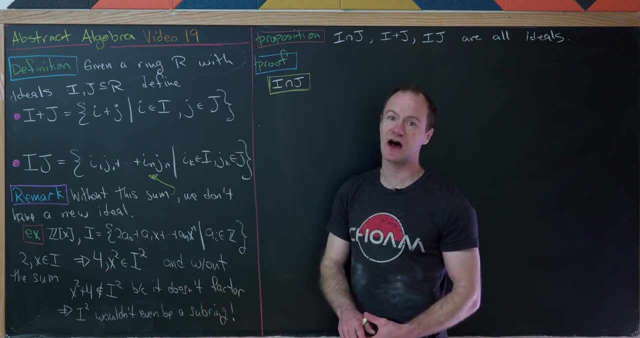 But that means 4 and X squared. Are both elements of I squared. 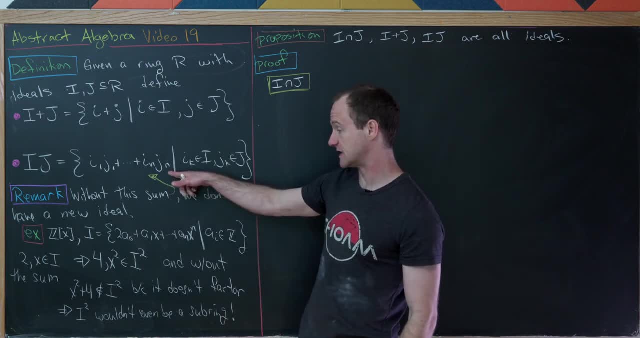 But if we do not. Allow sums here. 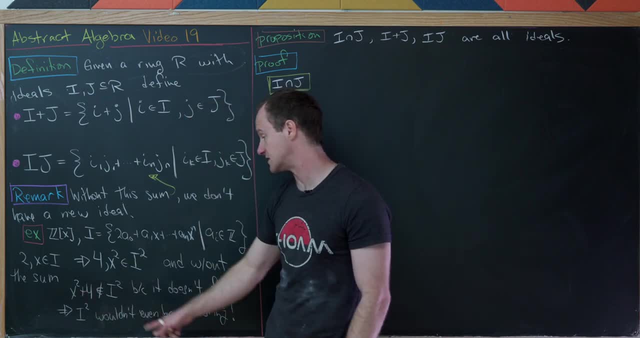 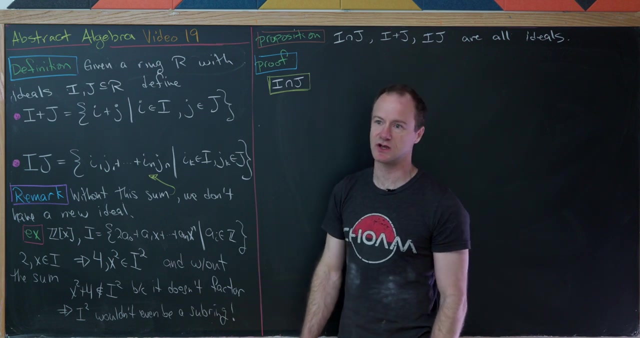 Then X squared plus 4. The sum of these two. Will not be an element of I squared. And that's because. You can't factor this thing. This polynomial. Does not factor over the integers. That means without these sums. We would not have closure under addition. 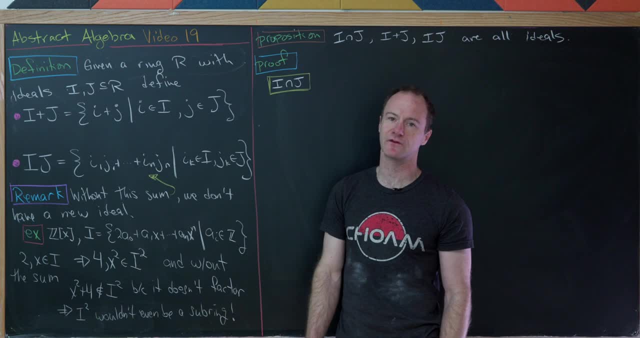 But if we don't have closure under addition. We're not even a subring in the first place. 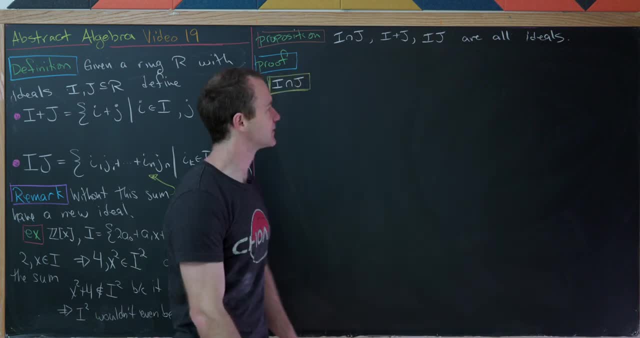 Which means. We can't even start to be an ideal. 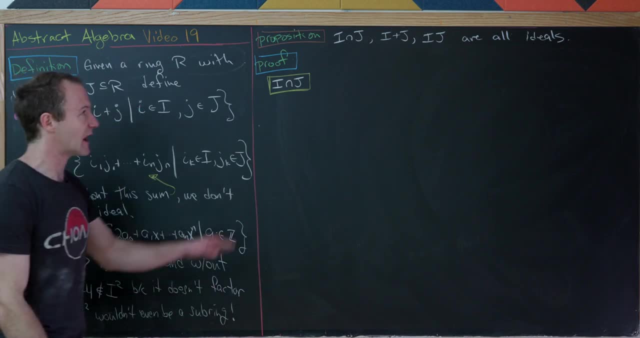 So now let's do the following proposition. So and that will be. That I intersect J. I plus J. And I times J are all ideals. 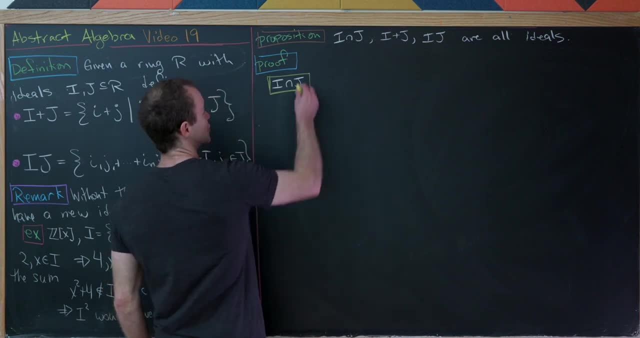 And notice. Really the first thing. That I want to check here. 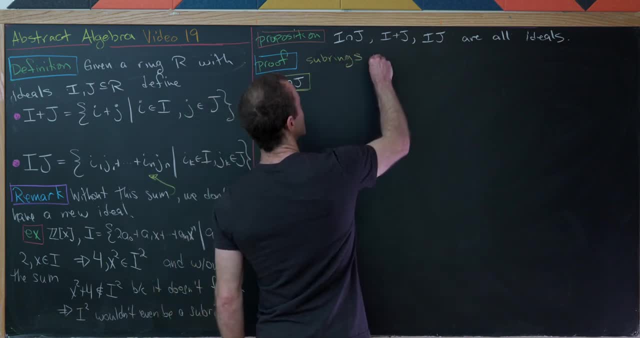 Is that they are all subrings. But I'm actually going to let you. Check that as a little exercise. 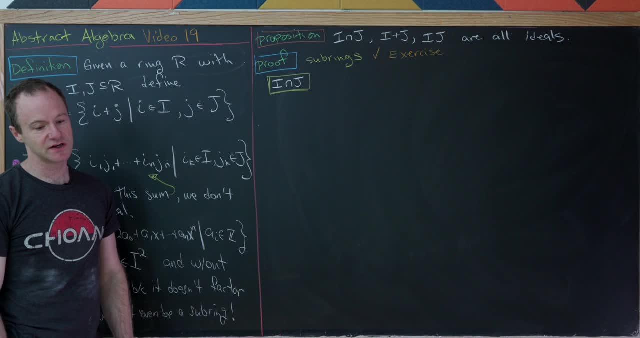 I think that's fairly easy to check. And it makes a good exercise. So let's show that they're ideals. 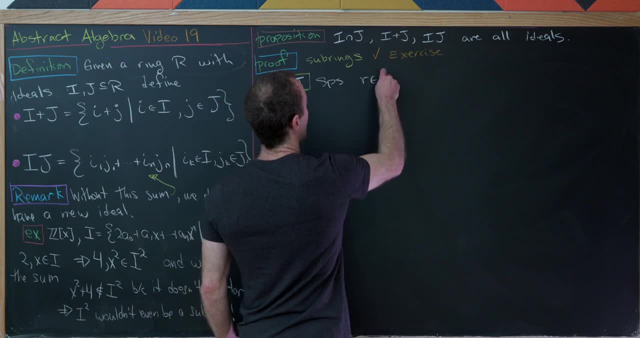 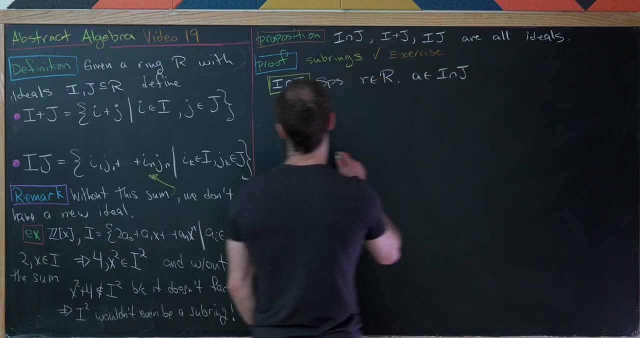 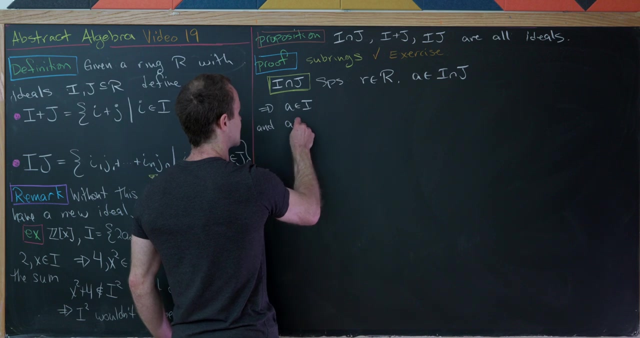 Okay so let's suppose. That we have R. An element of R. And we have A. An element of I intersect J. But notice that that means. That A is an element of I. And. A is an element. 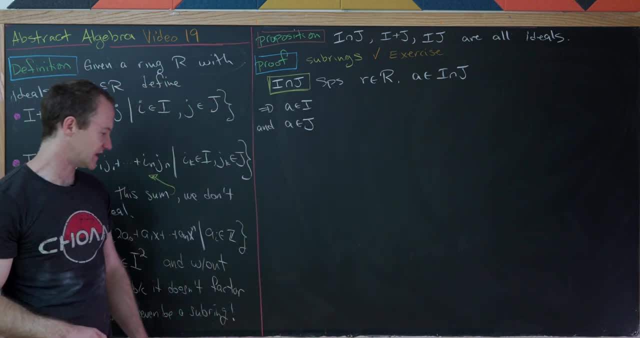 Of J. That's the definition of intersection. 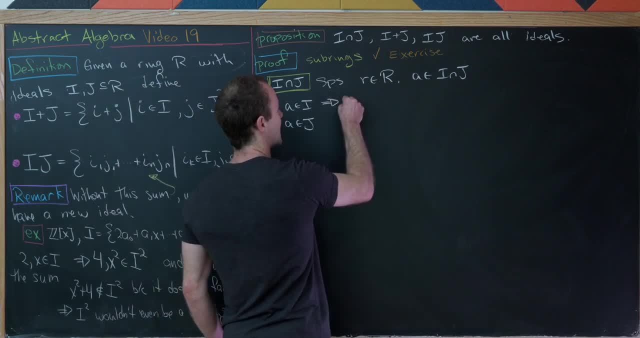 But since A. Is an element of I. We have A R and R A. Are both elements of I. That's because we're assuming I is an ideal. 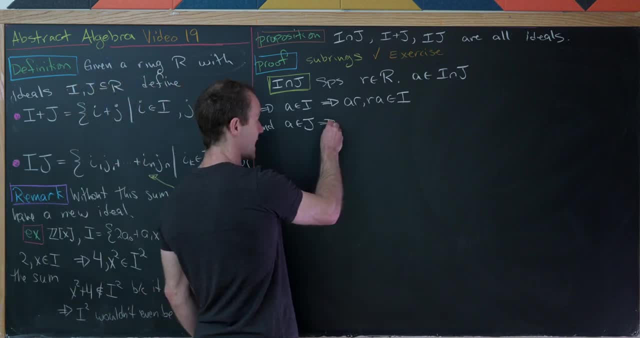 And then since. A is an element of J. 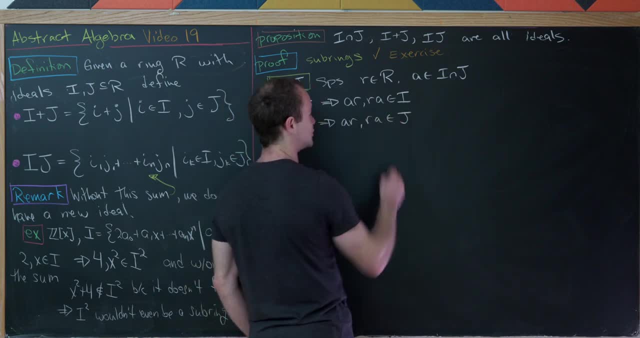 That means that A R and R A. Are both elements of J. 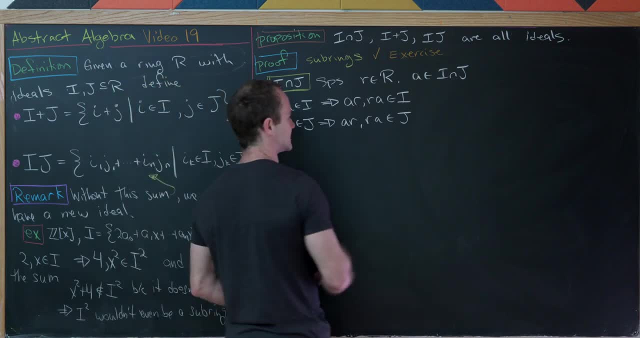 That's again. Because we're assuming that J is an ideal. 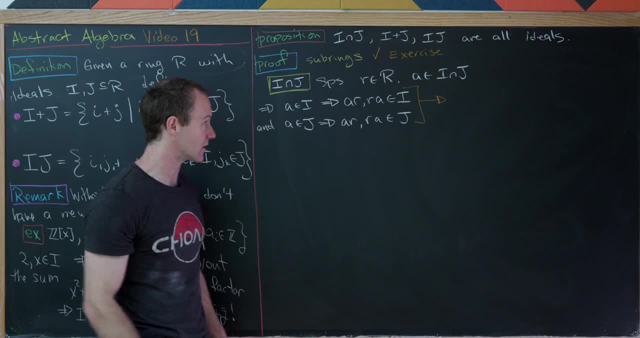 But now. We're putting these two things together. We see that. A R and R A. Are elements of I intersect J. 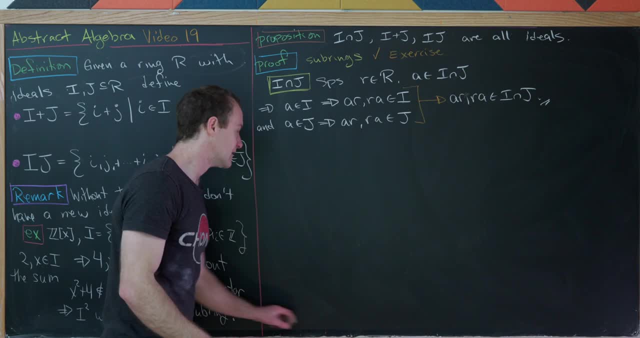 But that's exactly the condition. That we need. 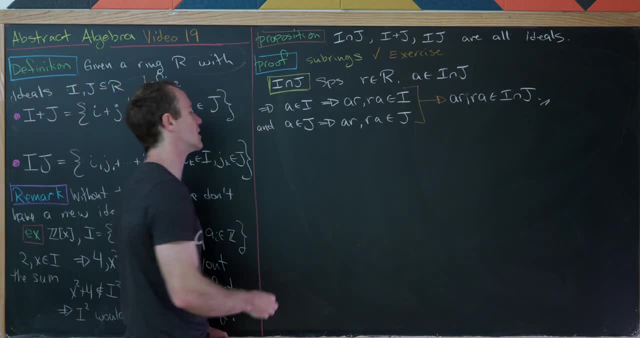 For I intersect J. To be an ideal. So we're good to go there. 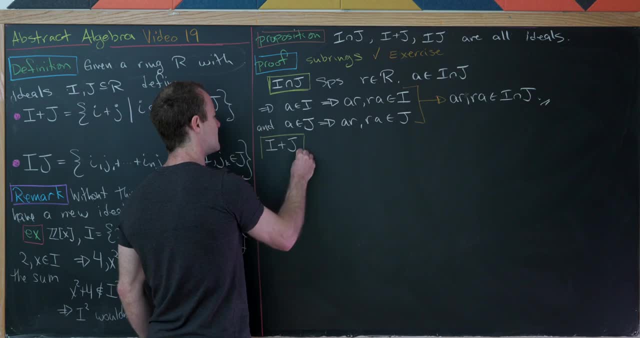 Okay so now let's look at I plus J. The sum. And maybe before we continue on here. I'd like to point out. 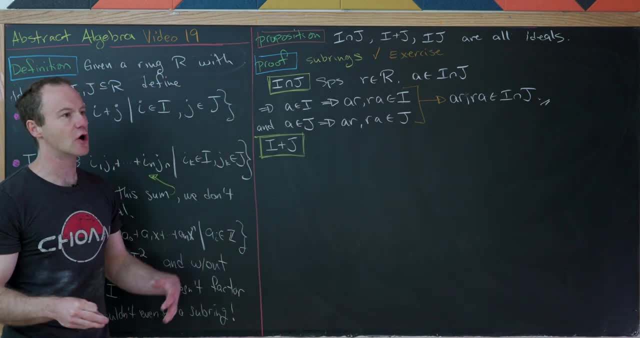 That these types of ideals. Will play an important role. In the isomorphism theorems for rings. Okay so let's do it. 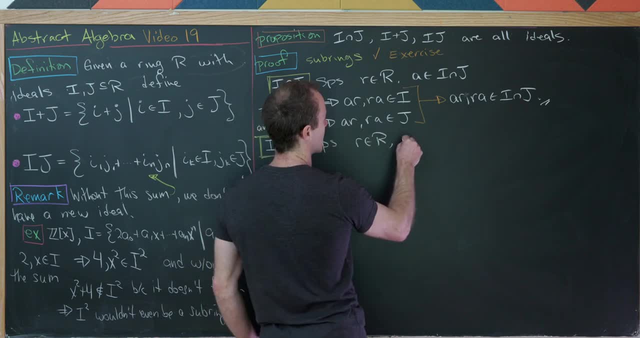 Let's suppose. That R is an element of R. 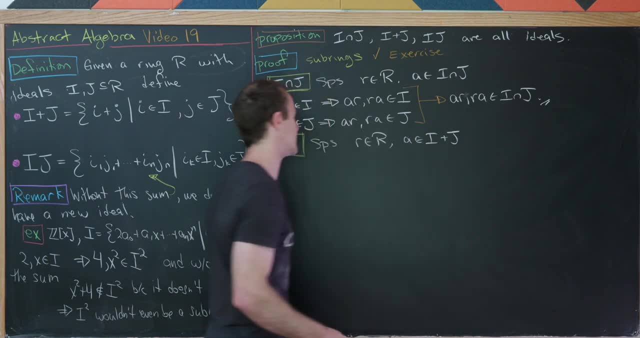 And we have A an element of I. Plus J. But notice that means that. 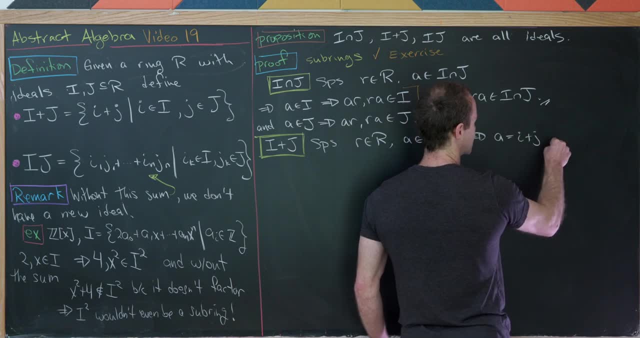 A has a special form. It's little I plus little J. Where little I is I. And little J is in J. 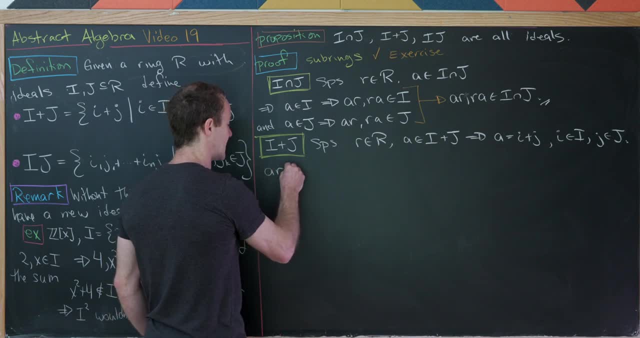 And now we can just let it rip. So let's notice that A times R. Is I plus J. Times R. But now we can do. 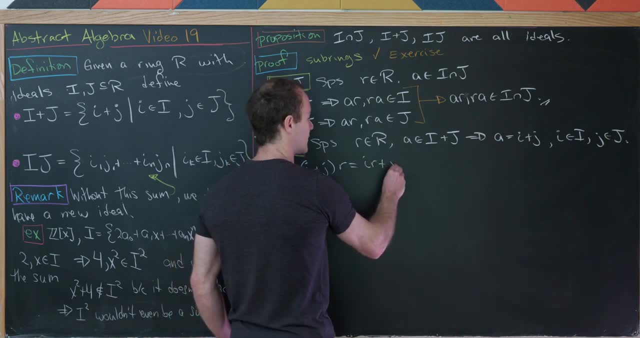 Distribution. To give us I R plus J R. 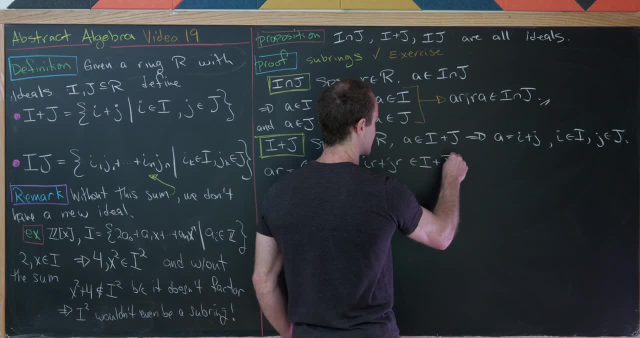 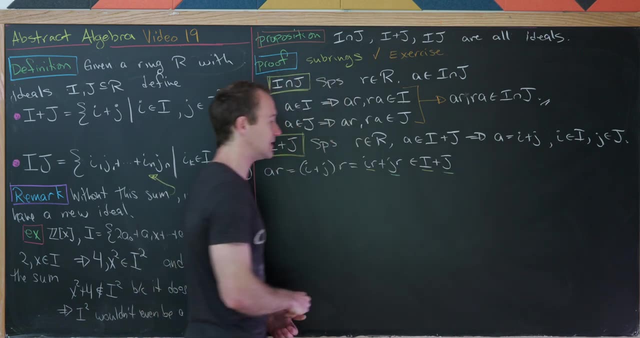 But now notice. That's going to be an I plus J. Because. I R is in I. And J R is in J. Because those are both ideals. Themselves. 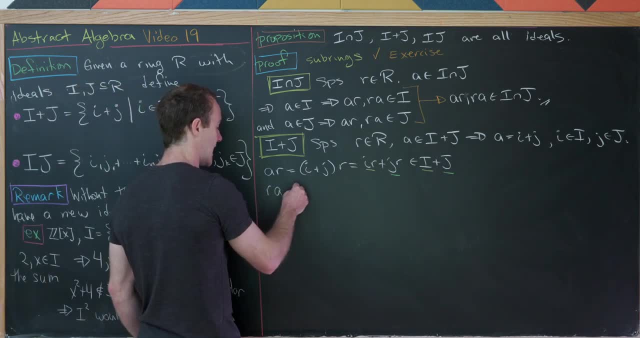 Now we can do the other sided multiplication. R I A. So that will be R times I. Plus J. That's going to be equal to R I. 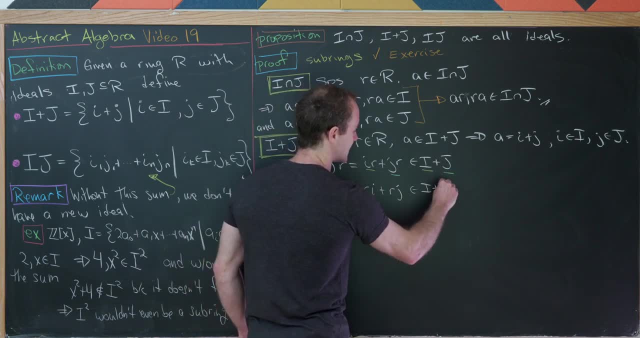 Plus R J. But again. That's going to be an I plus J. For the same reason. 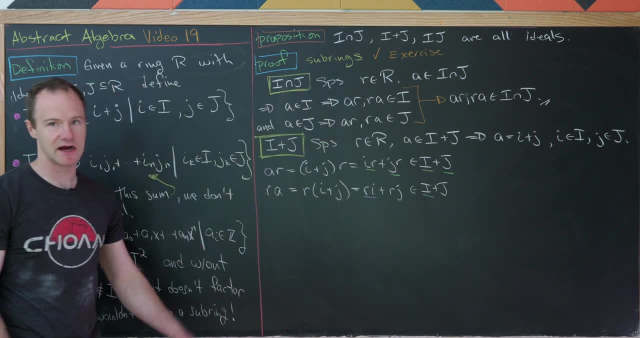 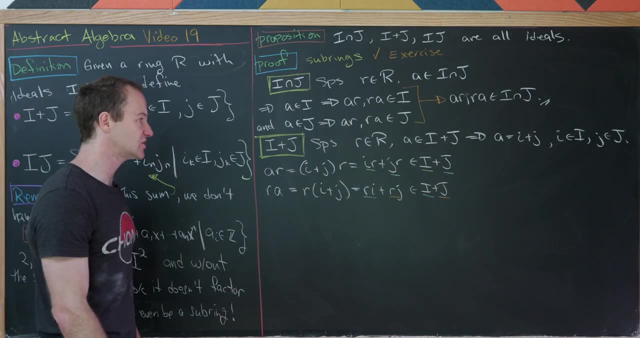 Because R I is in I. Because we have I as an ideal. And R J is in J. Because J is an ideal. So these two conditions. Tell us that. We have an ideal I plus J. And we're good to go. So now let's do our last one. Which is this product. Which is J. 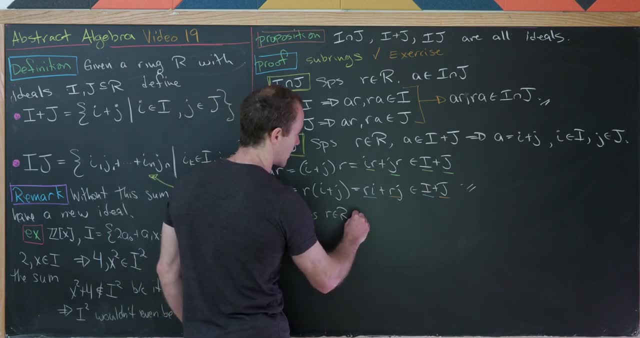 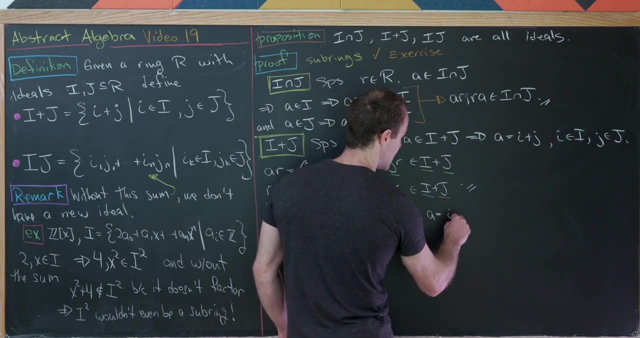 So let's again get started. Let's suppose that R is an element of R. And we have A as an element of I J. But. That means that A has the form. I 1 J 1. Added all the way up to. 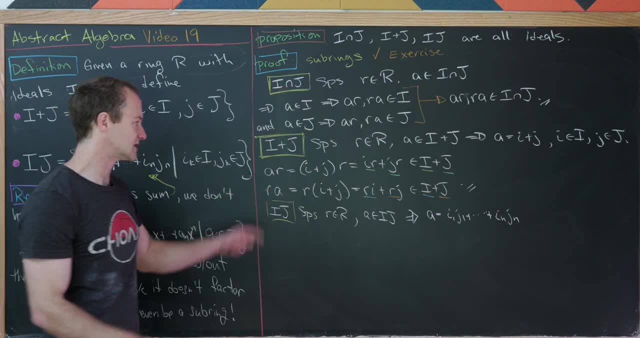 I N J N. Okay good. 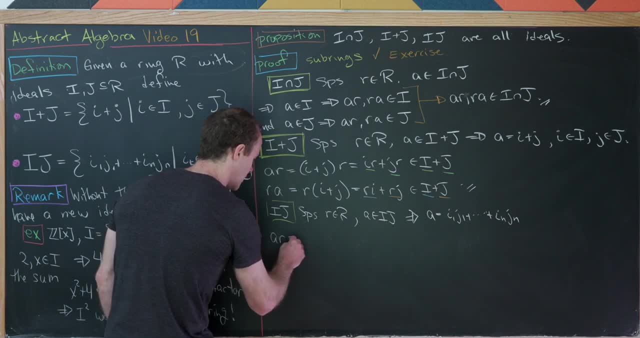 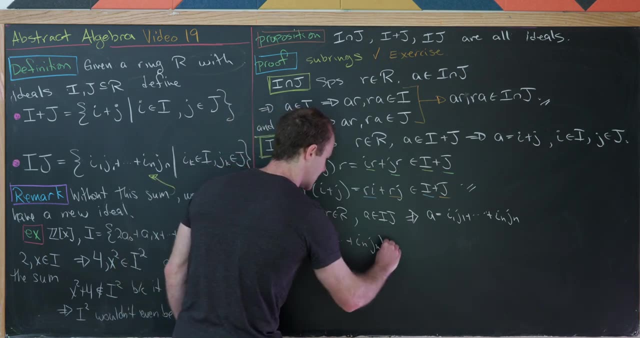 But now let's look at each of these. We have A times R. So that will be I 1 J 1. Plus all the way up to. I N J N. Times R. But now we can do our distribution rule again. And that will leave us with. 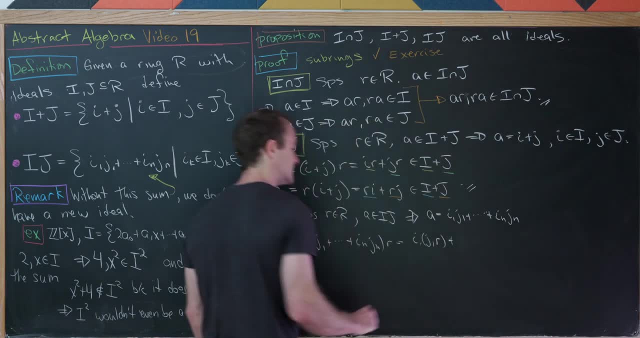 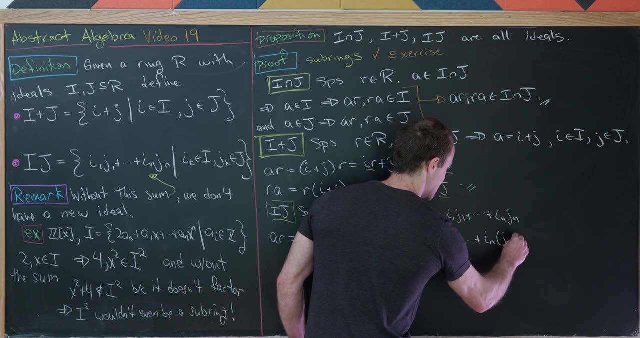 I 1 J 1. Times R. And I'm going to associate it like that. Plus all the way up to. I N. And then J N times R. But I'm going to argue. That this is inside of I J. 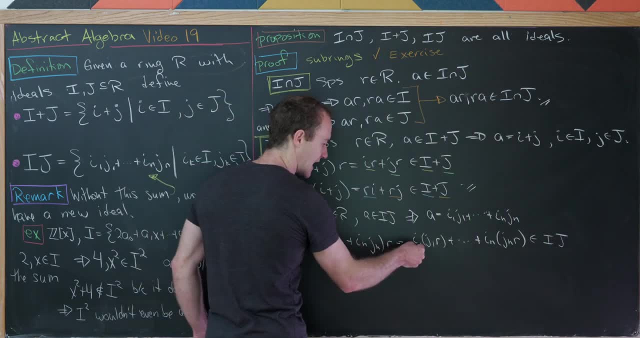 And let's color code the argument. That's because. 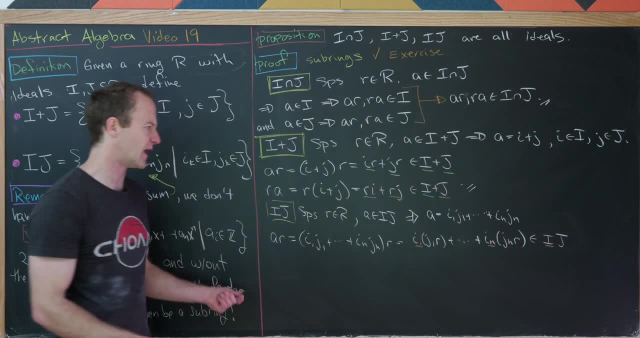 I 1 up to I N. Are all in I. Sort of our definition up here. I didn't write that. 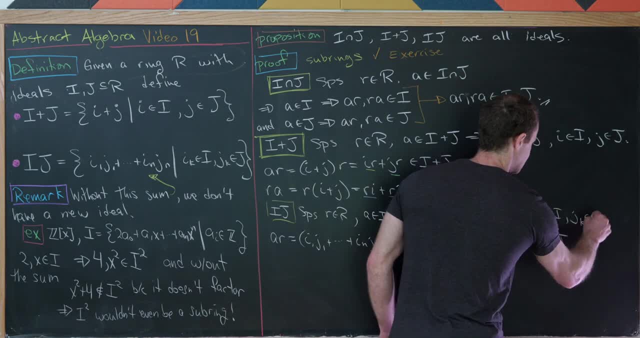 But that's because all of these I K's are in I. And all of these J K's are in J. Like our definition over here. 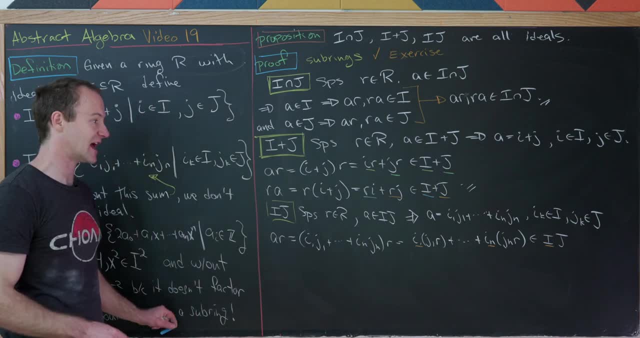 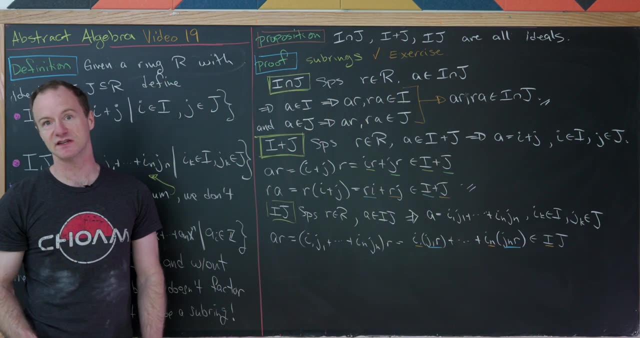 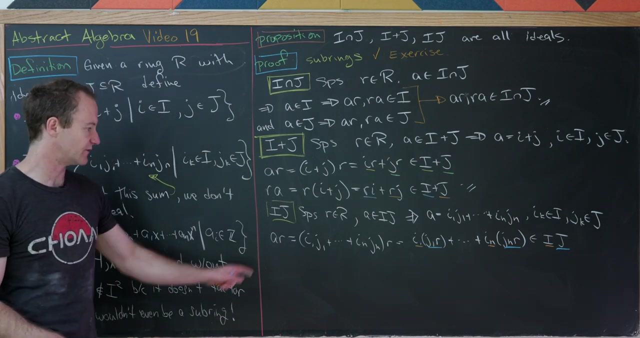 But now. We can use the fact that. J is an ideal. And since J is an ideal. All of these things right multiplied by R. Into the J term. Are inside of J. So that's because J is an ideal. Okay so we've got. 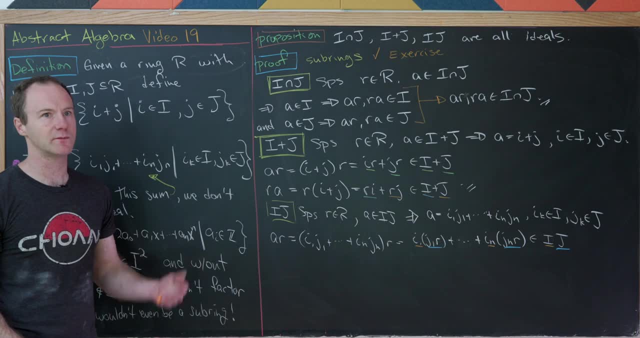 A times R is an I J. So that's one portion. 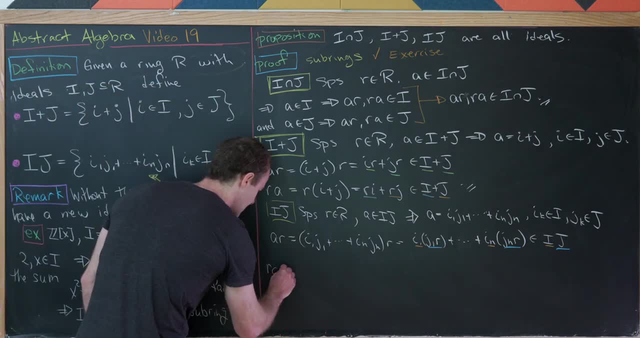 Of the ideal condition we need. And now let's look at R times A. 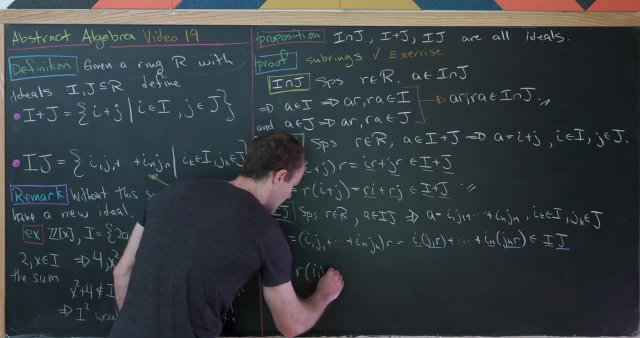 So that'll be R times. I 1 J 1. Added all the way up to I N. J N. But that'll be let's see. 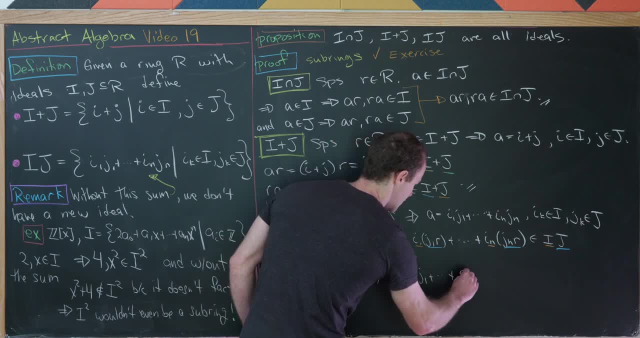 R I 1 J 1. Added all the way up to R. I N J N. But I'll argue. 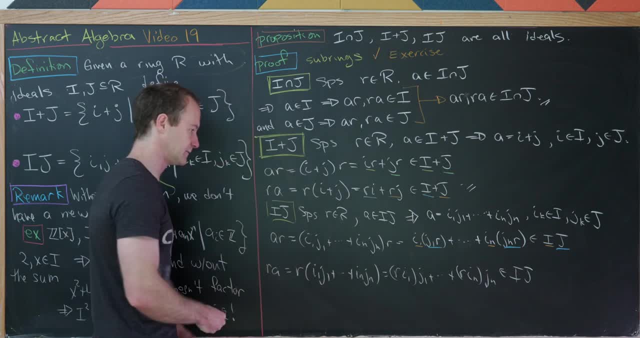 That that's in I J. Very very similarly. So notice that all of the J. 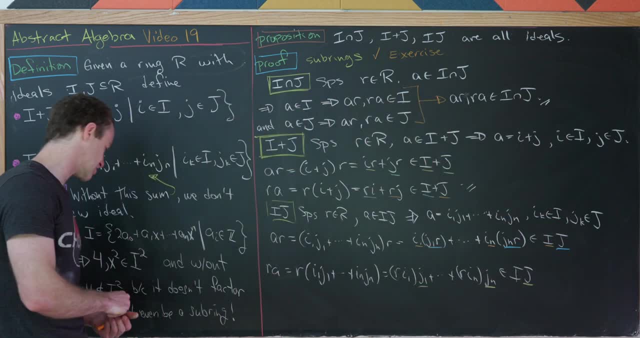 Are inside of J. By you know our original assumption. 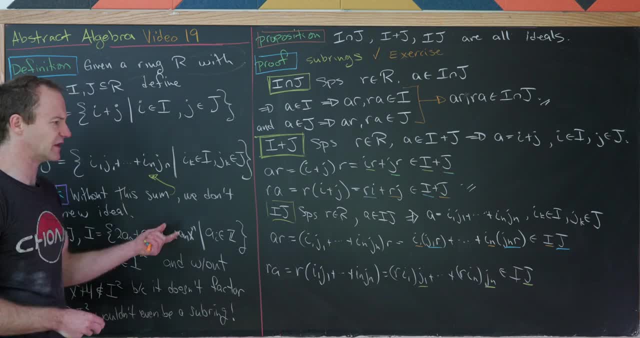 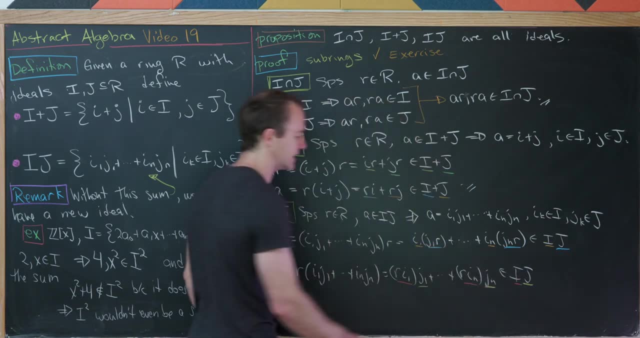 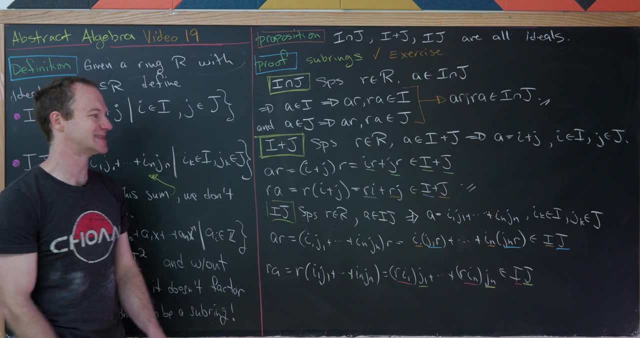 And then. By this property that we had. Before for ideals. We know that R I 1. Is an element of I. All the way up to R I N. Is also an element of I. Because I itself is an ideal. So we've got A R is an I J. 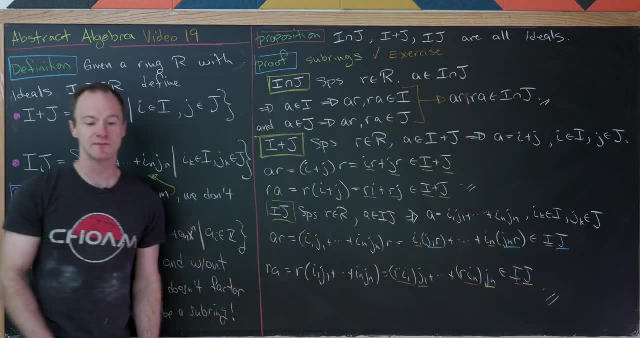 And R A is an I J. But that's exactly the condition. We need for I J to be an ideal. So in fact we do have an ideal. 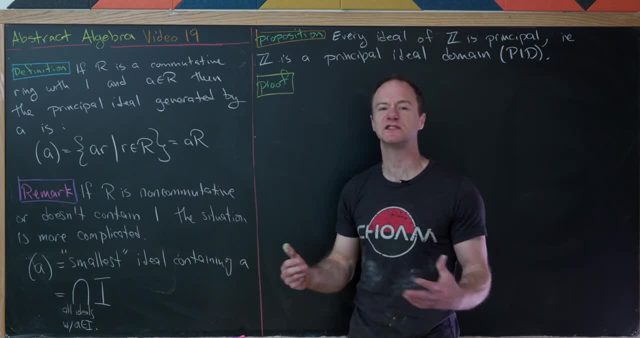 In this video off with a new type of. Ideal or a really special. Type of ideal that shows up a lot. 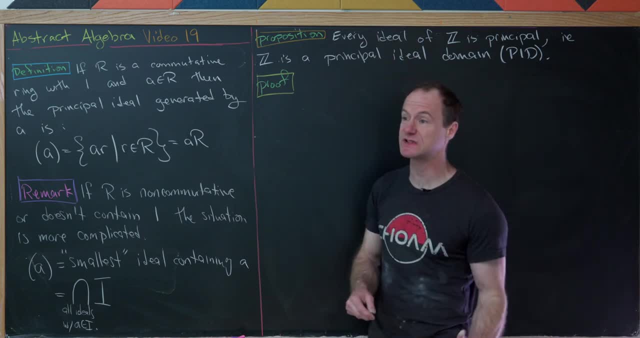 In the examples that we'll see. And that's something called a principle. 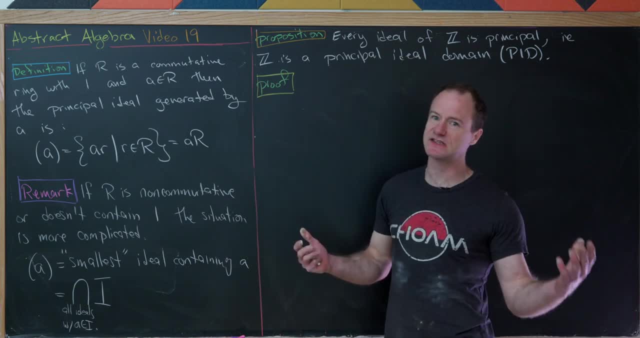 Ideal so we'll. Mostly do this in the setting of. Commutative rings with identity. 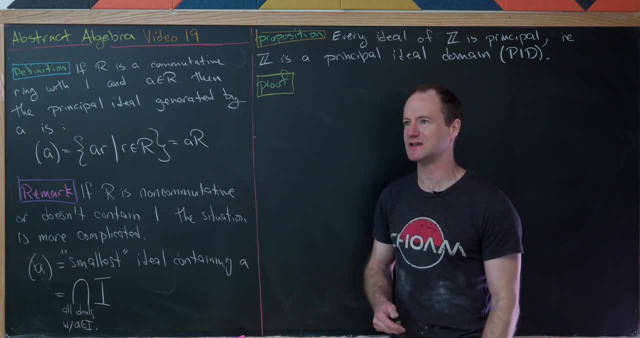 But I will point out. A remark of what happens if you're. 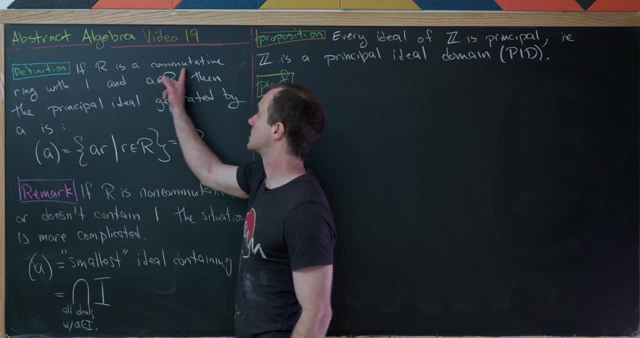 Outside of that setting. So if R is a commutative. Ring with one. And A is an element of R. 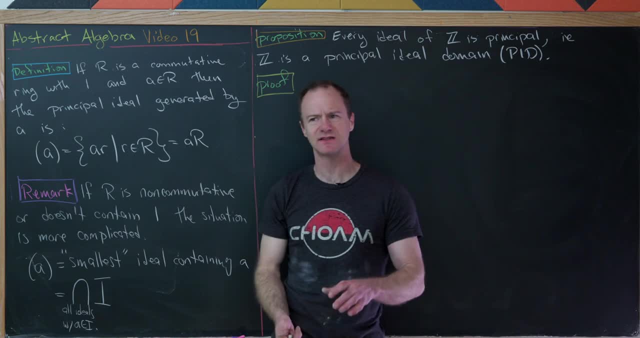 Then the principle ideal. Generated by A is. Put very simply. All multiples of A. 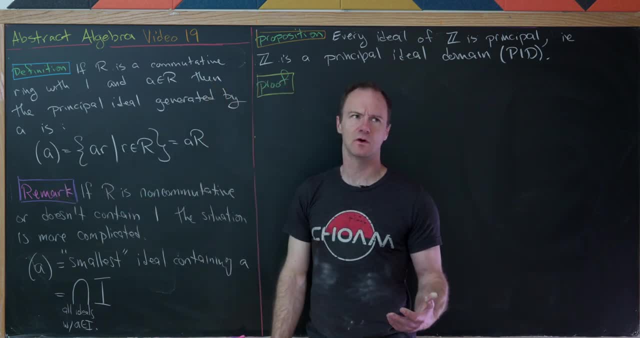 So you write this as these parentheses. With the A. Or sometimes they're like. Square brackets with the A. Or angle brackets with the A I should say. 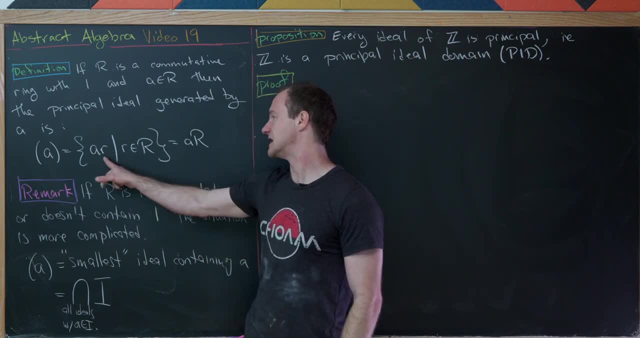 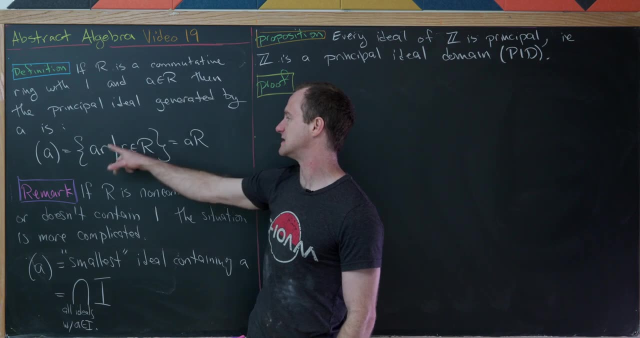 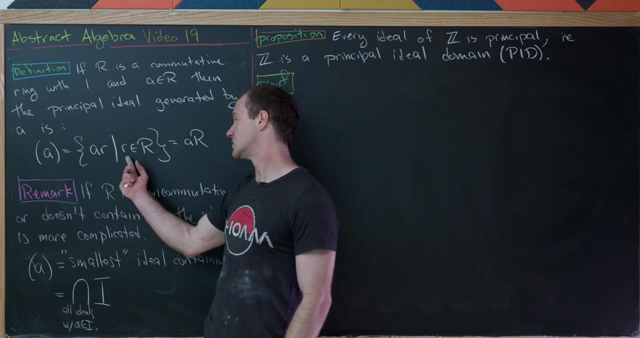 That's going to be like I said. All R multiples of A. So we've got A times R. As R runs through everything from the ring. Here we're assuming commutativity. So that means A times R is R times A. So we don't have to worry about that. And then also we're assuming. We have a one. 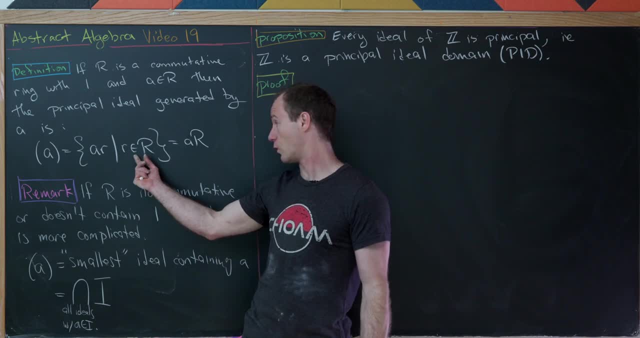 So we will eventually choose. The element one here. Which means A will be inside of this. 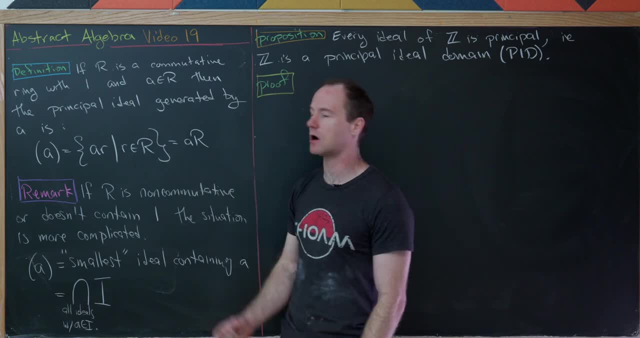 Sometimes this is. Written as little a R. Just for interest. 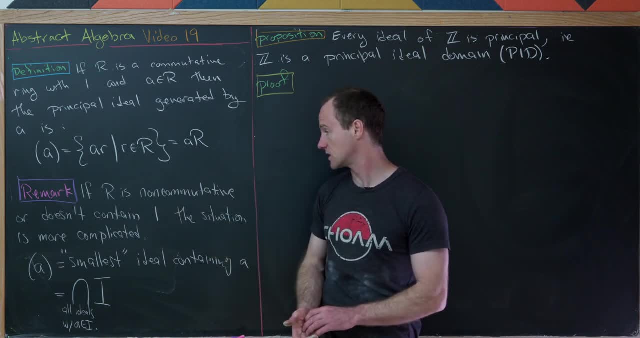 And then here's our remark. If R is non commutative. Or it does not contain one. 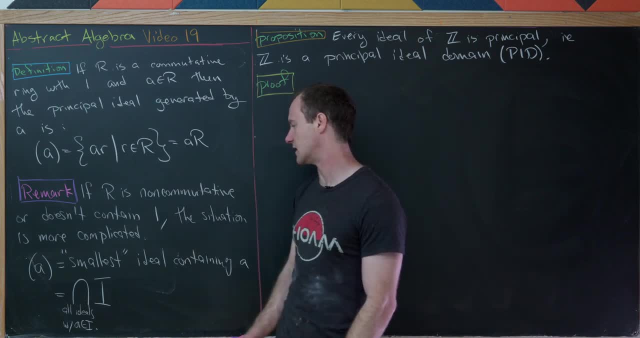 The situation is. A little bit more complicated. 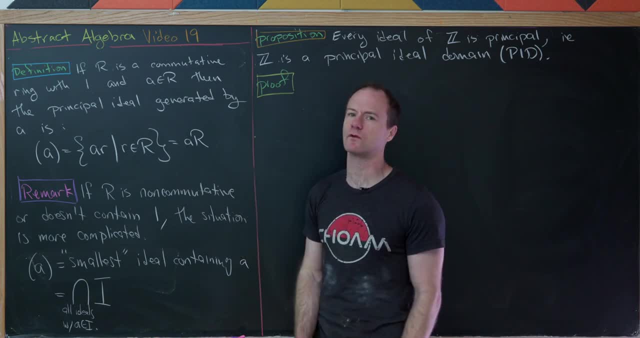 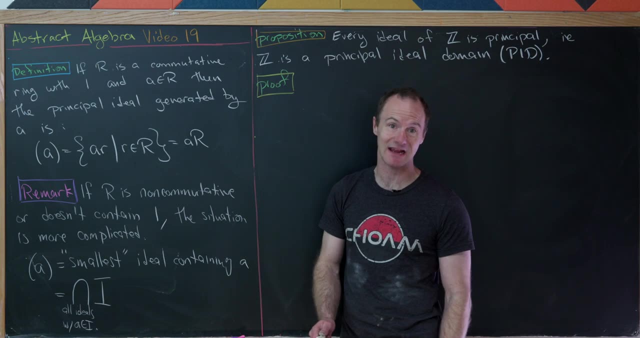 And in this case. Maybe most universal way. Of defining this. Principle ideal. Is to be the smallest ideal. Containing the element A. But what does that mean? Well one way of getting at it. 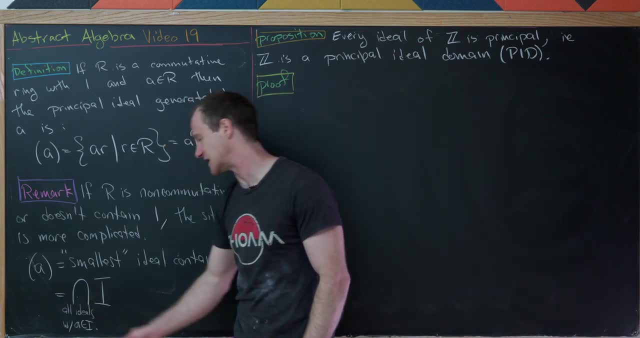 Is to intersect. All ideals that contain A. 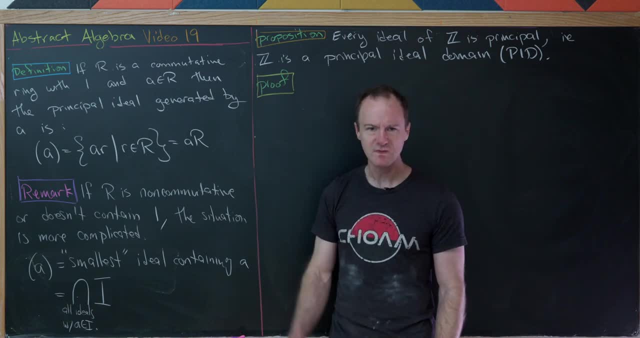 And that will give you. The smallest one. 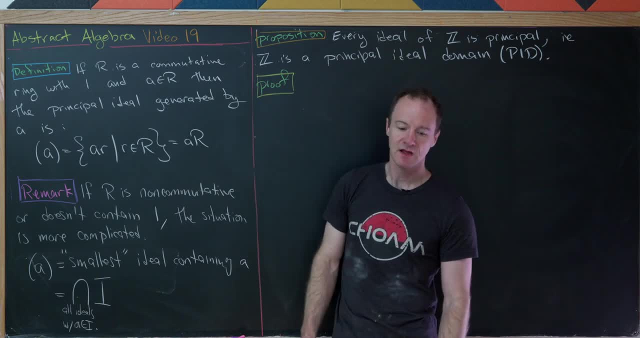 But like I said. We'll mostly be dealing with this up here. 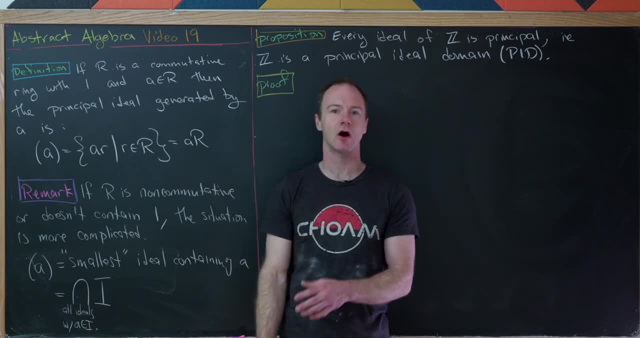 Now it's pretty simple. To show that principle ideals. Interact ideals. 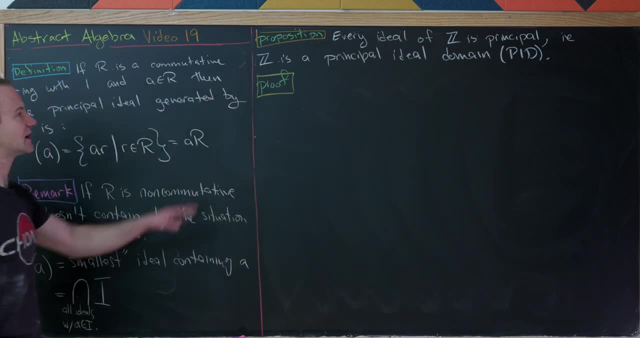 So I'll leave that to you. As an exercise. 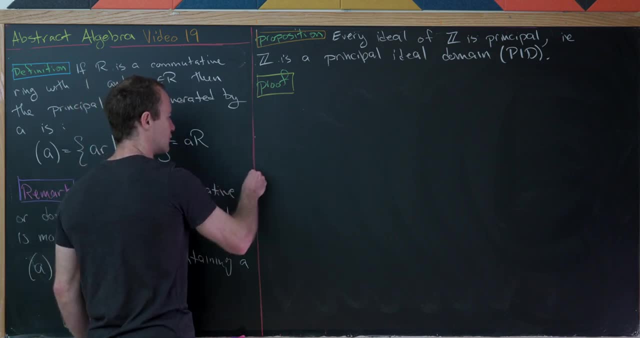 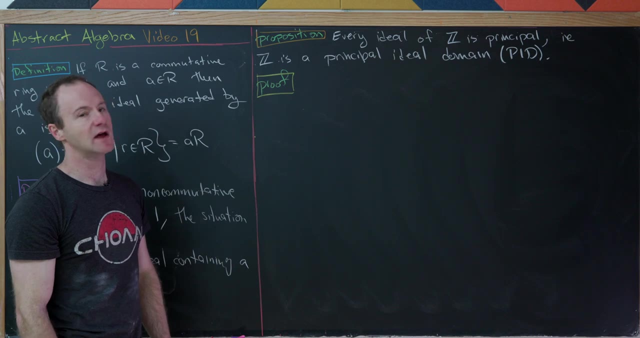 So now let's prove the following proposition. As maybe our last thing for the day. Before I leave you with some warm ups. And that is. That every ideal of Z. Is principle. 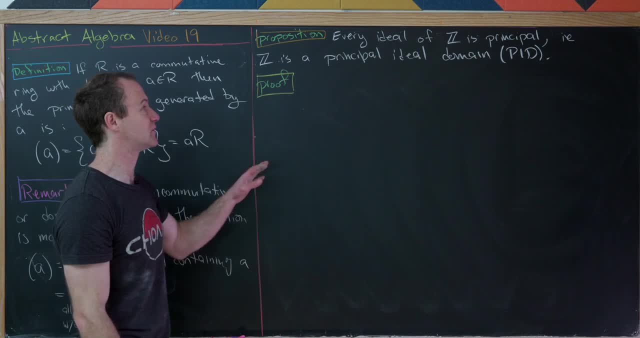 And the rings that have this. Characteristic are called. Principle ideal domains. 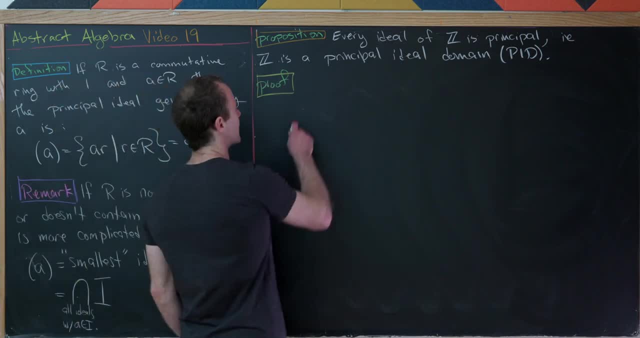 So what we're showing here. Is PID. 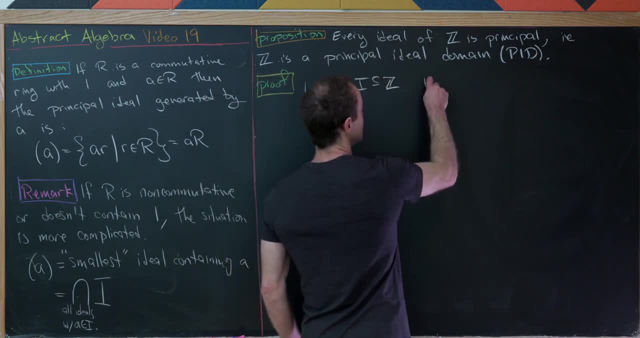 So how can we do this? Well let's start with an ideal. 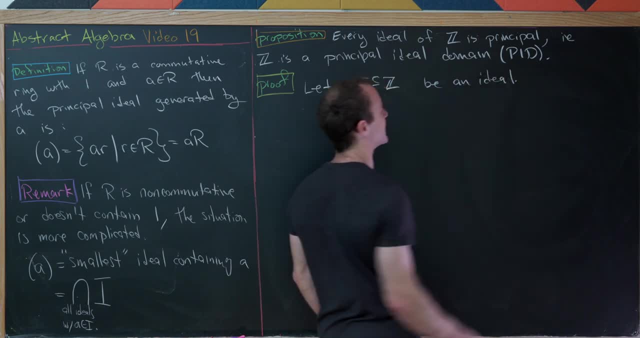 So let's let I. A subset of Z. Be an ideal. So that means it's a subring. 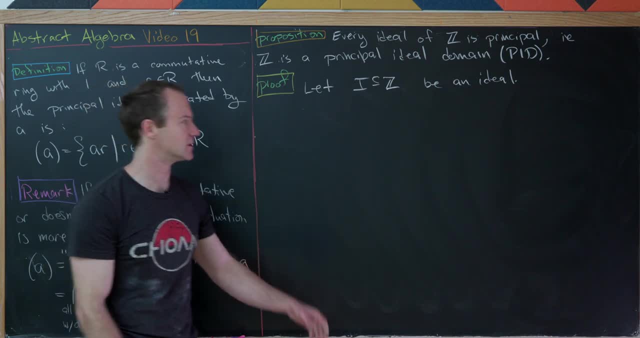 With that absorption property. And now let's notice that. Since I is an ideal. Let's maybe say it's non-trivial. So let's say that I. 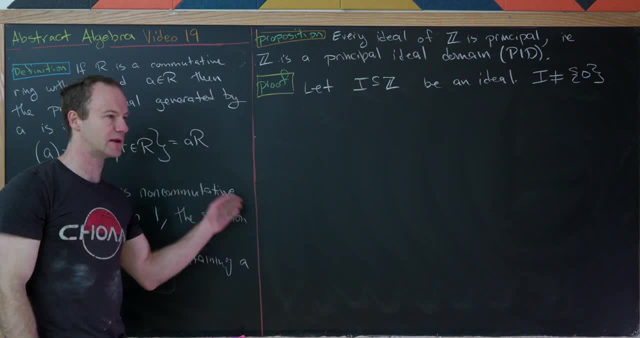 Is not just. The element zero. But it does contain. Positive as well as negative elements. 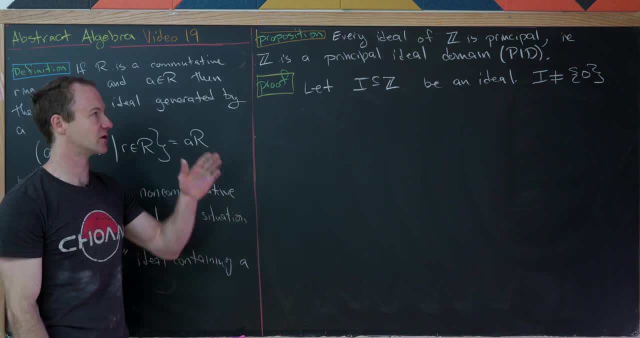 That's because anything. Will come with it's additive inverse. Given that it is a subring. 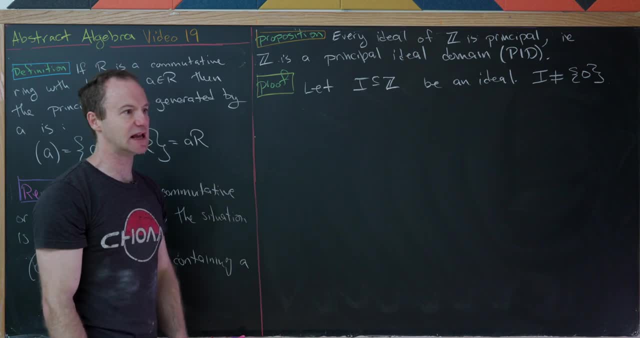 So since it has. Positive elements. 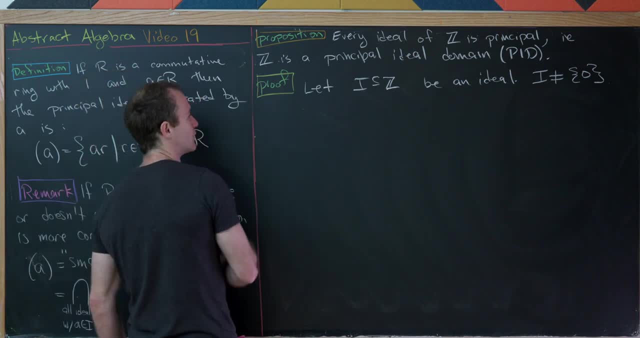 It intersects non-trivially. With the natural numbers. And that's what we want to use here. So let's set this number N. Equal to the minimum. 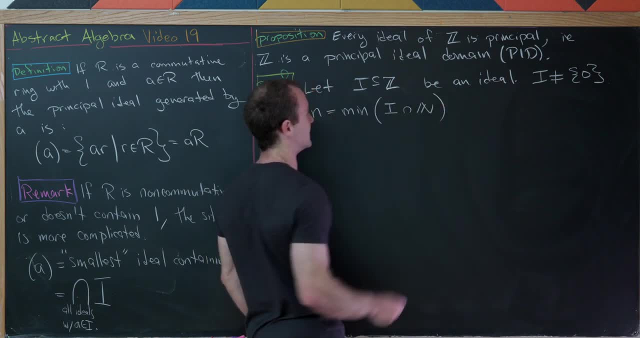 Of the intersection. Of N with the natural numbers. 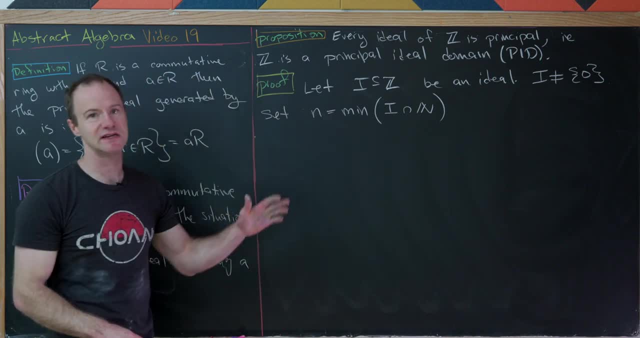 So like I said. That'll be a non-empty subset. 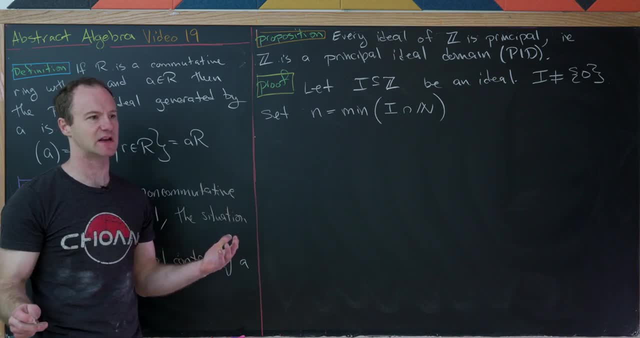 Of the natural numbers. And we know every non-empty subset. 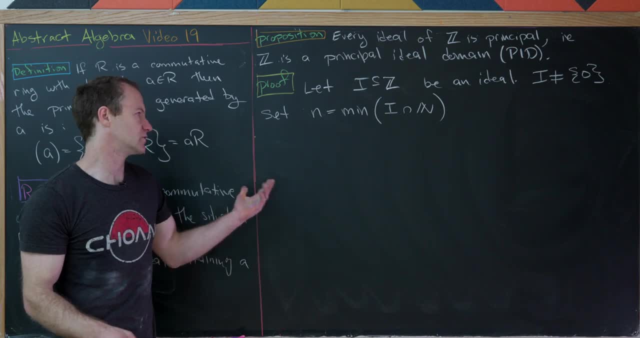 Of the natural numbers. Has a minimal element. 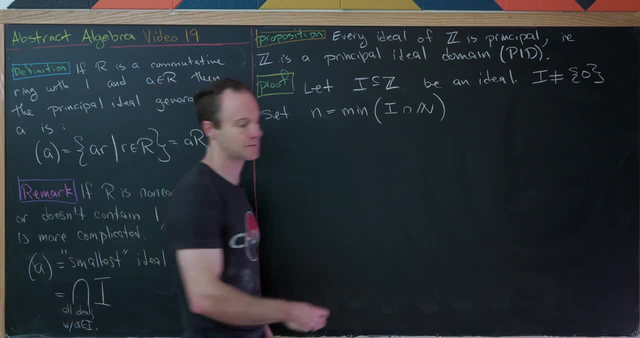 And we're just taking that minimal element. That's by the well ordering principle. Great. 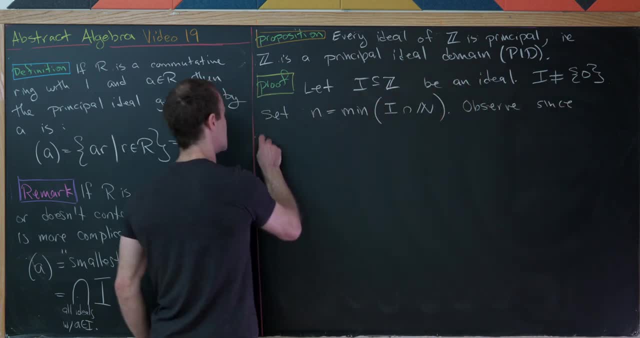 And now let's observe. That since. 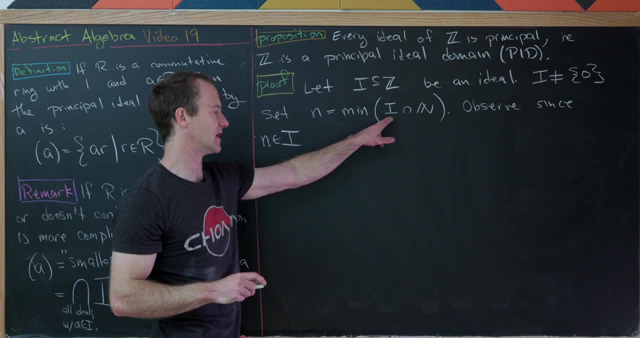 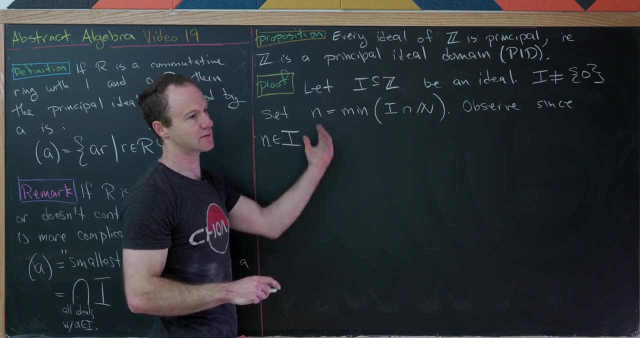 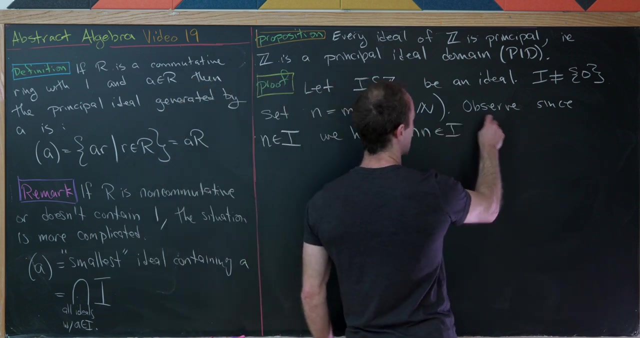 N is an element of I. Well it's most definitely an element of I. Because we're setting it equal to the minimum here. And like I said. By the well ordering principle. If natural numbers achieve their minimum. We have. M times N. Is N I. 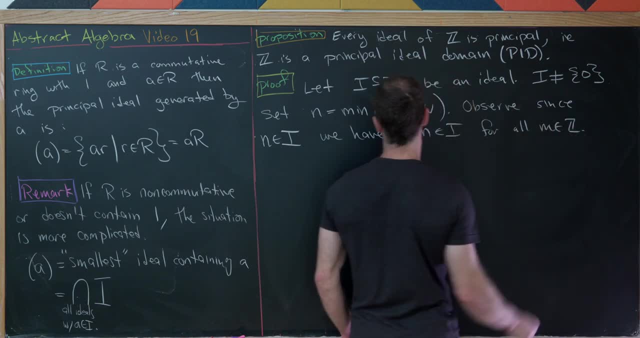 For all. Integers M. 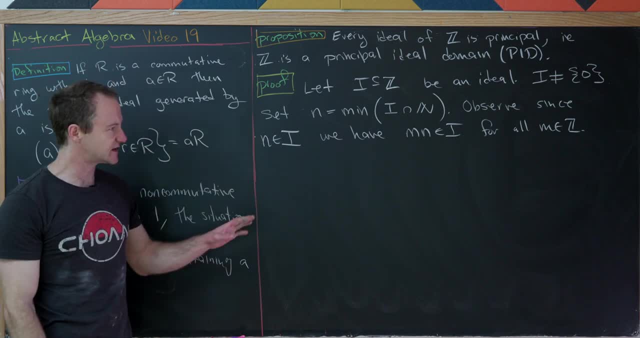 That's because I is assumed. To be an ideal. So since it's assumed to be an ideal. 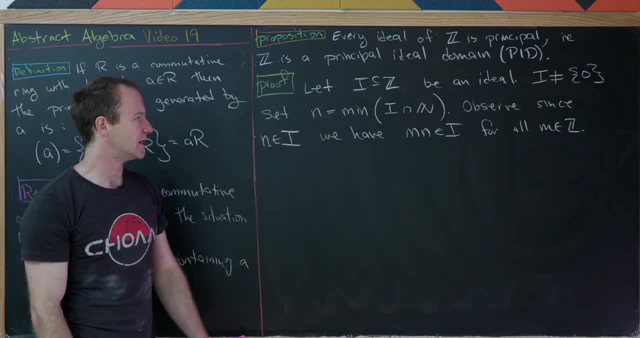 It has this absorption property. Like I talked about. But notice that everything of this form. Well that's creating everything. 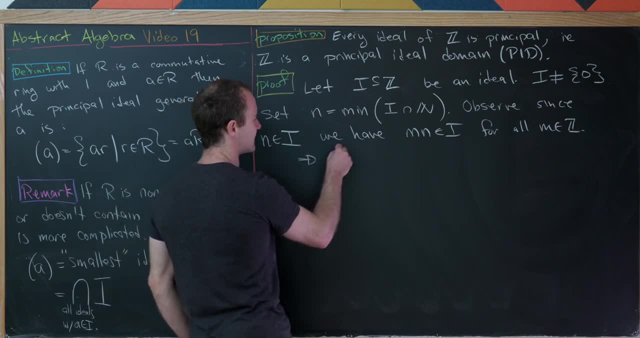 In the principle ideal. So that means that. 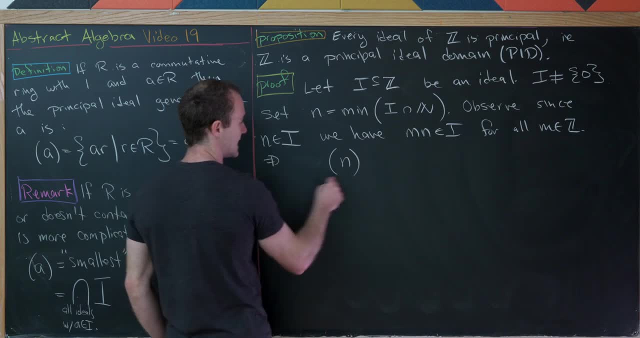 In fact the principle ideal. Generated by N. Is a substructure. A subset of. The whole ideal. 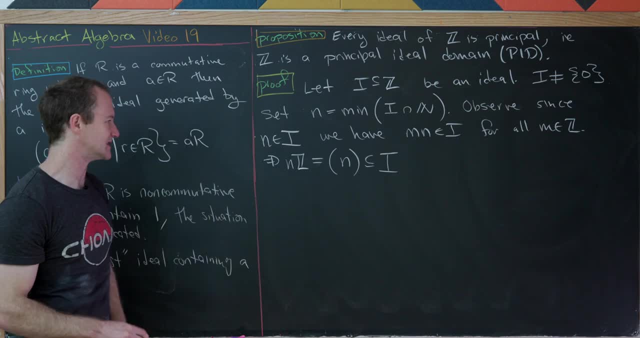 And I'd just like to point out that. We'll generally write this principle ideal. 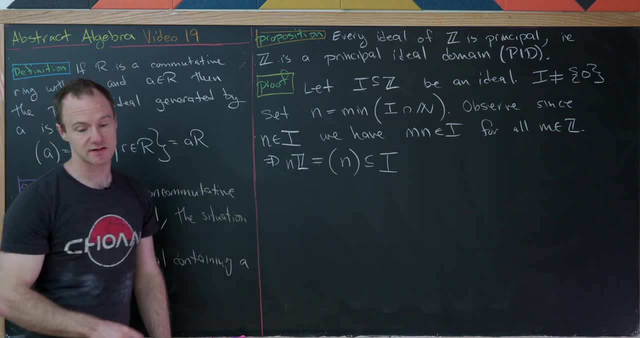 As NZ. Although sometimes it's written as N. So it's no big deal either way. 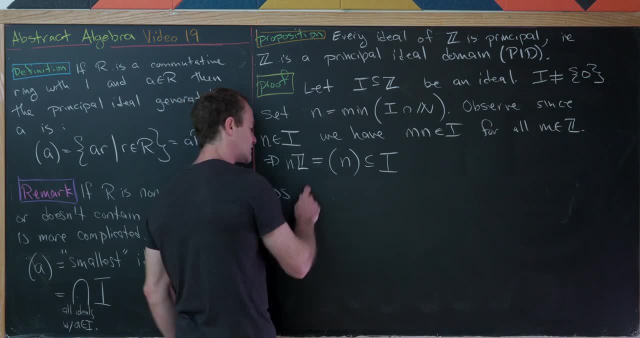 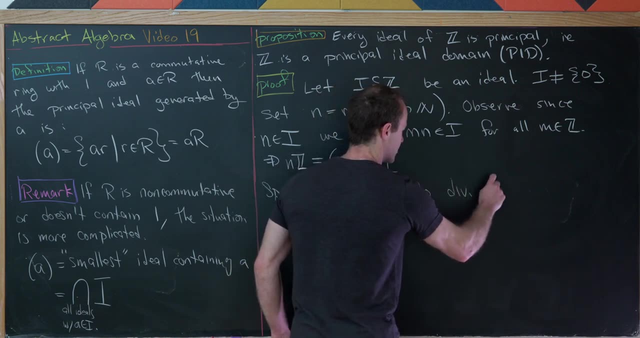 Now we'd like to show this subset containment. The other way. Okay so let's suppose that A. Is an element of I. And. Is an algorithm. 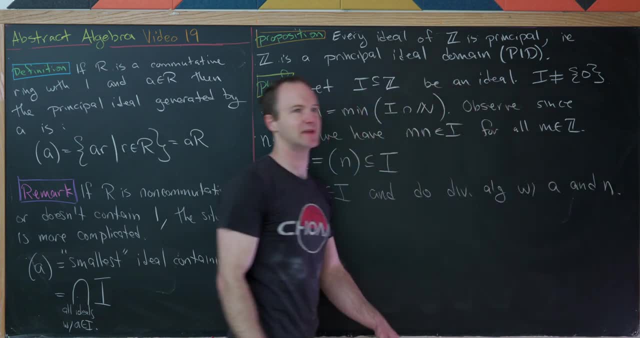 With A. And N. 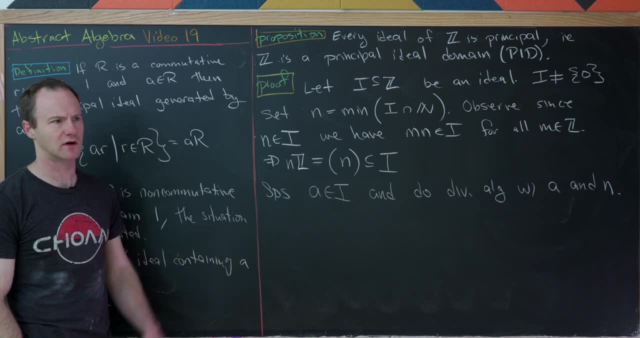 So as is somewhat common. It comes down to division with remainder. Something you learned many many years ago. 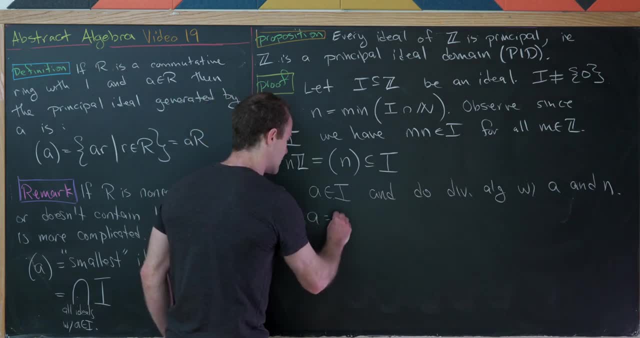 Okay so what is that going to give us. That'll give us. A equals N times Q. Plus R. 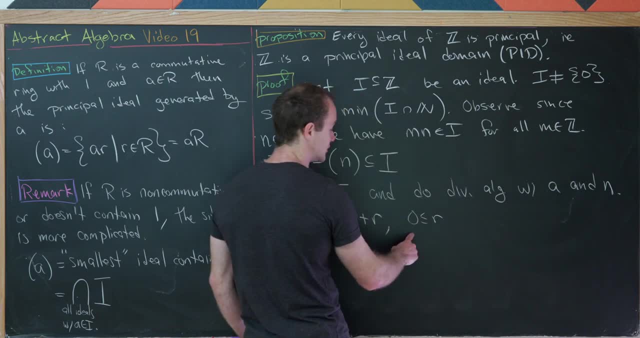 Where Q is an integer. R is also an integer. 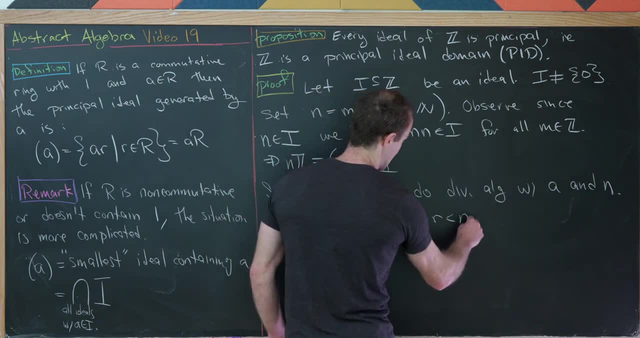 But R is between N. Sorry between 0 and N. It's allowed to include 0. But not N. 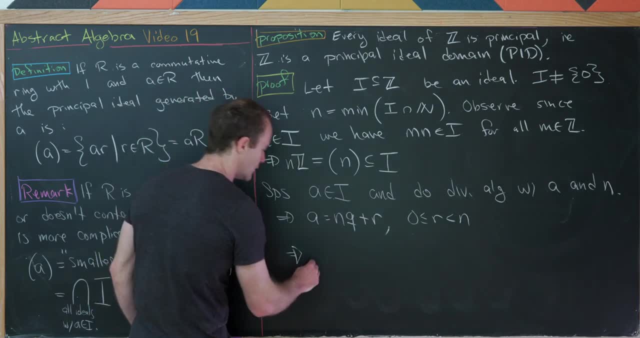 That's by the division algorithm. So now let's rewrite some things. We can write R is equal to. 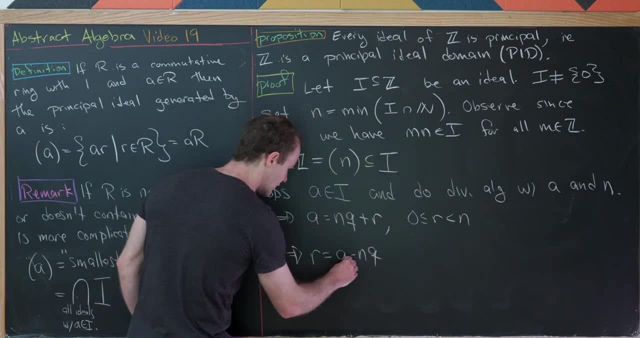 A minus N Q. And notice we took. A to be an element. 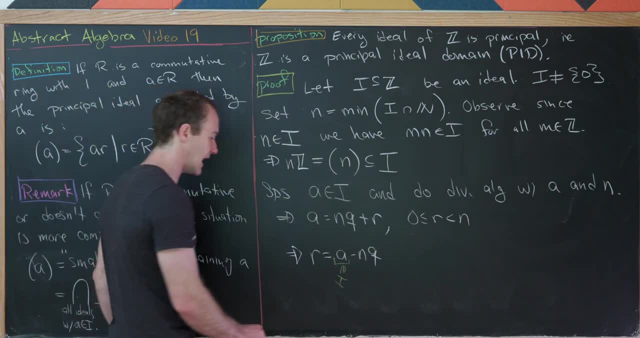 Of I. That was our assumption right here. 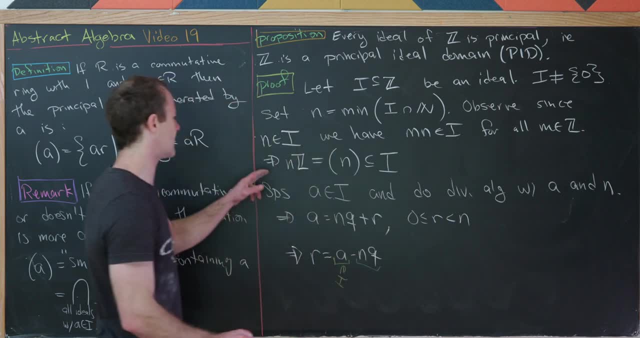 And then since. N is an element of I. As well. We know any multiple of N. 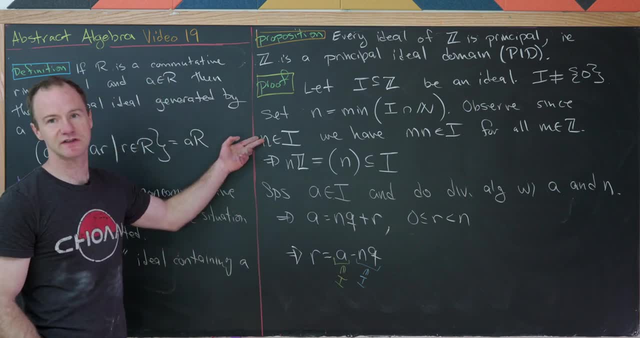 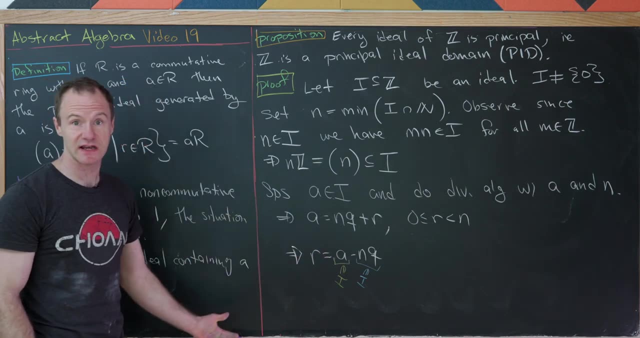 Is also an element of I. Because it's an ideal. Same argument we had here. But then since I is a subring. The difference of two. Elements of the ideal. Is an element of the ideal. So we've got this is an element of the ideal. But look there are two possibilities. 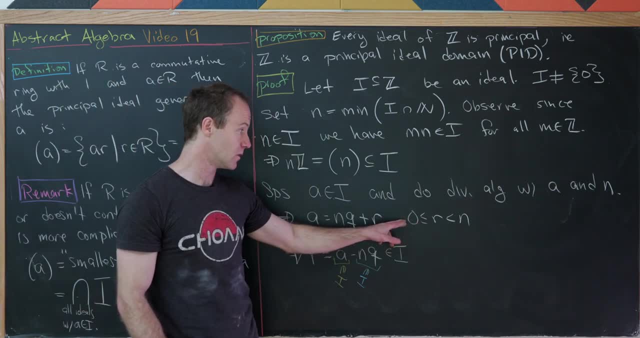 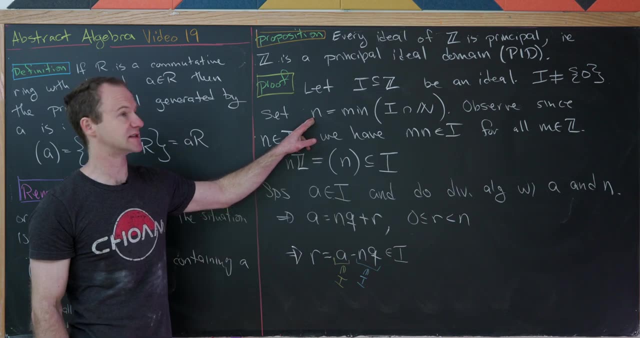 R could either. Be equal to 0. Or it could be. Smaller than. The smallest possible. Positive element of I. But it can obviously not be. Smaller than the smallest positive. Element of I. Because that would be a contradiction. 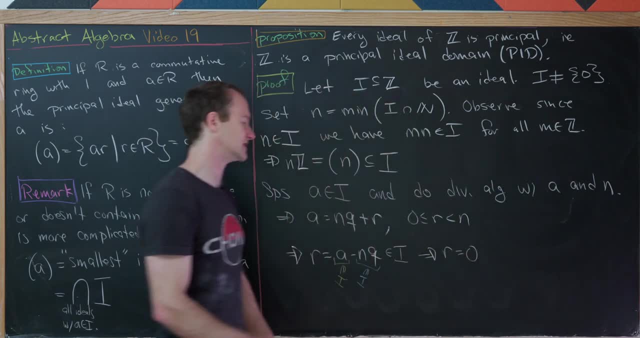 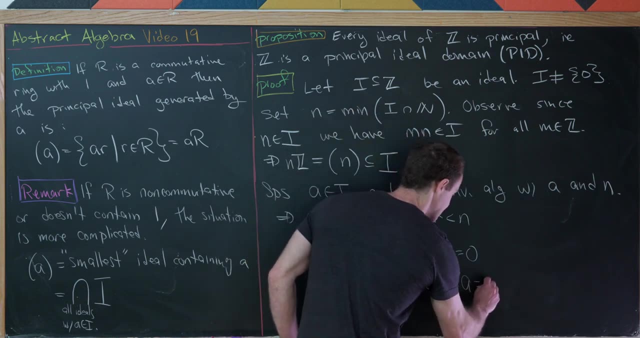 So that means by those words. That I just said that R equals 0. But now. Looping that back. Into this equation right here. We have A is equal to N Q. Which is. An element of the principle ideal. 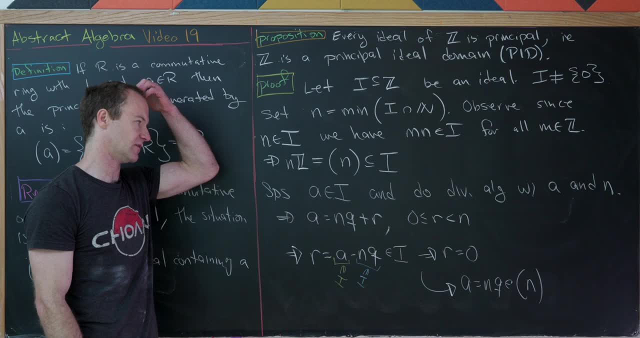 Generated by N by the definition. Of the structure of the principle element. Or principle ideal generated by N. So what does this tell us. 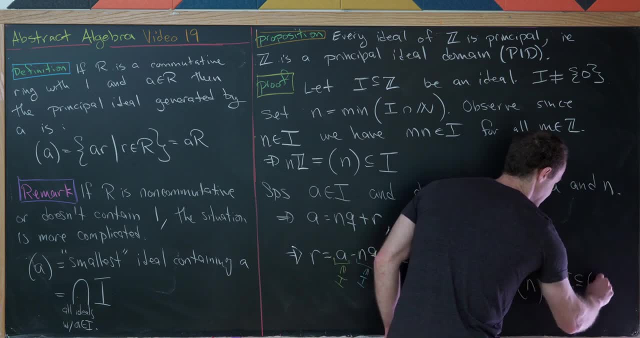 This tells us that I. Is the subset of the principle ideal. Generated by N. But that means we've got the subset. Relationship going both ways. 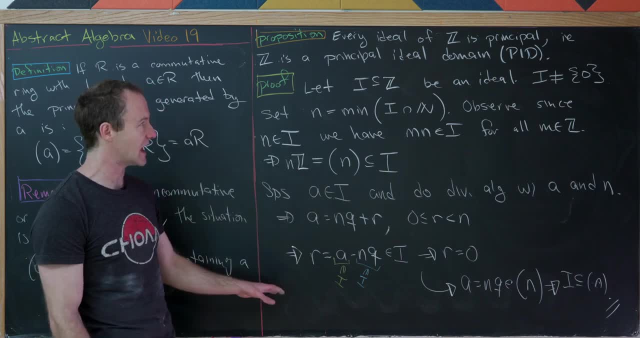 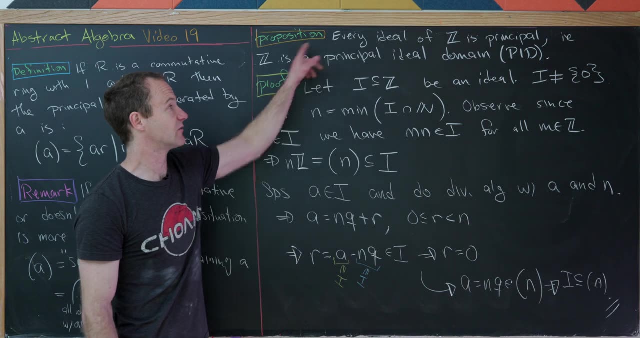 Which means that the ideal is really. Just this principle ideal generated by N. Meaning that. Since we started with an arbitrary ideal. Ended with a principle ideal. Every ideal of Z. Must be principle. 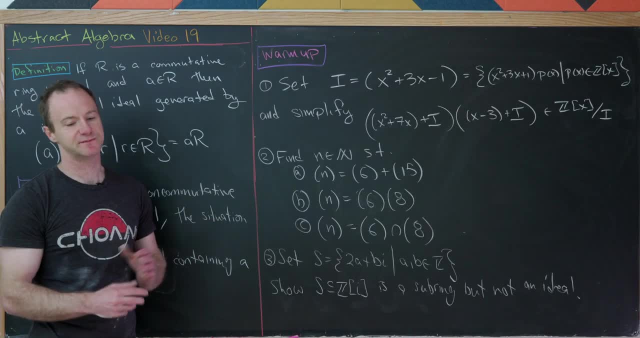 Okay now I'm going to leave you with some warm ups. Here are three nice warm up exercises. 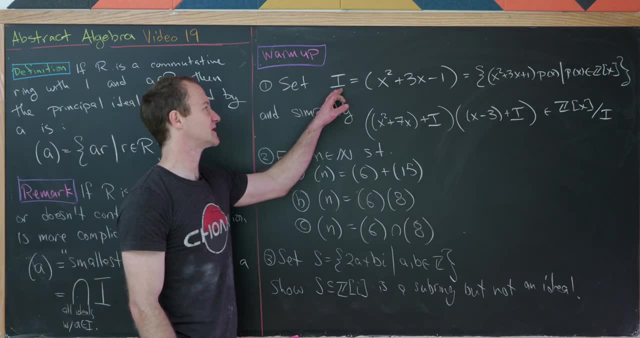 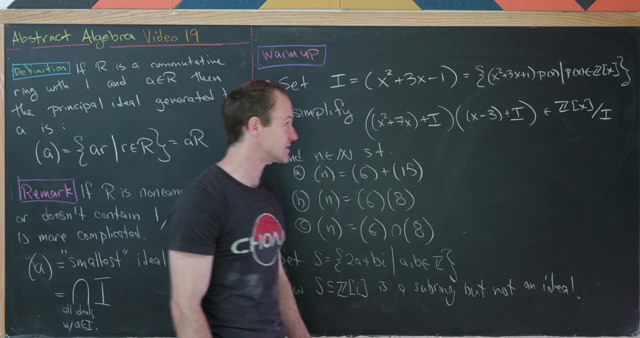 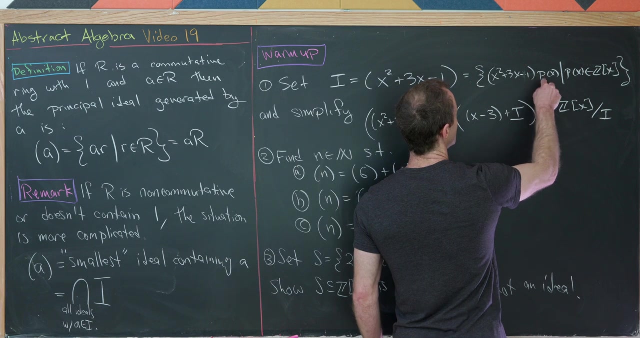 Based off of what we've seen. So the first. Is the principle ideal. Generated by the quadratic polynomial. X squared plus three X minus one. So just as a reminder. That's going to be everything of the form. X squared plus three X. Minus one. 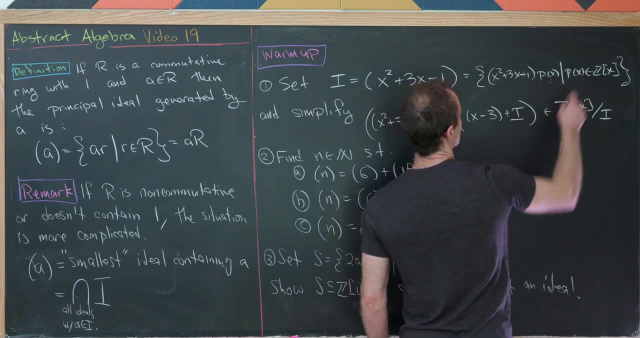 Times another polynomial. P of X. Where P of X is in Z adjoin X. 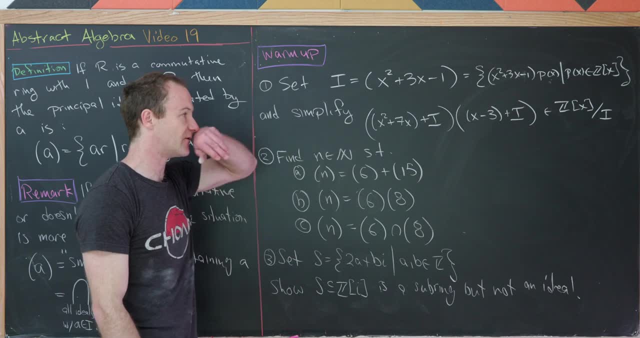 That's our parent ring here. And then let's simplify the following. 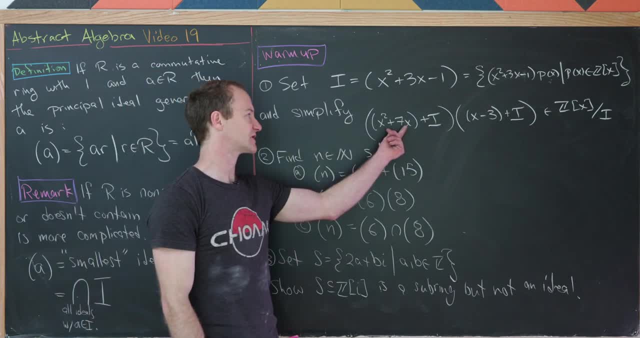 Product inside the quotient ring. So we've got. X squared plus seven X plus I. And then X minus three plus I. 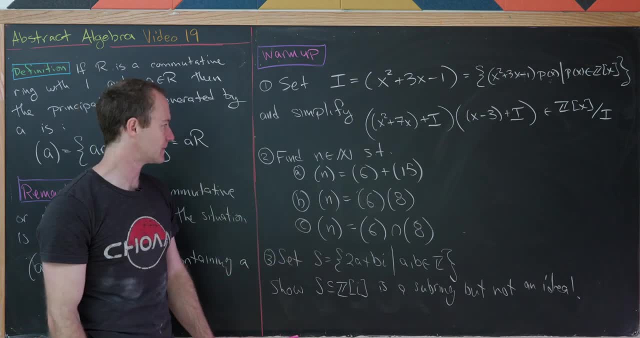 So do that product. And then simplify. 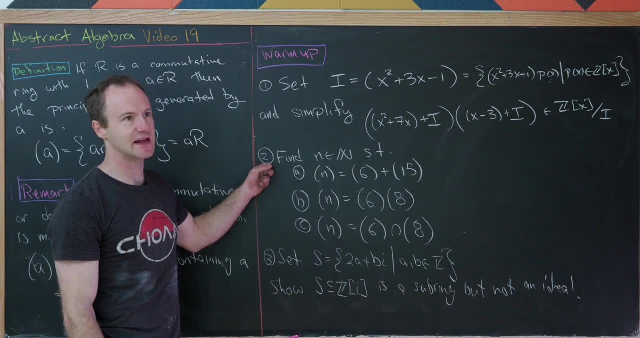 Then for the second one. We've got kind of a three part thing. 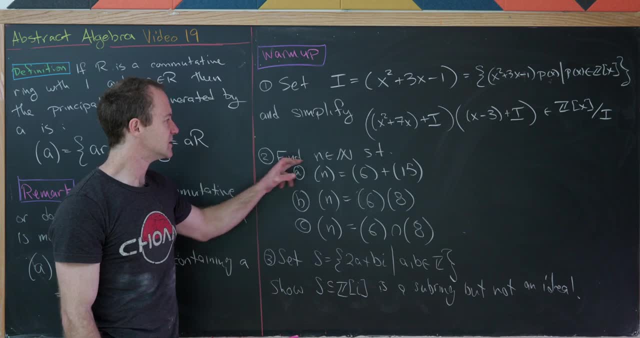 And that is using the fact that. All of the ideals in Z are principle. So let's find a natural number N. Such that. N is equal to the sum of the ideals. 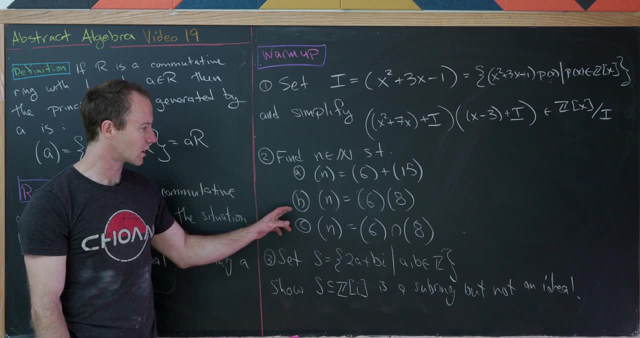 Generated by six and fifteen. Or. 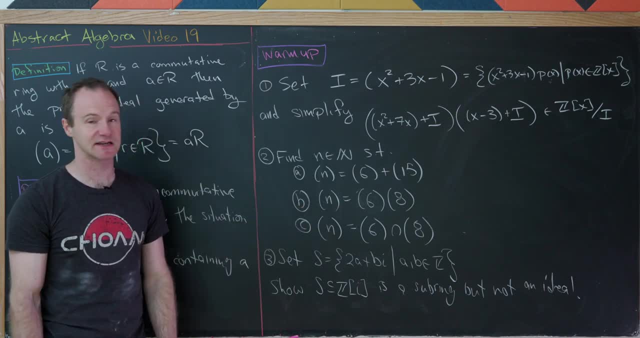 The second one is. N is the product of the ideals. 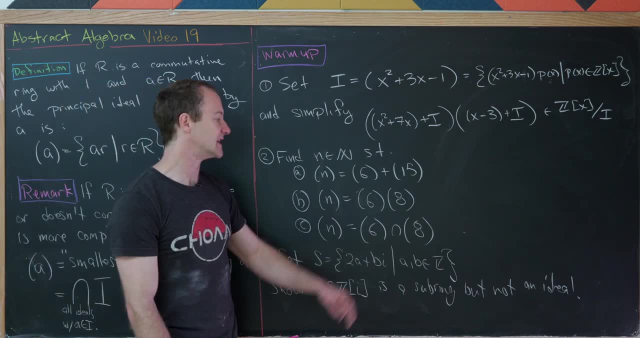 Generated by six and eight. And then finally. 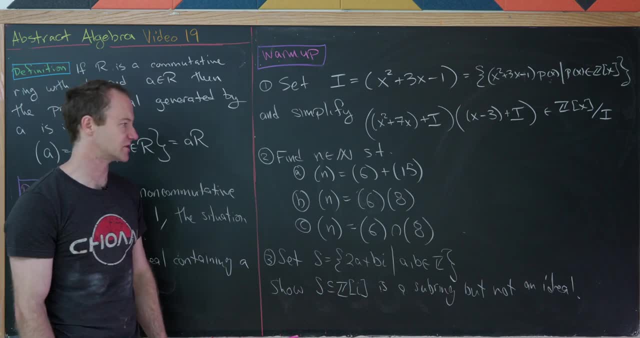 N is the intersection of the ideals. Generated by six and eight. So I think those are all pretty interesting. 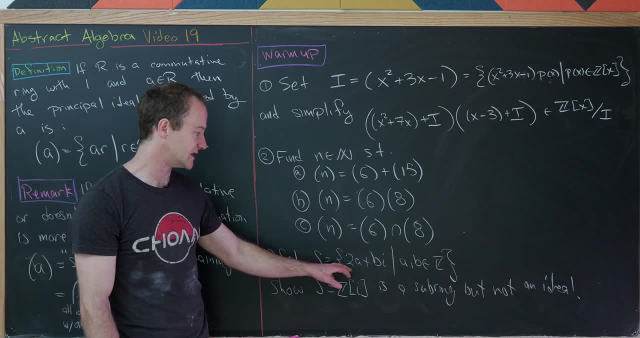 And then finally. Let's set S equal to all Gaussian integers. Where the real part is even. So in other words. We've got everything of the form. 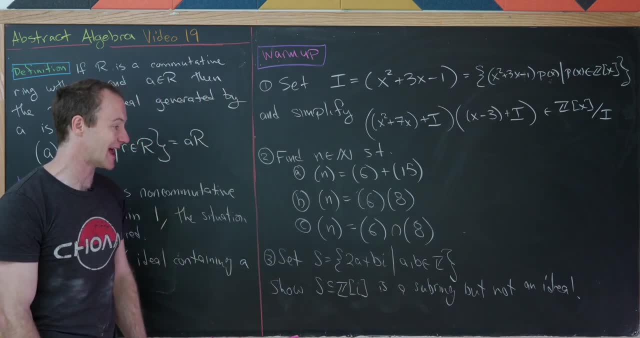 Two A plus B I. Where A and B are integers. 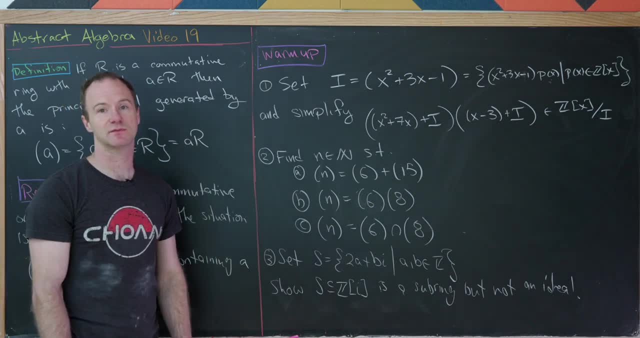 Then next let's show that S is a sub ring. But not an ideal. 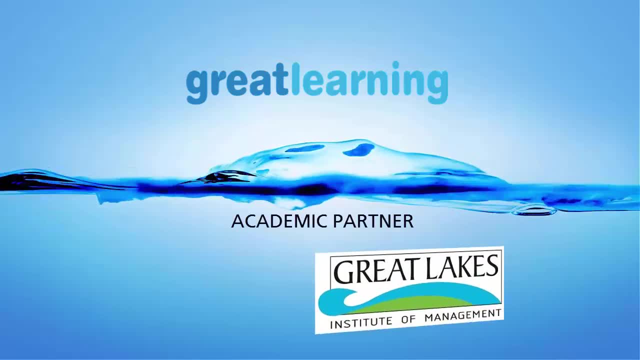 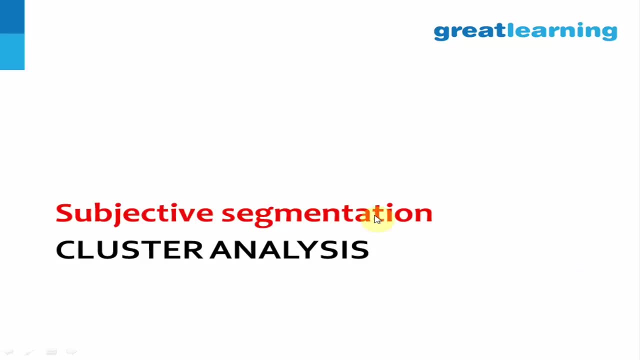 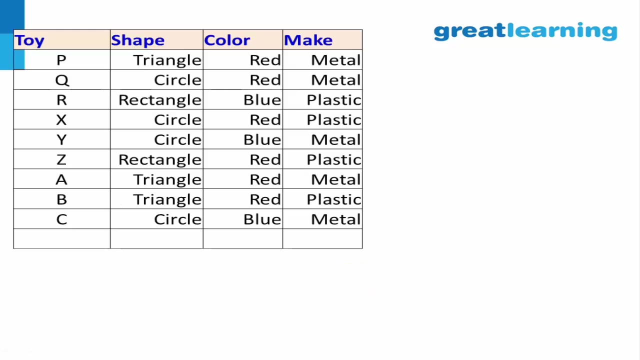 Let me briefly explain you: subjective segmentation or cluster analysis. In case of cluster analysis, your task is to figure out which are the objects which are similar. This is the case where you have been given some toy. their shape, their color, their make, Shape is like triangle. 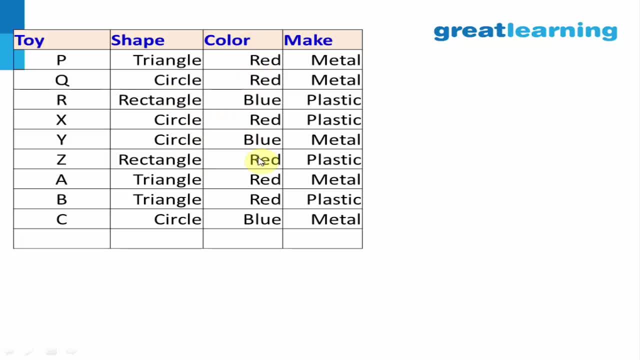 circle, all those things Color you have red, blue, all those things and make. you have. these are made of metal or plastic And the task that has been given to you that find objects, observations which are similar. You can call these are observations or these are objects. 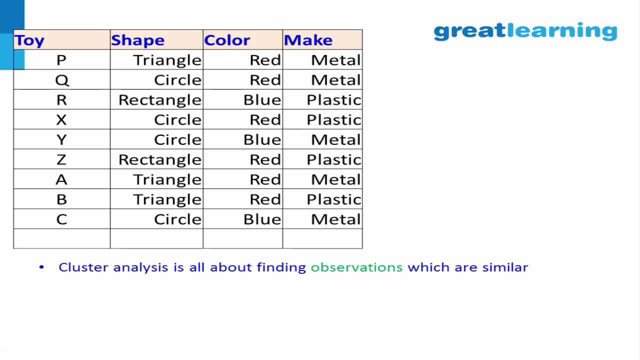 So in cluster analysis, your task is to find observations which are similar. Now, what is the whole idea? The idea is that when you group them together, they should be homogeneous within group. What does it mean? that each object in the group should be similar to each.